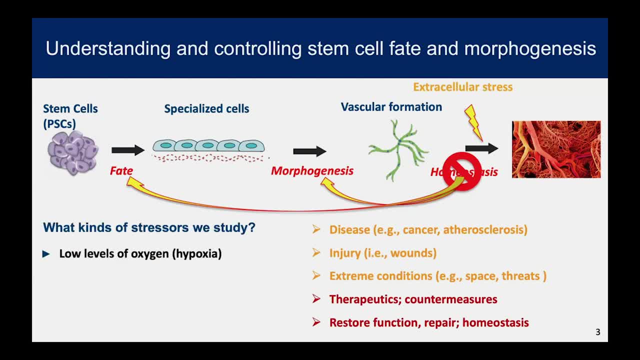 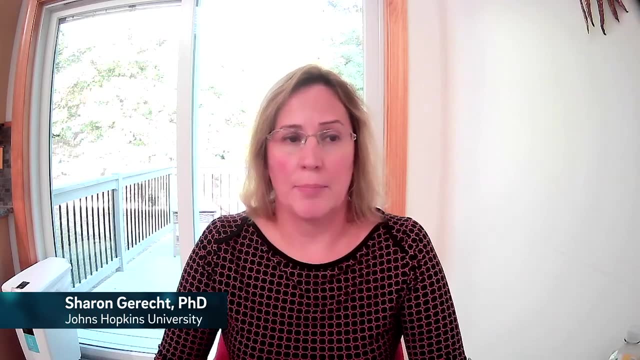 Which stressors we study. We study low levels of oxygen, hypoxia. We study changes in the surrounding extra cellular matrix in flow and strain and radiation. Today I'd like to focus on a couple examples surrounding our work with hypoxia and with the extracellular matrix. 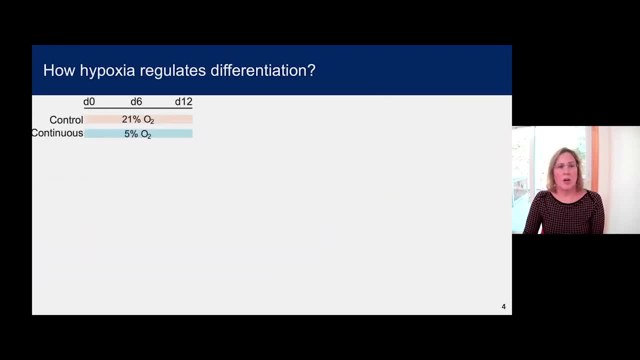 The first study done several years ago, we looked into how the differentiation or cellular or endothelial fate is impacted by hypoxia Through the differentiation of our induced pluripotent stem cells, through the differentiation of our induced pluripotent stem cells. 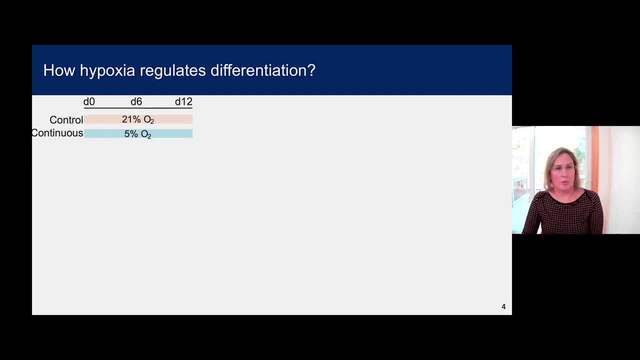 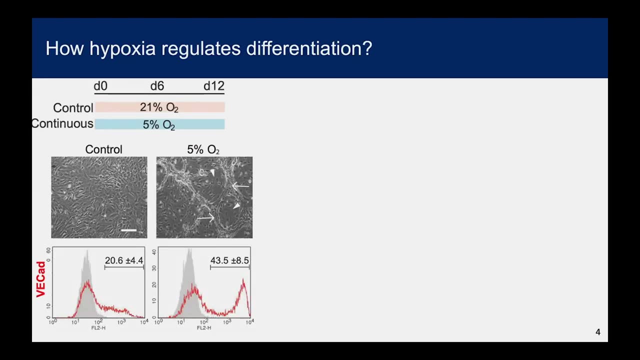 we found that the co-efficient of hypoxia is seen as this one. this thing, This is a proliferation of the cell and this cell is deviating from the cell based cell to the cell based cell. When you look at the cell, 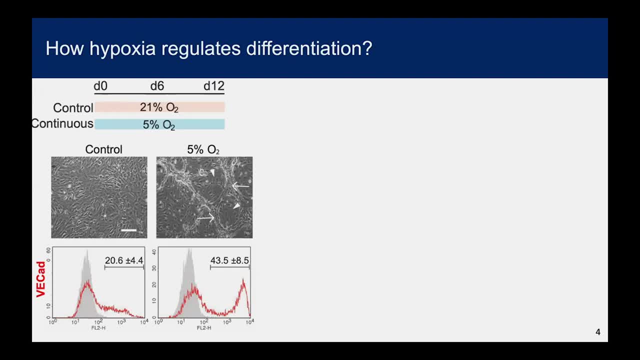 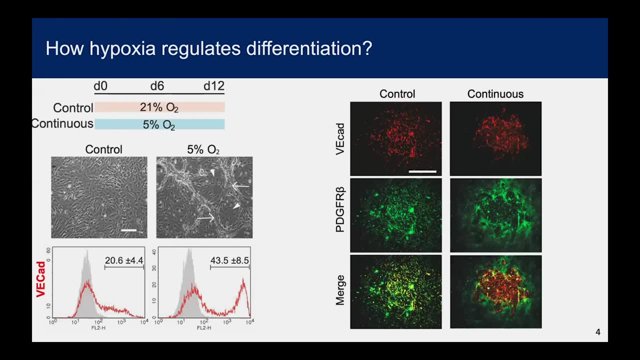 we can see the endothelial condition and we can see the function of this cell. And since it's this one, we can clearly see the function of the cell. We can see the function of the cell. The cell is still having small changes. 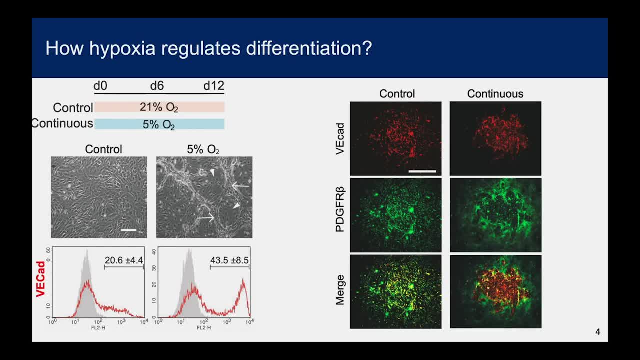 It's becoming more and more. I mean the EGC has to be done: V-cadhering positive cells that are surrounded by PDGF receptor beta positive cells, which are parasites. With that, we wanted to understand: is it the early stages of differentiation that 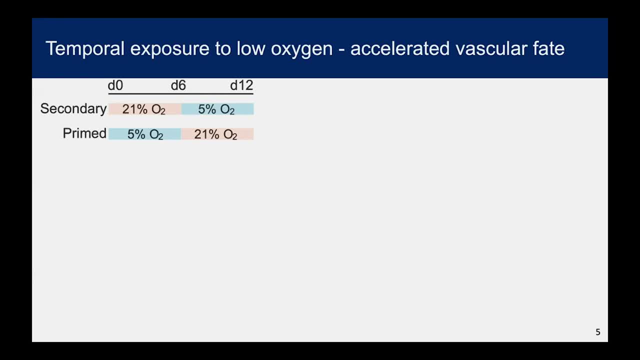 impacting the differentiation in hypoxia, that impacting the fate, or later on, So around the middle of the differentiation, around day six. this is about a mesodermal induction. So we expose the cells to what we call secondary hypoxic or prime hypoxies. as well, the control and continuous 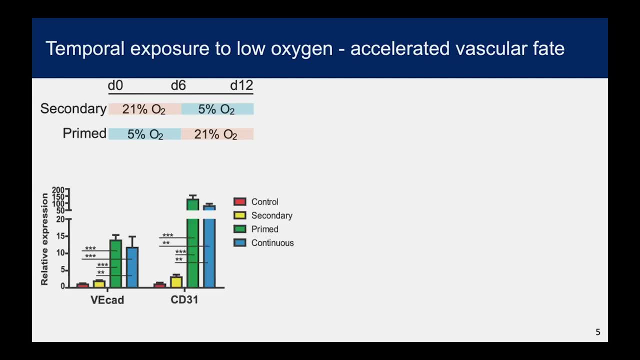 hypoxia And what we have found is that when we expose the cells to either atmospheric condition or later stages of differentiation to hypoxia, we see no upregulation of specific endothelial marker: V-cadhering and CD31. But we saw upregulation of these markers when we expose the 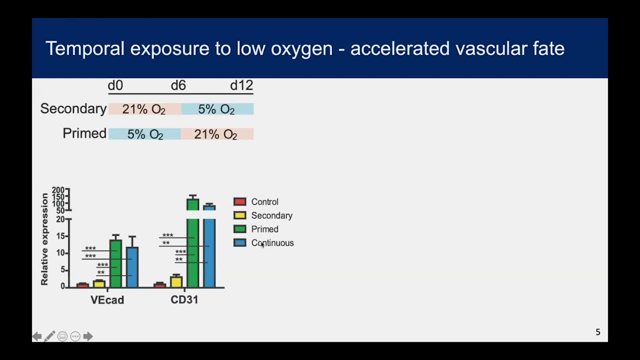 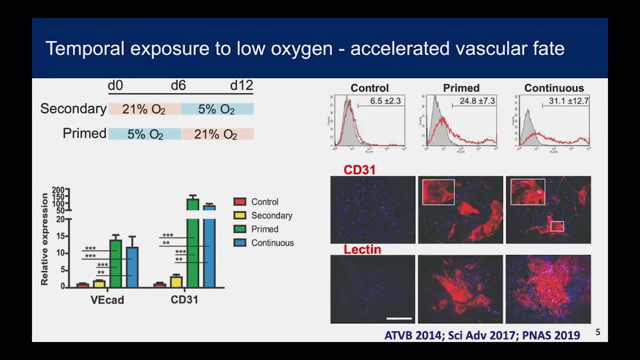 cells during early stages of differentiation to either atmospheric condition or later stages of differentiation to hypoxia. We have done several other analyses where we show again upregulation of V-cadhering, CD31, and lectin as well as the functionality of these cells. 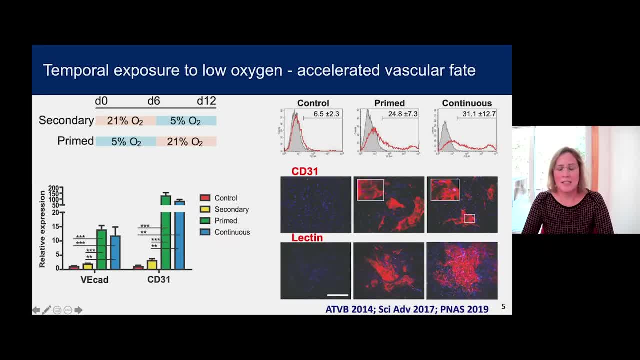 This study was published in 2014, but since then, what we noticed in other published that I'm just not going to go over right now is that other stresses, such as different stiffnesses of the matrix and other stresses such as stiffness of the matrix and other stresses such as stiffness- 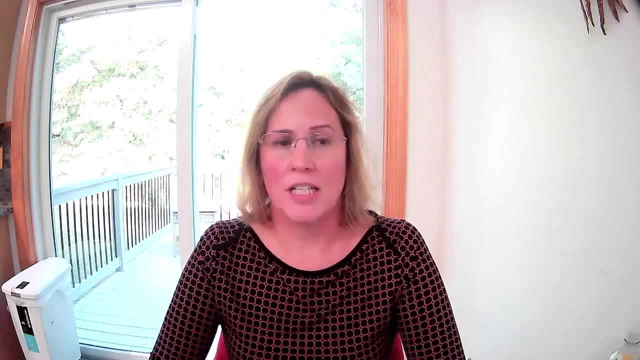 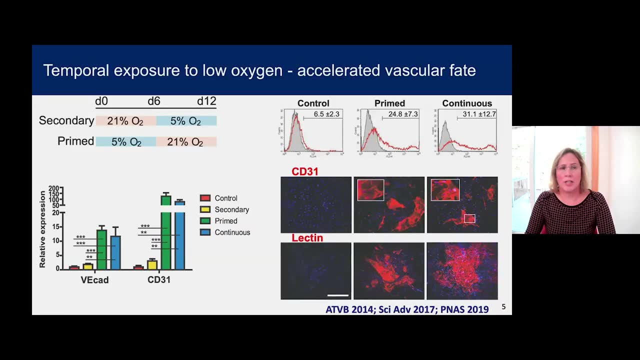 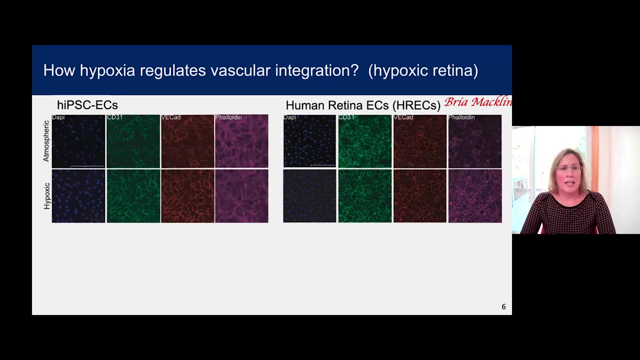 of the matrix and also patterning of the extracellular matrix will impact this vascular fate. So, with that in mind that we know that hypoxia regulate the fate towards, or impacting the fate towards, a more endothelial cell, we wanted to ask how the hypoxia regulate vascular 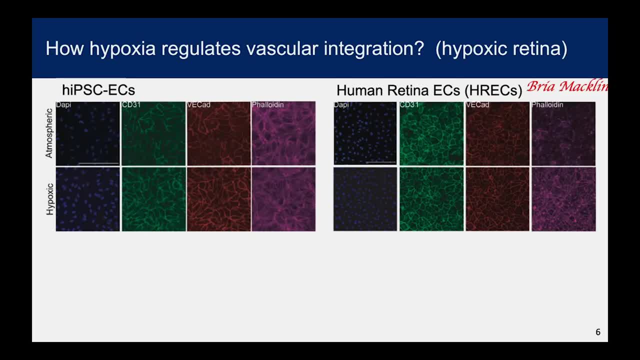 integration. Specifically, Bria Macklin, who was a PhD student in the lab back then, wanted to examine the hypoxic retina tissue. I'll explain a little bit later why we chose this specific hypoxic retina. So the first thing she did, she just compared the IPS-derived endothelial cells and mature human 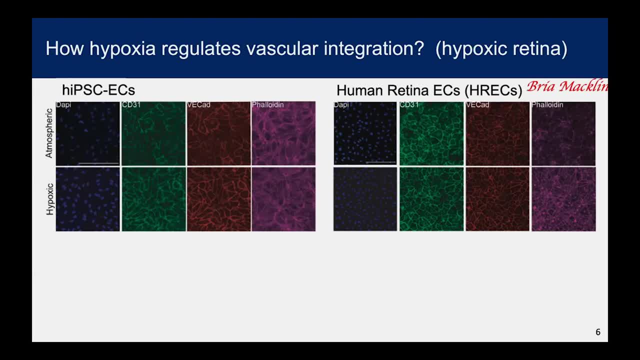 retina endothelial cells when she exposed them to hypoxic conditions and we have in vitro and we saw no difference. She did notice that there is some difference in the proliferation rate of these cells in vitro, where we saw that the hypoxia did not impact the 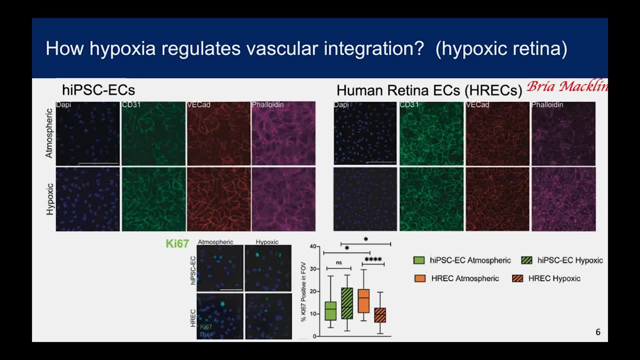 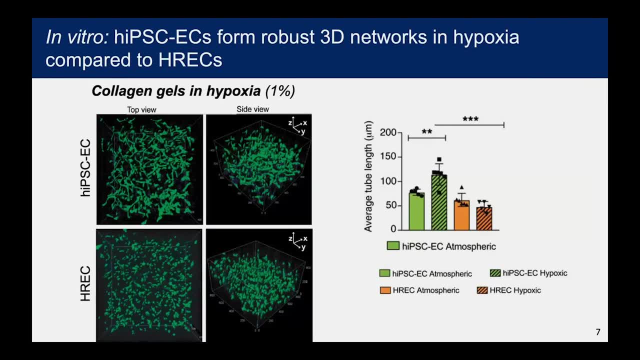 IPS-derived endothelial cells proliferation rate, but it did slow down the proliferation of the mature cells. She then moved to three-dimensional assay where she took collagen gels and formed a network inside these collagen gels. in hypoxia, and comparing again the IPS derivative to the 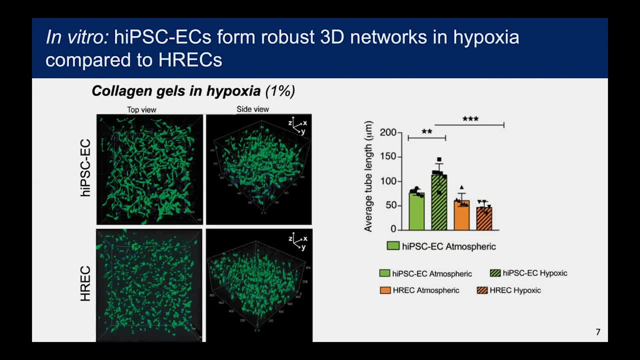 mature retina endothelial cells. and she found that the hypoxic condition in the IPS case induced better and more proliferation of the mature retina endothelial cells. and she found that the hypoxia did not impact the mature retina endothelial cells. and she found that the hypoxic condition in the 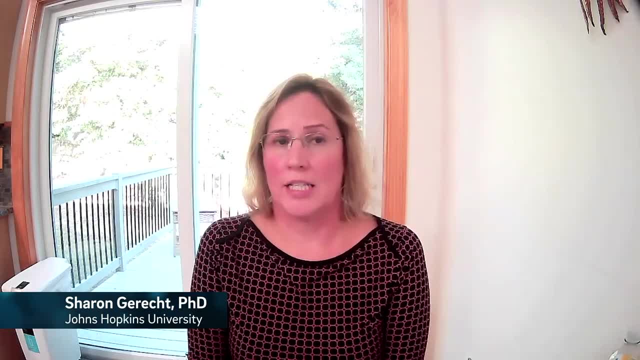 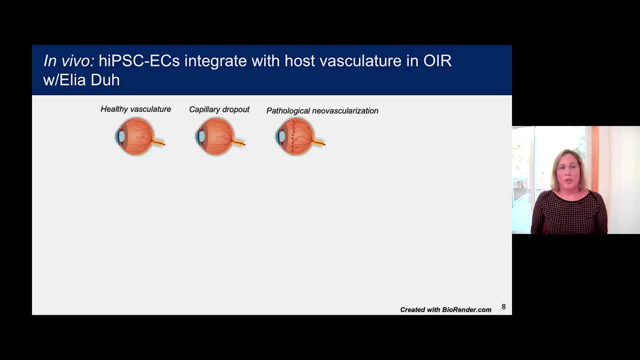 with that, we wanted to go in vivo and ask how we can study more about the integration of IPS cells in hypoxic conditions. For that we collaborated with Elia Dow, who is at the Wilmer Institute at Hopkins, using this oxygen-induced retinopathy model, which is a 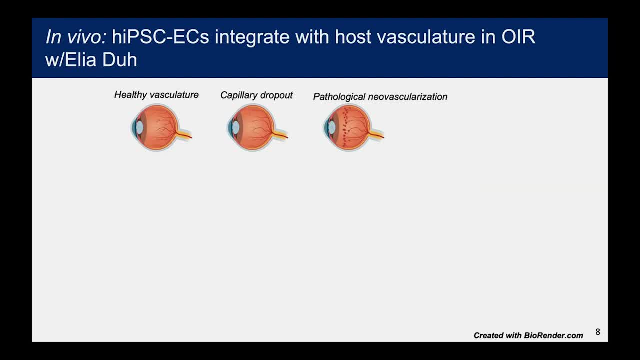 clinical trial of the hypoxic condition in the hypoxic condition in the hypoxic condition in the classic, to examine how our cells respond to hypoxia During retinopathy. what's happening is that the healthy vasculature are exposed to stress, in this case glucose, causing the 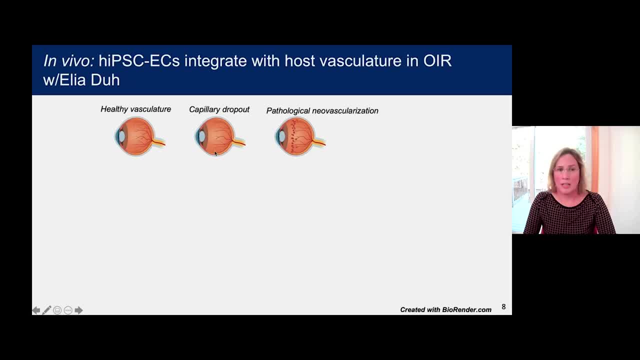 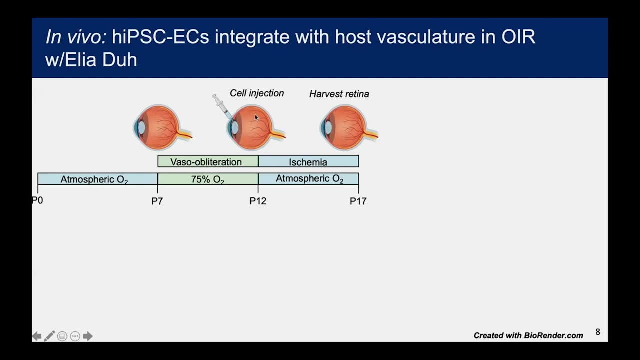 capillary to drop out this, causing hypoxic or ischemic region in the retina which is induced pathological neovascularization. What we thought we could do is basically inject the cells in that point where we are generating this ischemic condition, hypoxic conditions, and see if they 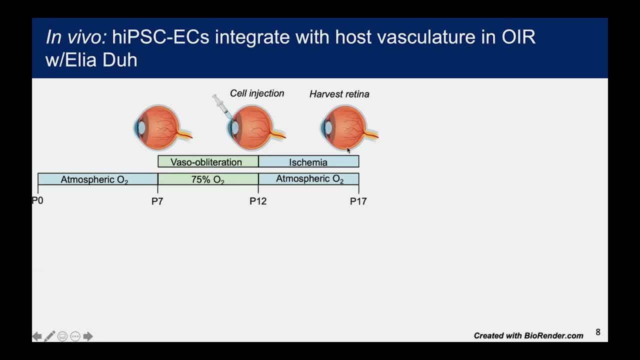 are going to stabilize the retina vasculature. The way this essay goes, we take the PAPs on day seven, we expose them to or we take them into high oxygen chambers and then move them back to atmospheric condition, which is induced ischemia. What we have found is that when we inject the 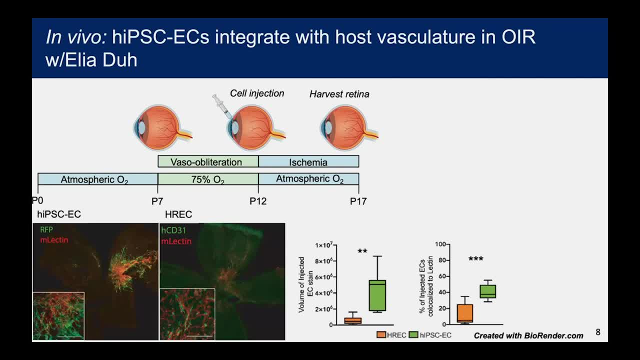 IPS-derived endothelial cells into this hypoxic retina. they integrate very nicely with the host vasculature. You can see here in green are the injected cells, either the IPS-derived or the mature cells, and M-lectin is the mouse lectin. They integrate much nicer with the mouse vasculature. You can. 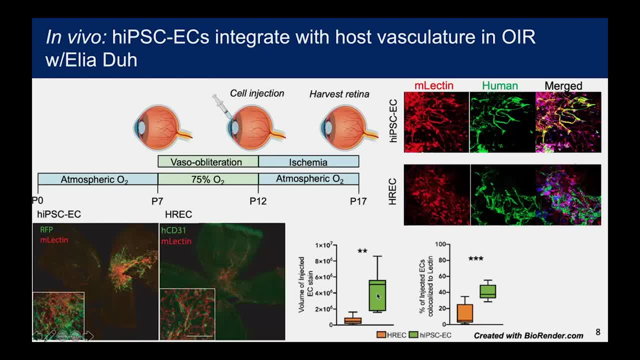 see this clearly in these images where we see nice integration in yellow of the mouse and the human vasculature versus the mouse. We can see that the mouse vasculature is very nicely integrated into the hypoxic retina versus the mature retina endothelial cells that are basically generating. 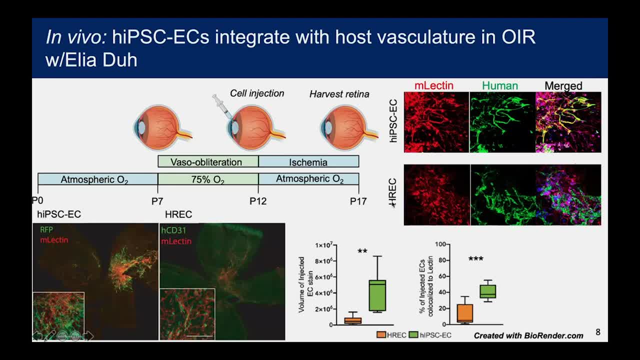 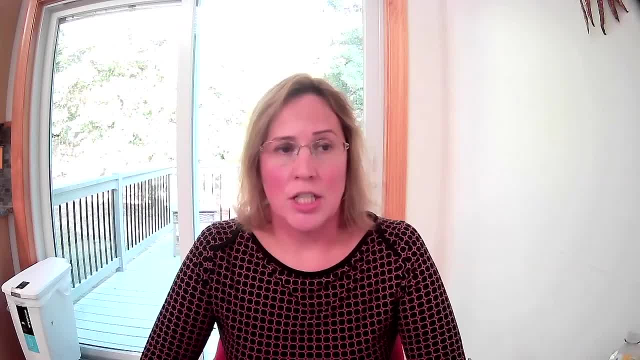 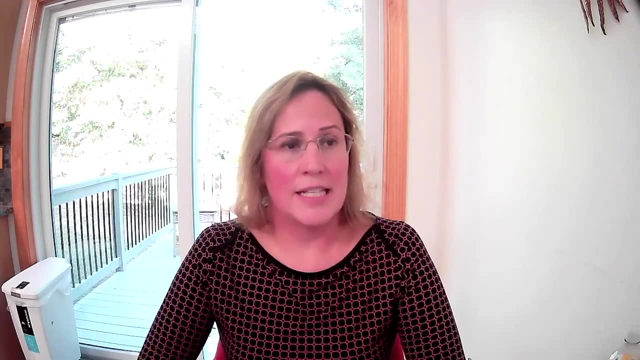 a layer of vascular network on top of the mouse vasculature. Bria continued to ask why this is happening. She came up with this nice essay where she encapsulated in the collagen gel SDF1-alpha, which will recruit endothelial cells and basically sit at the endothelial cells on top. of this hydrogel. Again, put them in hypoxic retina. We can see that the mouse vasculature is very nicely integrated into the hypoxic retina. We can see that the mouse vasculature is very nicely integrated into the hypoxic retina. We can see that the mouse vasculature is very nicely integrated. 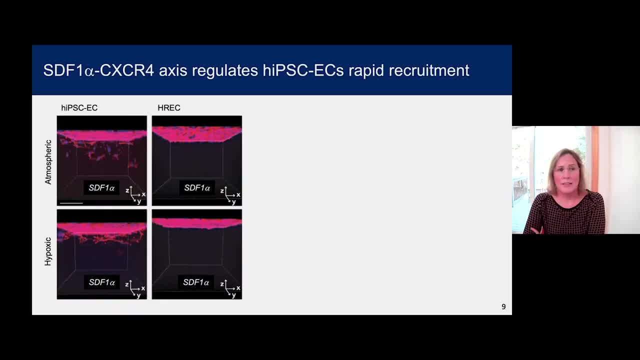 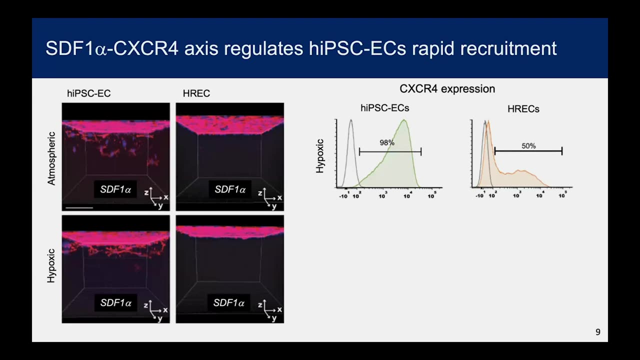 or atmospheric condition. As you can see here, we found that the IPS-derivative penetrated better to this collagen, either in atmospheric or hypoxic conditions. Indeed, she found in the hypoxic conditions that our IPS-derivatives express the receptor for the SDF1-alpha, the CXCR4.. 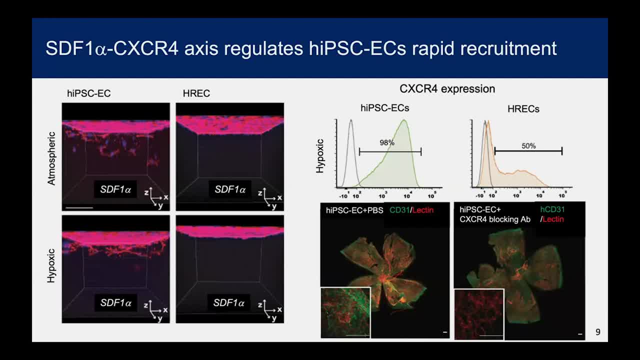 Indeed, when we inhibited the CXCR4 using blocking antibody in the case of the mouse vasculature, we found that the mouse vasculature was better in vivo. When we injected that along with the cells, we see a much less integration of the. 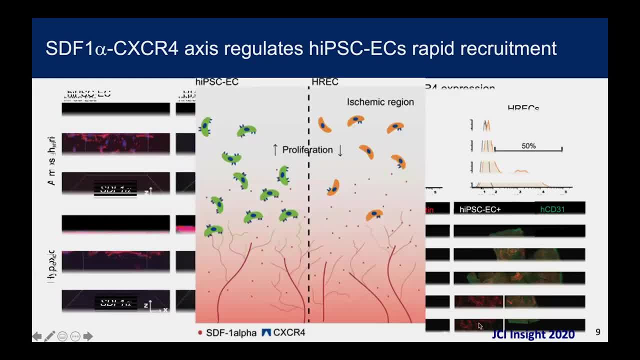 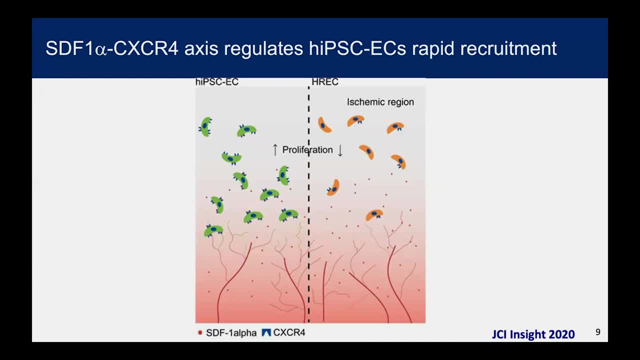 human vasculature with the host vasculature. So all in all, what we're thinking is happening in the IPS-derivative. compared to the human retina endothelial cells, the IPS-derivative proliferate faster, They're recruited to the host vasculature and integrate much more efficiently. 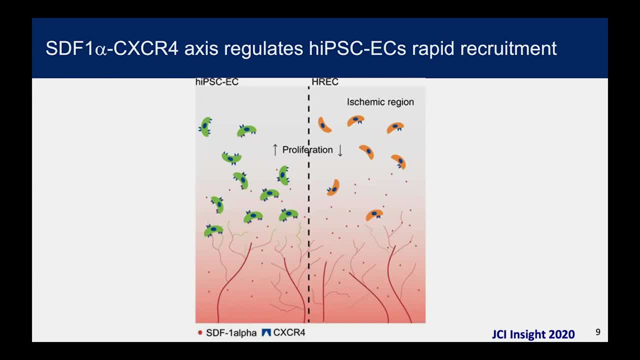 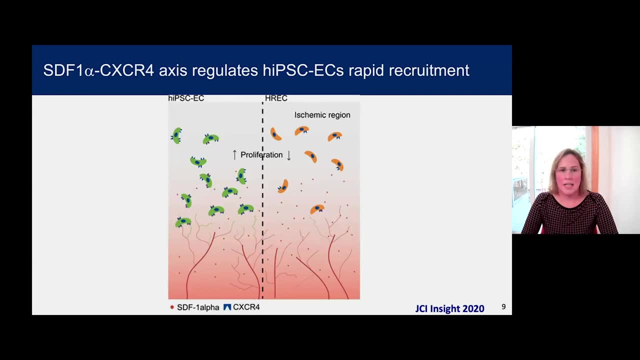 than the mature endothelial cells. So we can see that the mouse vasculature is much more efficient than the mature cells. So we continue in this study to understand better also how or what is the role of the parasites in this cascade which are known to contribute to the retinopathy. 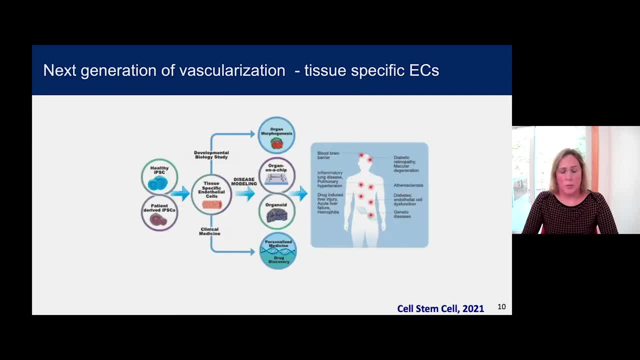 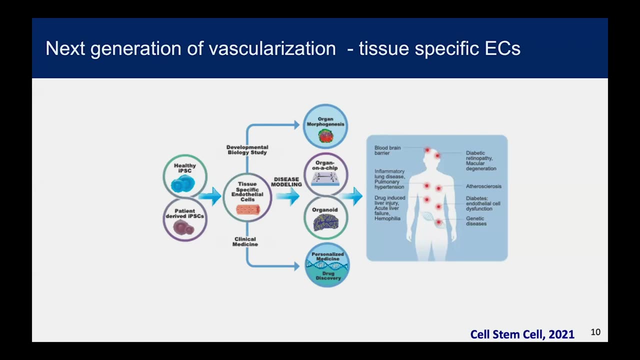 pathology, But in general, where we are thinking these studies or this area is going to, and I think Gordana gave a good overview of what we can do with these cells. So what we're thinking is that in large scales and also in organoids on the chip, is we're thinking 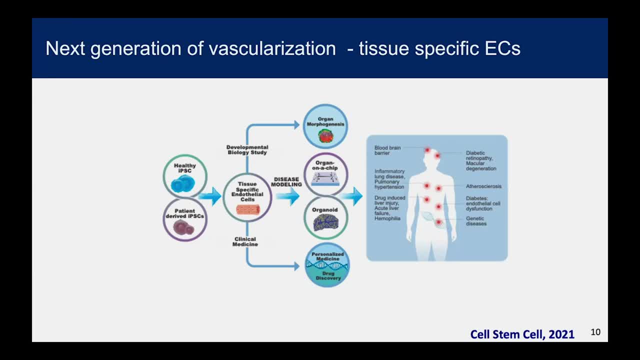 it's going towards tissue-specific endothelial cells, where we'll be able to analyze how the endothelial cells impacting specific tissue or in the tissue environment that they're in, and, vice versa, how the tissue environment regulate the functioning of these tissue-specific endothelial cells, And this will allow us to understand more about organ morphogenesis. 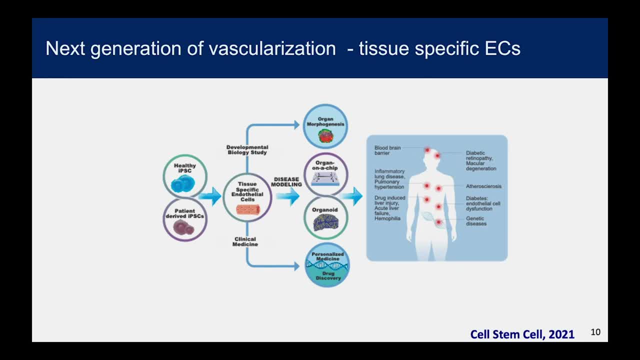 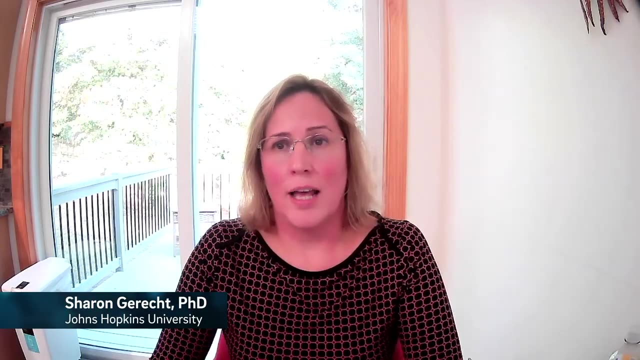 develop more precise organ and chip models as well as organoids, and hopefully develop a personalized medicine and drug discovery in specific organs in the body. So with that we wanted to understand how hypoxia regulate vascular assembly, and vascular assembly is happening in three-dimensional. 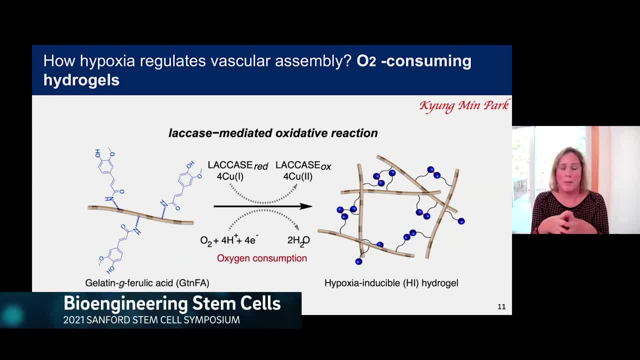 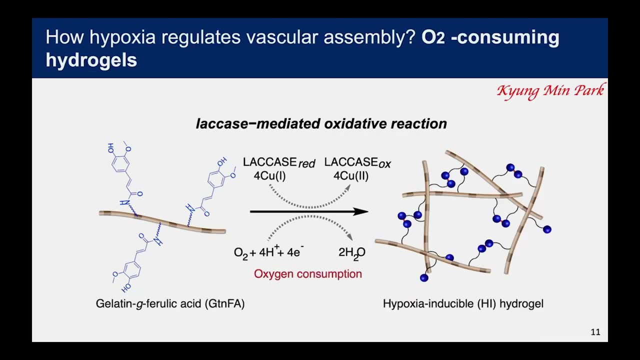 And towards that. instead of taking those collagen gels like what Agriya did before and just put them in this hypoxic chamber and then take them out and analyze them, what we? Keong Ming Park in the lab, who was a postdoc in the lab, developed this nice hydrogel system that basically has a backbone. 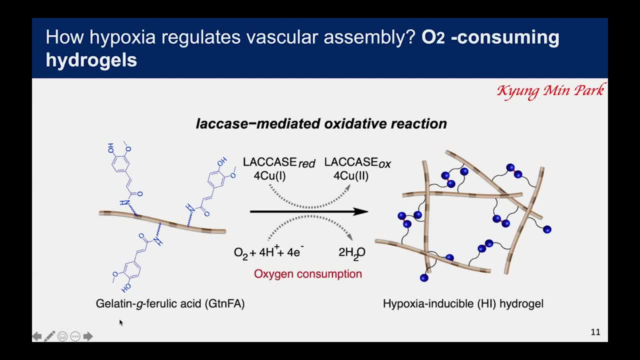 it could be a gelatin or polysaccharide such as dextran, and it's modulated with ferulic acid that, in the presence of leches, creating this reaction that consume oxygen. What's happening is then that we have hydrogels that are in this hypoxic chamber, and then we take them out and 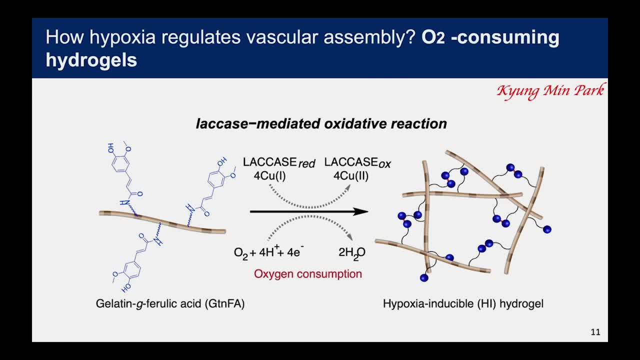 analyze them. what we Keong Ming Park in the lab? what was a postdoc in the lab develop this nice that while it's forming in the lab it's becoming hypoxic. So we have hypoxic environment basically on the bench. When we add cells in those hydrogels, the cells continue to consume. 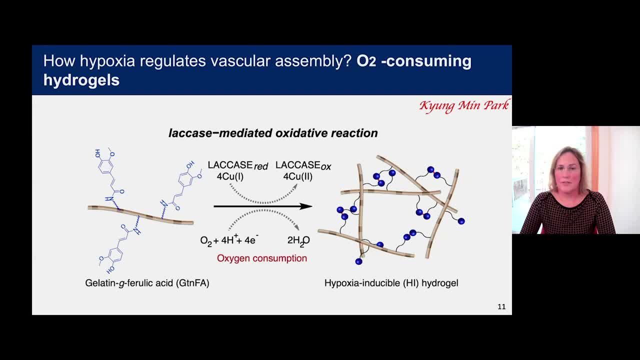 oxygen and those maintaining this hypoxic levels for longer periods of time. We found that it's with the endothelial cells, or endothelial progenitor cells. they're continuing these hypoxic conditions up to a three-dimensional state, And then we take them out, and then we 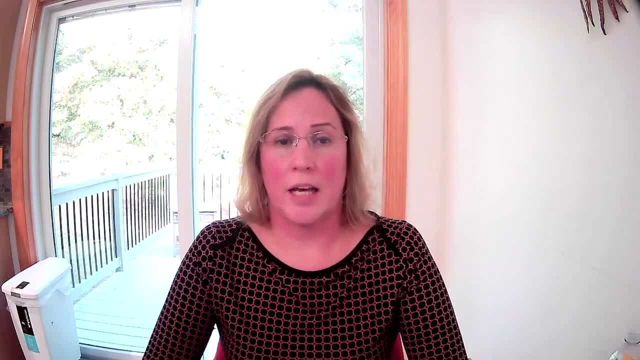 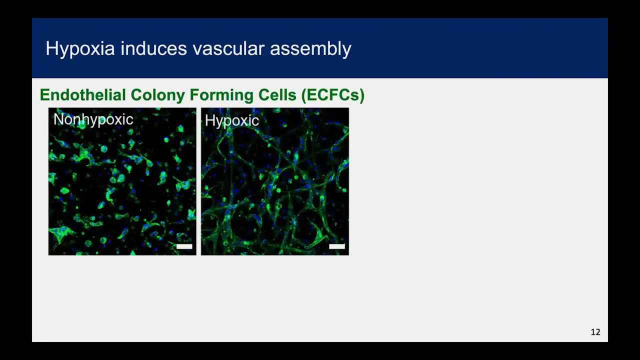 calculate the hypoxic rate of the fact that the cell is forming in the hypoxic condition. So in the endothelial cell it's about a 40th hours which is enough to activate a hypoxia-inducible factors one and two, which takes about a four to six hours to accumulate. So with this I'm not. 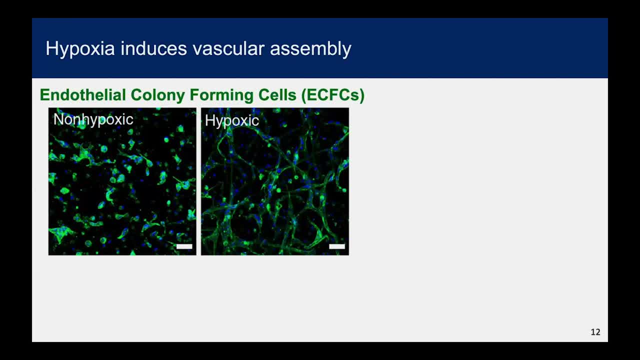 going to get into too many details, but we encapsulated here endothelial colony forming cells And as you can see here in the hypoxic condition there was, they promoted very nice vascular networks compared to the non-hypoxic, which kind of allowed us not to be able to do跳atopraza. we spavatoloma, uterine lyme cells and the other things there. So that's very interesting and I'm going to look at that. And then we can also look at the transcriptional structure which is going down in 3, Professor Seckler's. 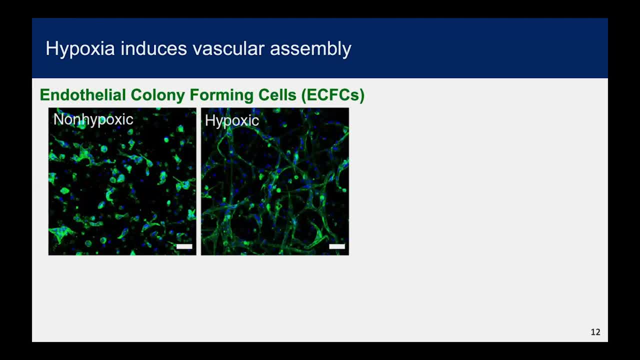 the cells to sprout but not really form robust network. Through a series of studies we found that the hypoxia, of course, stabilizing hypoxic inducible factor- in our case both one and two- and they upregulate the MMPs that allow. 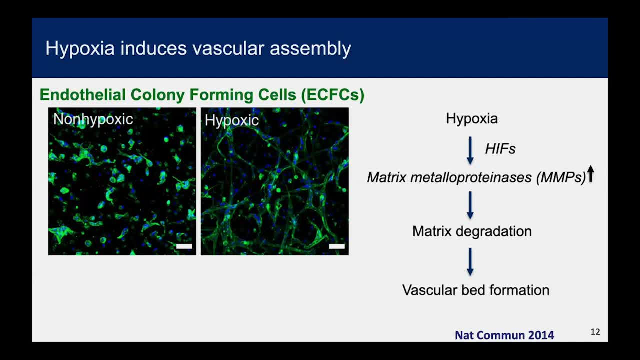 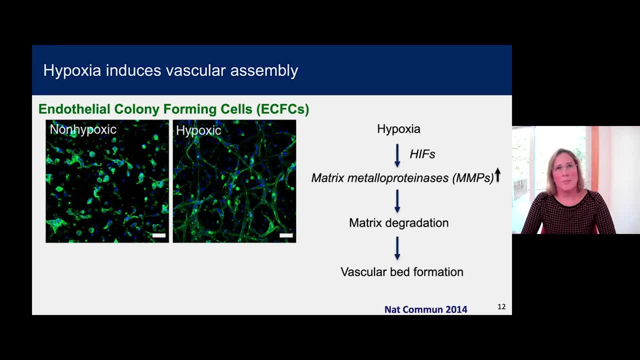 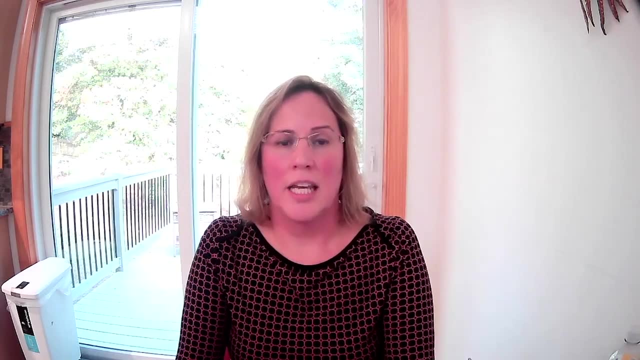 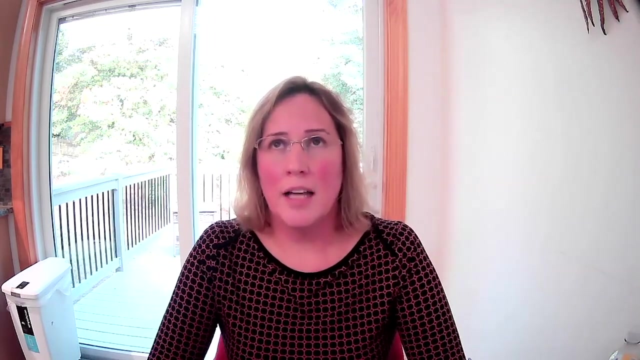 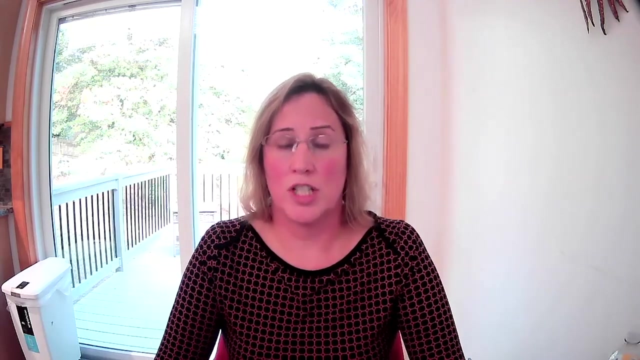 the matrix to degrade and then to be a vascular bed to form. So with that in mind, this was basically our first study that demonstrated that there is a direct loop between a hypoxic condition impacting the matrix through their degradation. So with that, we thought about how the matrix mechanics regulate this vascular morphogenesis. 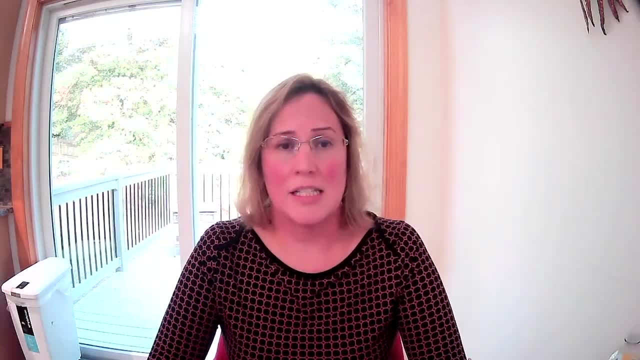 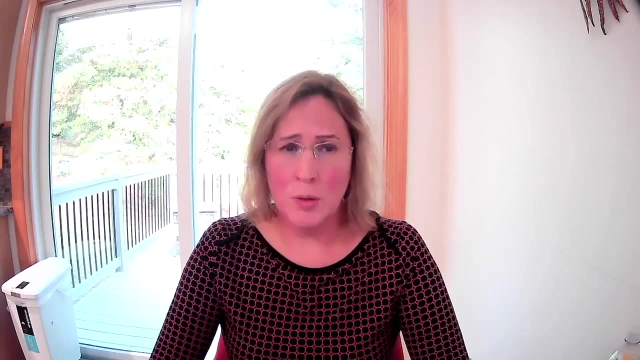 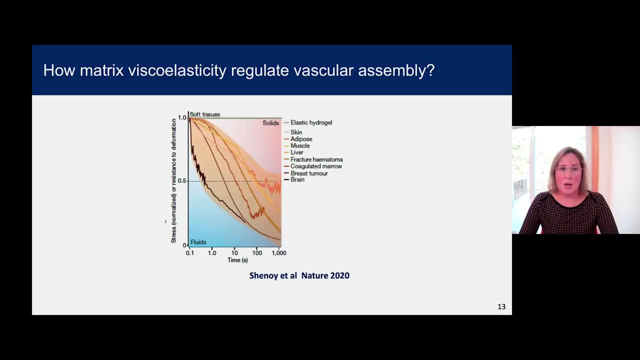 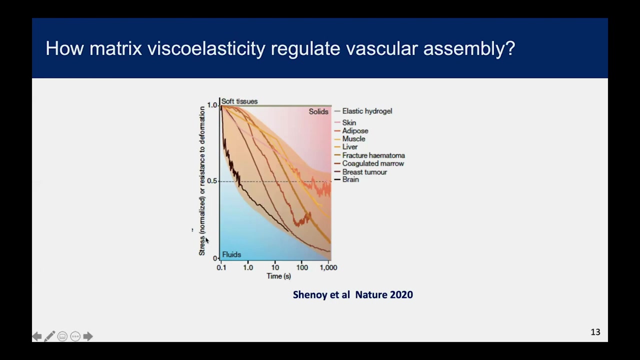 And there have been other studies that show the impact of stiffness on network formation. But we were actually interested in how vascoelasticity regulate vascular assembly. So most of our tissues in our body basically have both elastic and viscous properties. This is a nice review published last year. who is demonstrating the vascoelasticity properties? 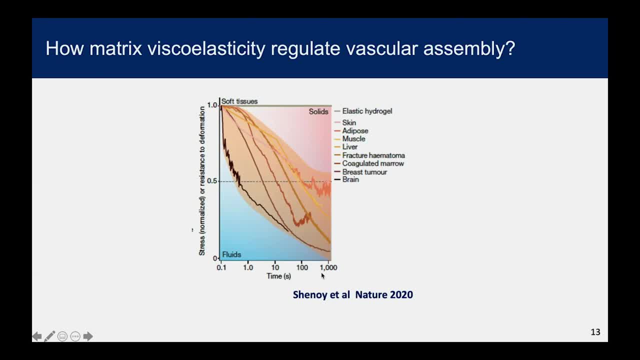 of the matrix, their ability to respond to deformation by relaxing. So, with that in mind, we wanted to understand: is vascoelasticity regulate this morphogenesis of the vasculature? So Zhai Wei and Rahel Sheleman in the lab developed this nice hydrogel system which 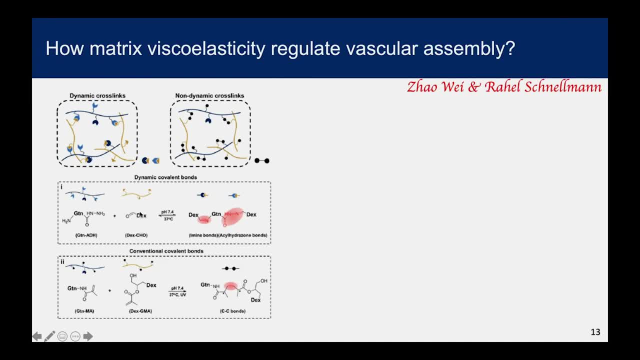 composed from a dextran, so from polysaccharide and from gelatine, and we generated two types of hydrogel system: One, what we call dynamic cross-linking, So what we call dynamic cross-linking. So what we call dynamic cross-linking. 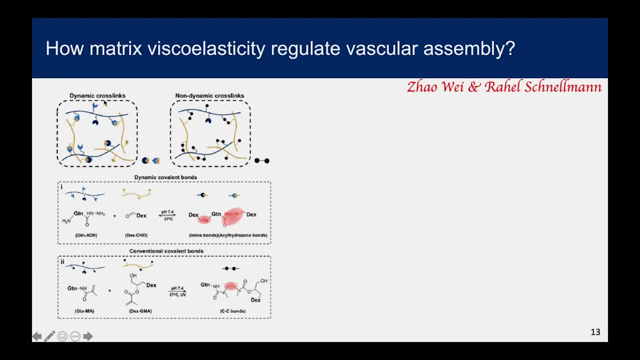 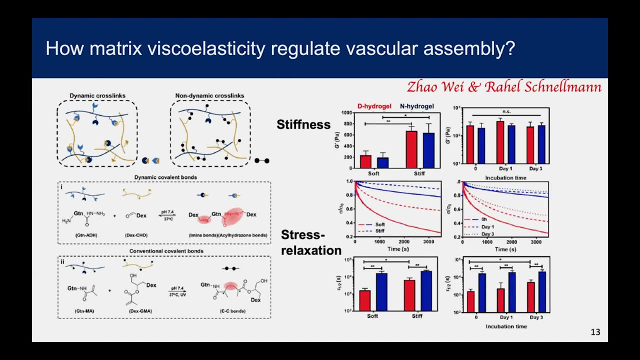 So we call dynamic cross-linking, Which allow us to mimic vascoelastic properties, and one that is non-dynamic cross-linking. We made sure that we can decouple stiffness and stress relaxations in this hydrogel, so then we can make the hydrogel soft or stiff and maintain that soft and stiffness throughout. 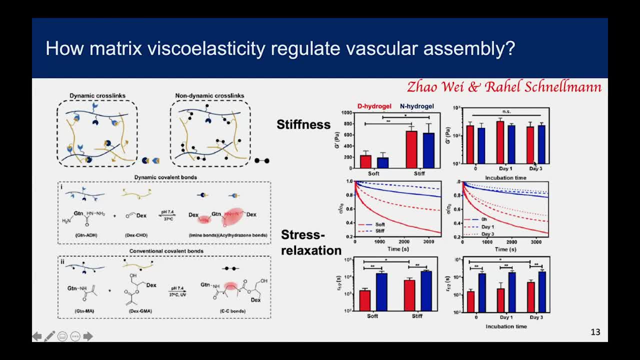 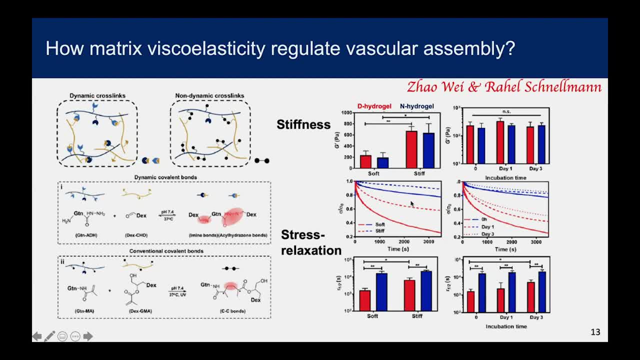 We are really happy to have you here. We will be joined soon. Thank you, Have a good day. differ in their stress relaxation, And this difference in stress relaxation can be maintained over three days of culture break. So with that, we wanted to understand how they modulate. 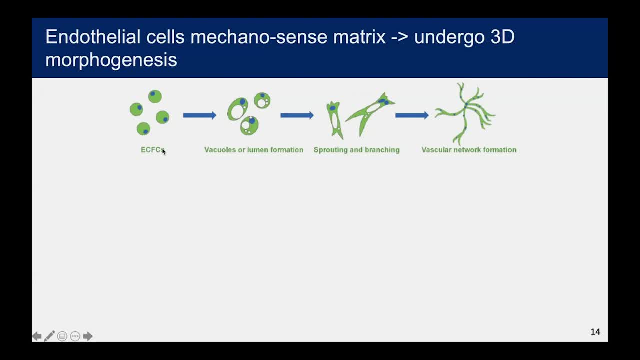 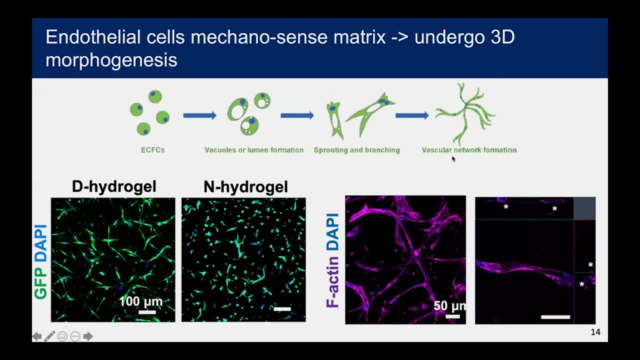 morphogenesis So quickly. endothelial cells morph into vascular networks through a process that starts with vacuole or a small lumen formation, Then the cells then sprout and branch and form the network. And indeed, when we encapsulated these cells in what we call the dynamic hydrogel, 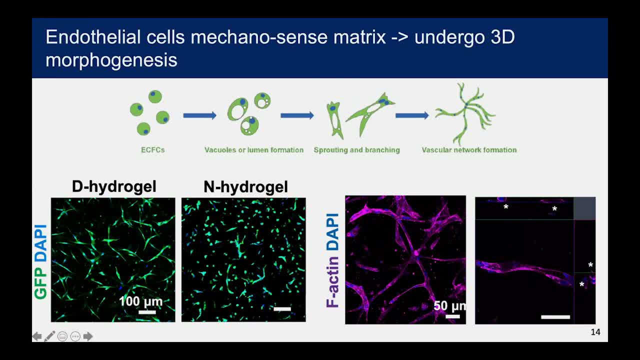 the vascular elastic hydrogel. they form these beautiful networks versus the non-dynamic hydrogel. We see that they are forming some network, but not as robust and complex as in the dynamic hydrogels And you can see here a luminal structure forming in the dynamic. 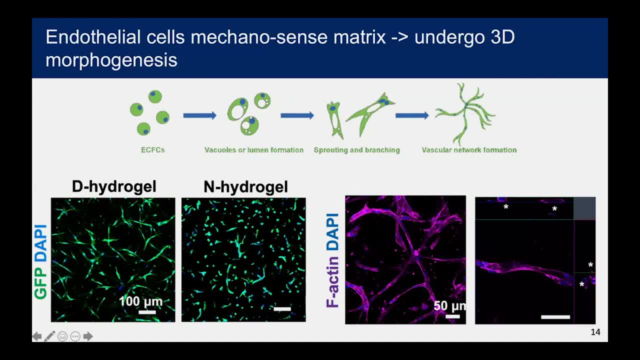 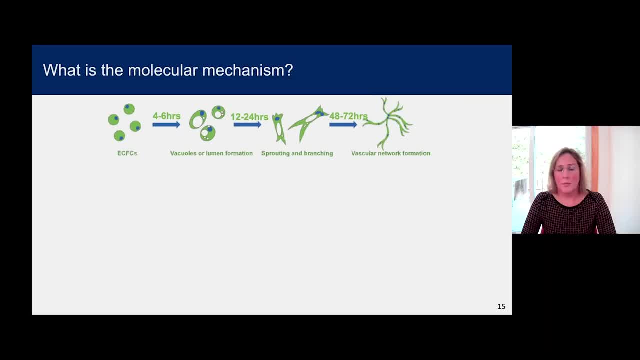 hydrogels, which we cannot find in the non-dynamic hydrogel. We then wanted to understand how they morph into morphogenesis. So we wanted to understand more. what is the mechanism that regulate this process? And we first examined if the vacuole and 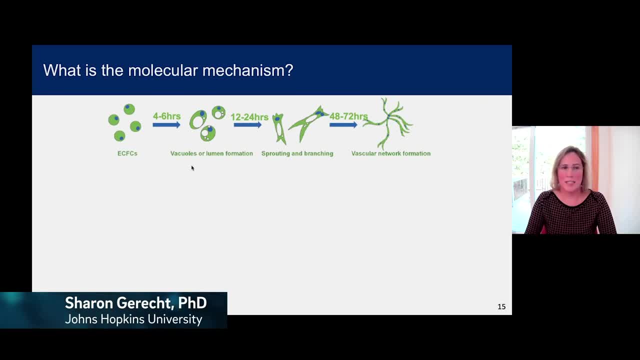 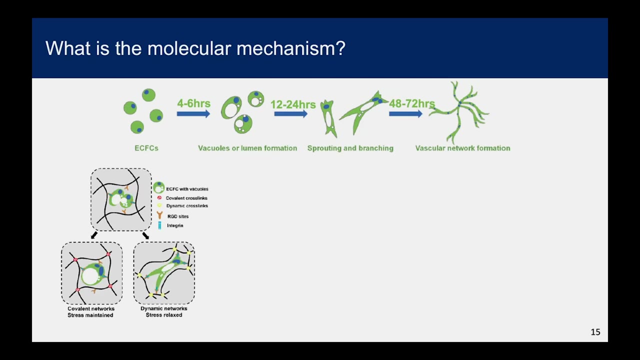 lumen formation process, which takes in culture about four to six hours, is modulated between the two hydrogels, and we did not find any difference. Both of them allow the cells to undergo vacuole and small lumen formation. Then we hypothesized that what's happening in our hydrogels is that 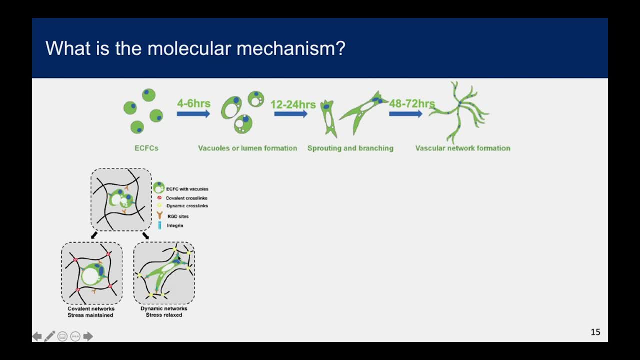 the dynamic hydrogels allow the cells to contract and push and allowing them to sprout, And this does not happen in the non-dynamic hydrogels because they are not flexible. And indeed, by encapsulating fluorescence beads and following them with time-lapse, we could see that the 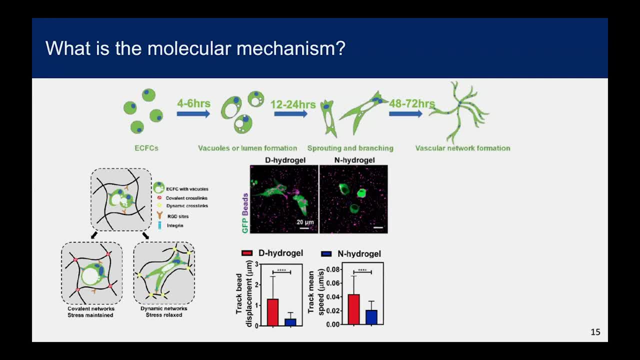 fluorescence beads move, while we have cells in the hydrogels move further and faster in the dynamic hydrogel compared to the non-dynamic hydrogels, And we also found that the dynamic hydrogels are more flexible in the non-dynamic hydrogels And indeed, when we stand for a contractile marker. 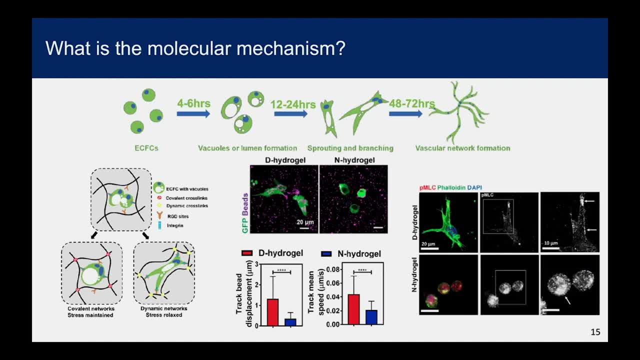 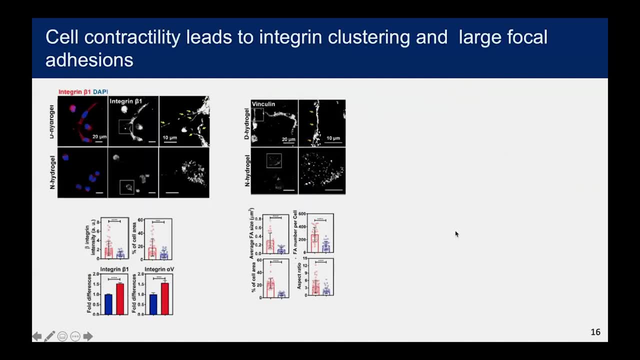 the phosphorylated MLC, a myosin light chain, we could see that the cells in the dynamic hydrogel are contractile. We also noticed that this contractility is leading to integrin clustering and you can see that with the basically clustering of integrin beta-1 in the dynamic and not in the non-dynamic, And we also found that the cells in the dynamic hydrogel are more flexible in the non-dynamic hydrogel. We also found that the cells in the dynamic hydrogel are more flexible in the non-dynamic hydrogel. We also found that the cells in the dynamic hydrogel are more flexible in the 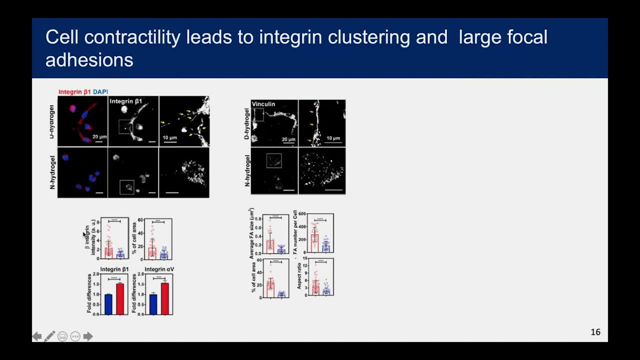 Also done some UPCR and showed the differences in integrin beta-1 and integrin alpha-V in the dynamic versus the non-dynamic. This lead to large focal adhesion formation, here marked by vinacoline, again that we could see the difference between the dynamic and non-dynamic. 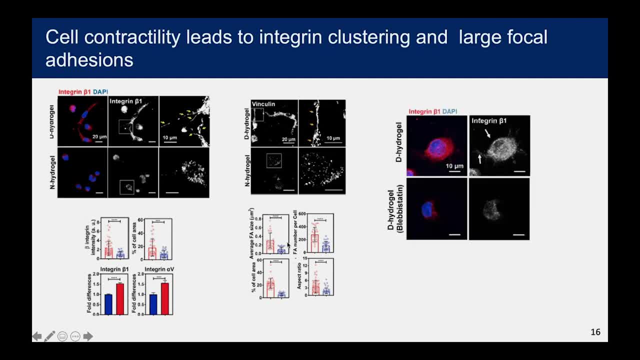 And when we inhibit the contractility of these cells with blabestatin we could see a motherfucker's of course, a downregulation of the intergrin clustering, And this leads also to inhibition of network. when we inhibit cell contractility compared to controls. 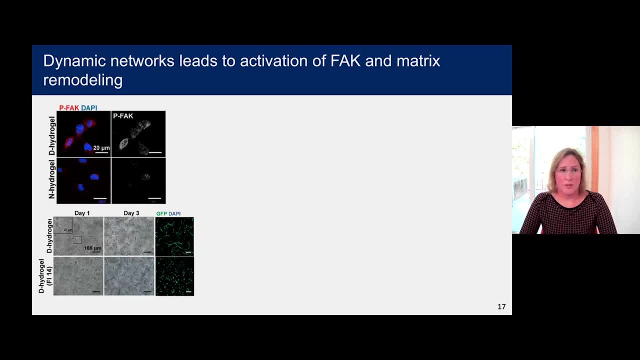 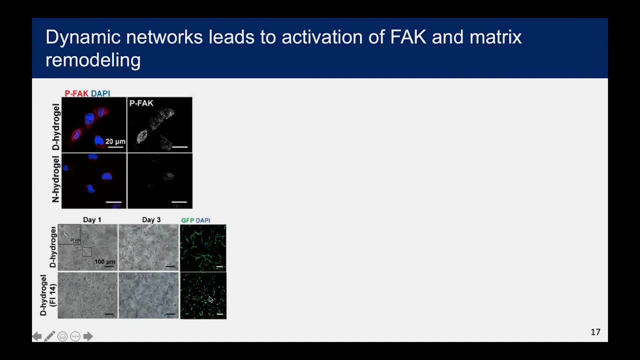 We then looked into deactivation and phosphorylation of focal adhesion kinases And again we could see upregulation in the dynamic hydrogel and the non-dynamic hydrogel. When we inhibit phosphorylation of focal adhesion kinases, we could see inhibition of the network. 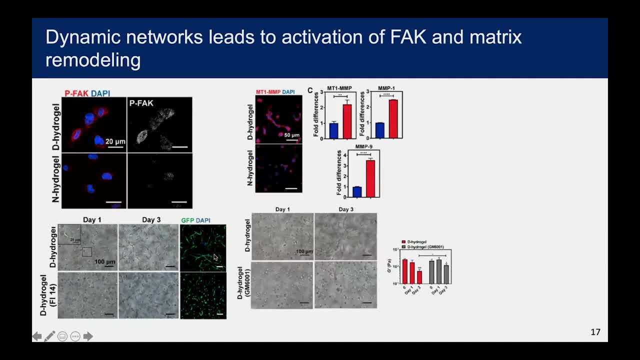 compared to the control. Our cells, not just sitting there and starting to make networks, they are actually interact with the matrix. They start to degrade the matrix and they degraded faster and better with the dynamic hydrogel And we see that with expression of the membrane. 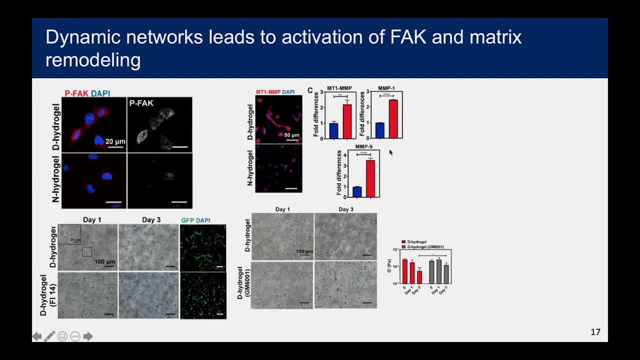 Mp1 and Mp9. And again, when we inhibit with the general inhibitor of MMPs, we could see inhibition of network formation. Nicely, we could also see that when we inhibit the MMP we could see that the degradation of the matrix 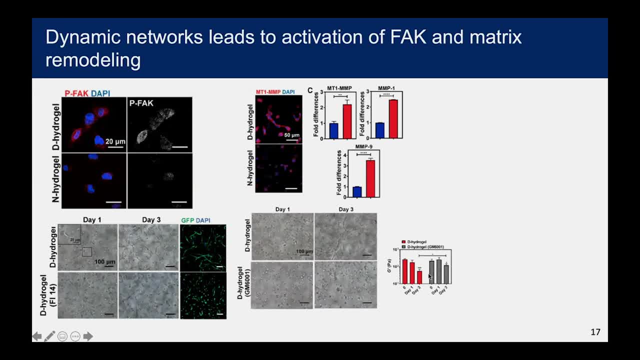 that is seen here with the reduction in stiffness it's slowing down with that inhibition Nicely. the cells would also produce their own extracellular matrix, both collagen four and laminin. And you can see here very nicely in red the collagen four is deposited. 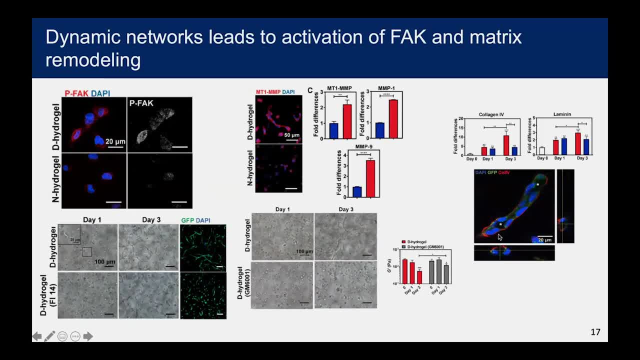 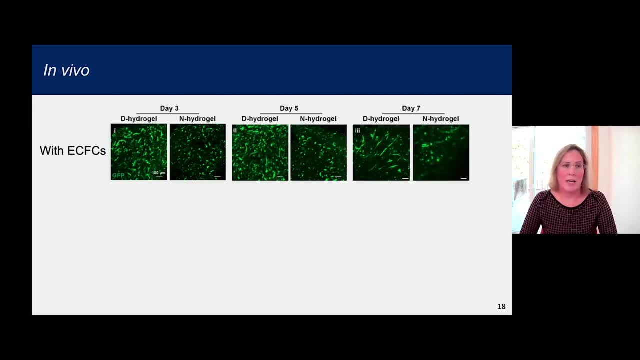 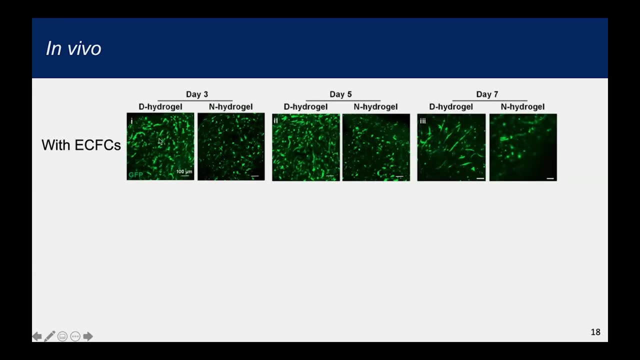 around a luminal structure in the dynamic hydrogels. Finally, we also examined the relevancy of the system for in vivo, as we were thinking about therapeutics and we injected them with the endothelial colony forming cells. We can see here network forming. 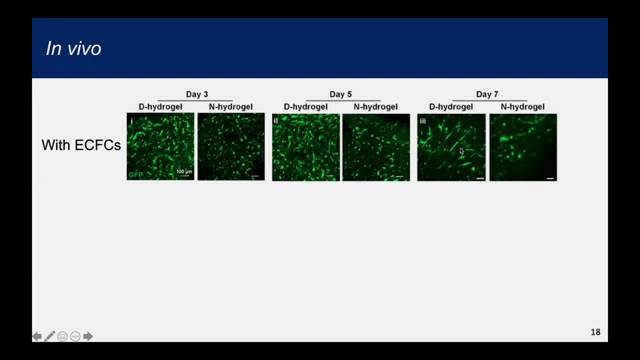 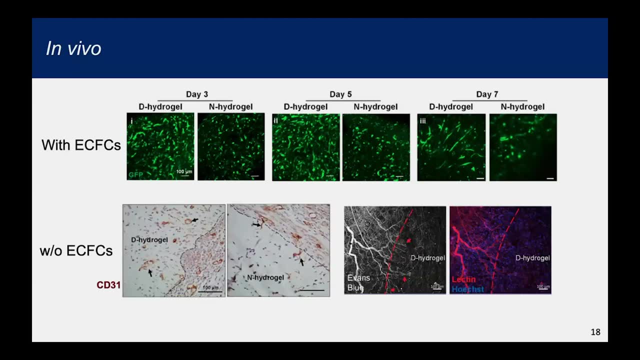 and the dynamic hydrogels. And here, day seven, we'll see a larger vessels in those hydrogels And we can also see. we can also see. we can also see when we inject the cells and this was done subcutaneously. 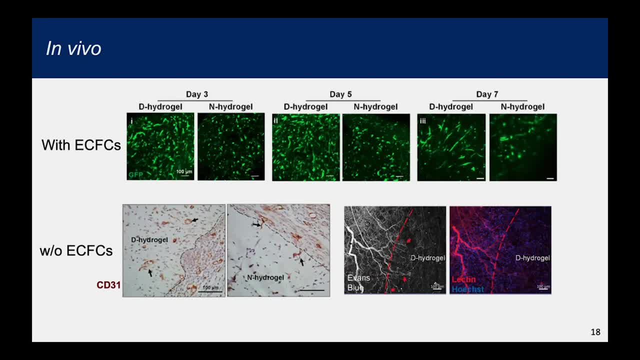 when we inject these cells with no cells, we see that these hydrogels, sorry, inject the hydrogels. we see that they encourage angiogenesis by these CD31 positive cells in the dynamic hydrogels which we could barely find in the non-dynamic hydrogel. 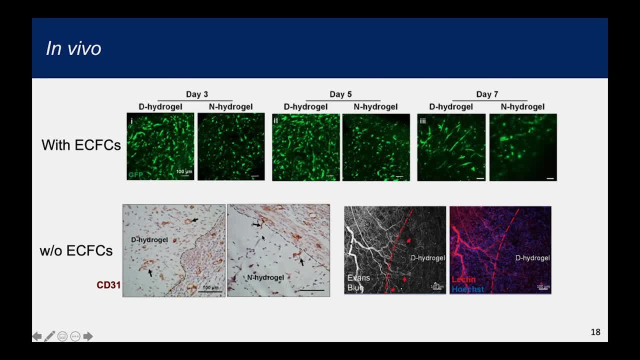 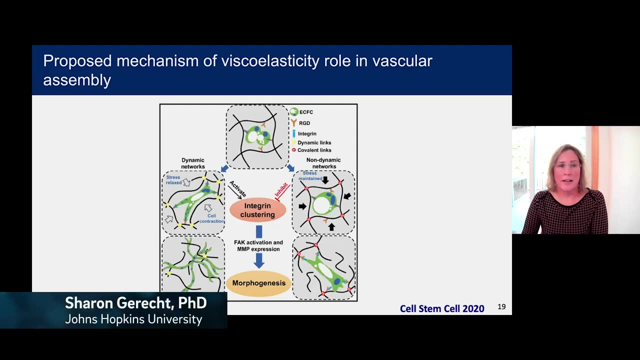 And if we found them, they would be typically at the interface between the tissue and the hydrogels. By injecting to the tail vein either Avans, blue or lectin, we also confirm the functionality of those angiogenic vessels. We concluded that the dynamic networks 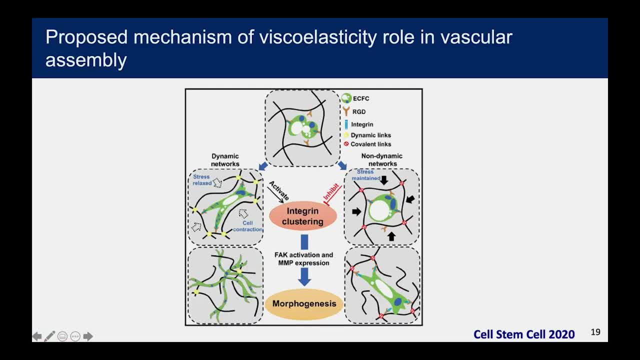 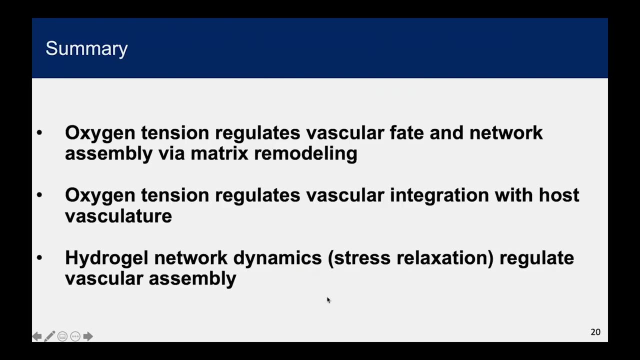 allow the cells to contract and this activates integrin clustering, followed by focal adhesion activation, MMP expression and also extracellular matrix deposition, and all of that allow for a morphogenesis to happen. And with that I'm going to finish. 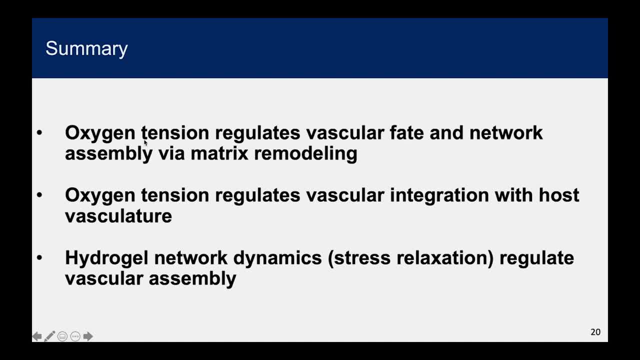 I'm just going to summarize that we found that oxygen tension regulate vascular fate using a matrix remodeling and it's also regulates vascular integration with host vasculature and that's a hydrogel networks dynamic of viscoelasticity regulate vascular assembly. Just to thank all the people that done the work. 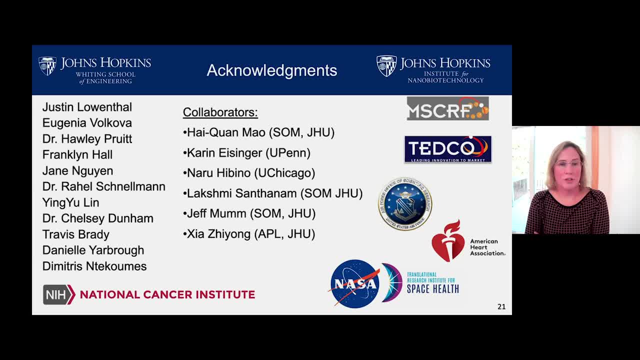 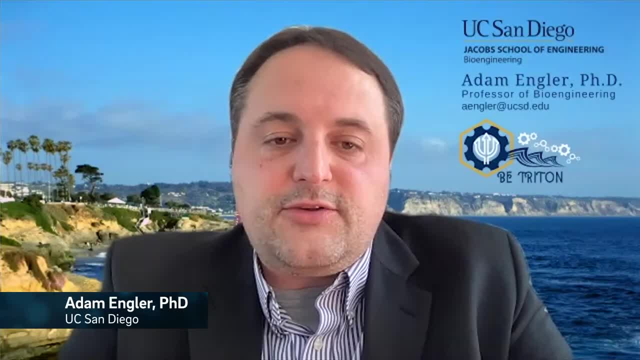 I tried to mention throughout the presentation, of course, our collaborators and our funders. Great, thank you so very much, Sharon, for the presentation. So next we're going to turn things over to Dr Laura Nicholson. So whenever you're ready to go. 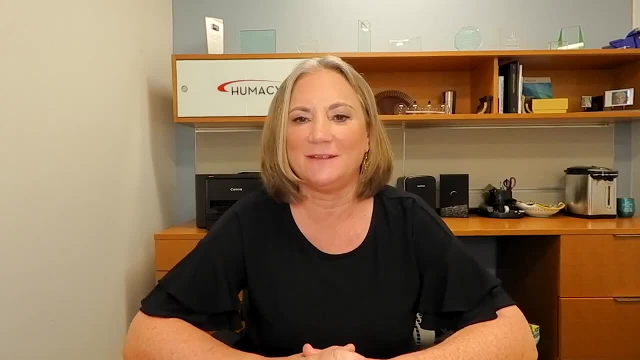 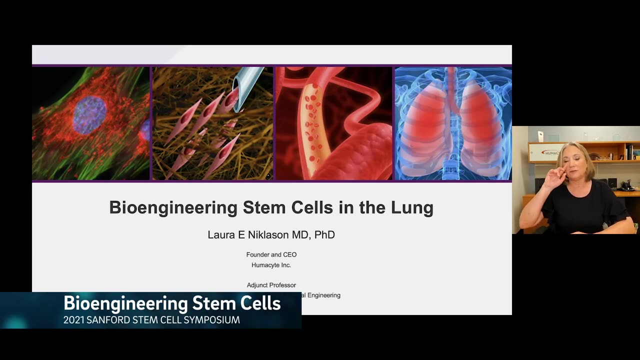 Thank you very much, Adam and the organizers, for being able to participate in this meeting. So I will continue the theme a little bit to talking about the use of stem cells in regenerative medicine, but my focus is going to be on lung engineering. 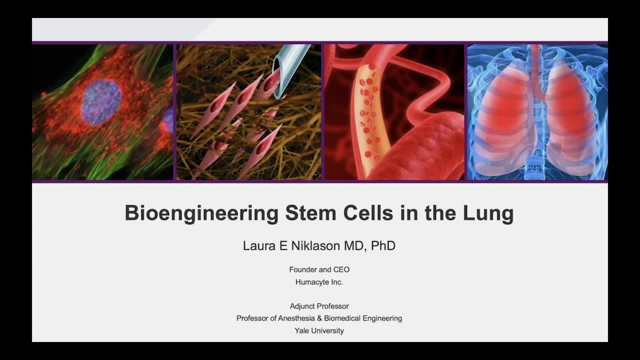 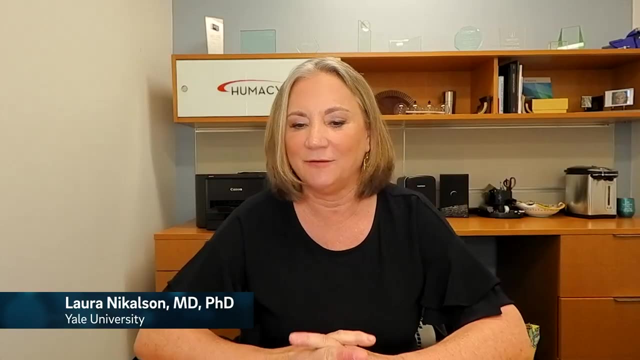 So I know that Adam mentioned that I founded Humacyte. In fact, about a year ago I became the CEO of Humacyte, And so I'm now an adjunct professor at Yale. My lab still runs there, but the vast majority of my time is spent in my offices. 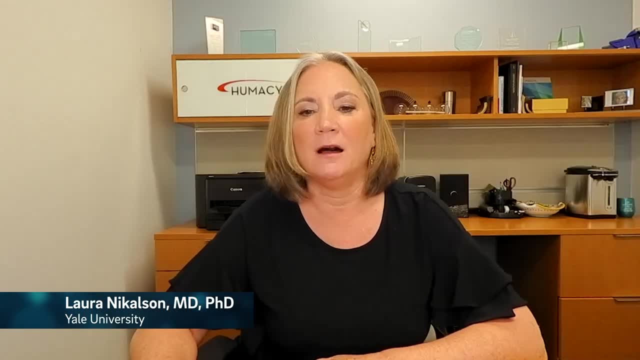 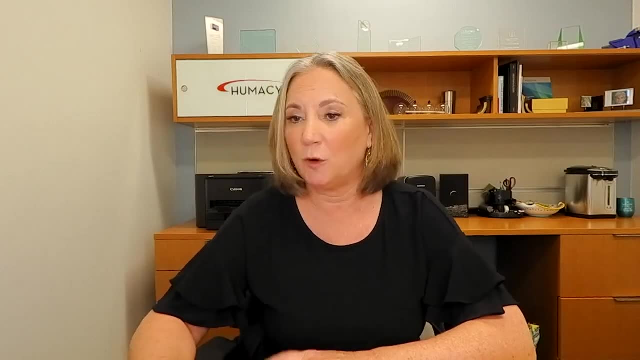 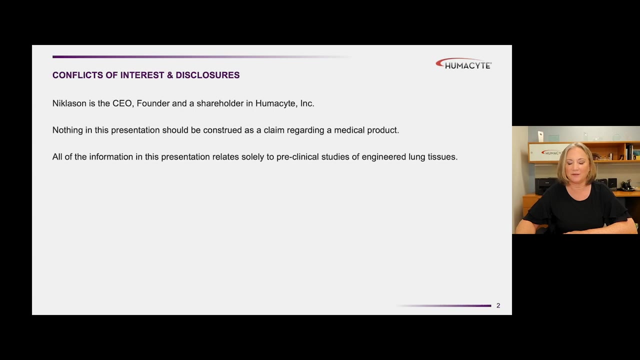 at Humacyte, where we're growing engineered vessels for clinical use. But I would say that in this talk I'm not going to focus on vascular engineering, but more on lung engineering, And so the content in this presentation really is not related to any clinical products. 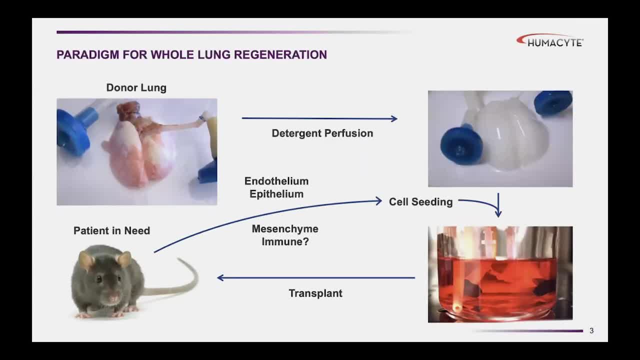 at least not yet. So I'd like to talk about our approach to whole lung regeneration. This is an effort that we started in my lab at Yale more than a decade ago, And we were one of the first groups to show the feasibility of decellularizing native lung. 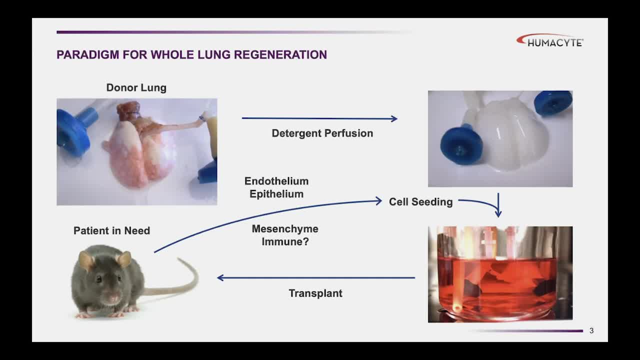 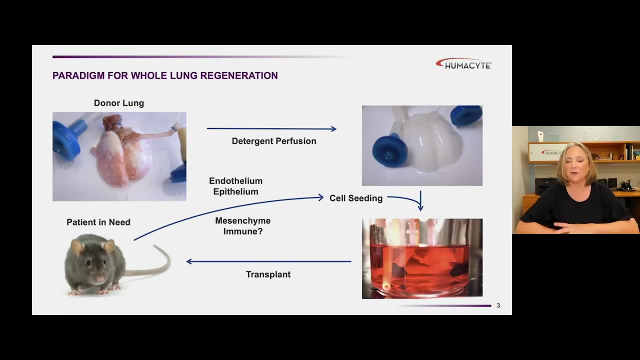 and then repopulating that acellular matrix with cells, lung cells, such that we could reconstitute an organ that could actually participate in gas exchange for a few hours. This report came out in Science in 2010.. And, frankly, at the time when we showed 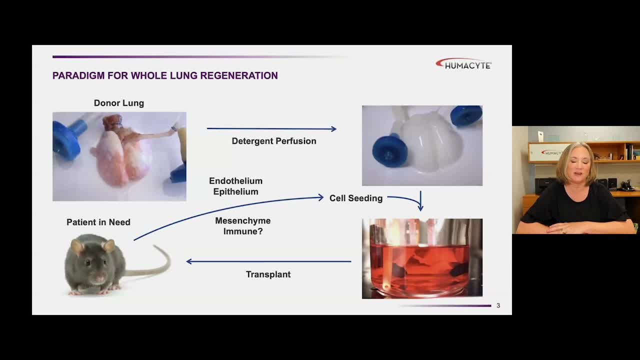 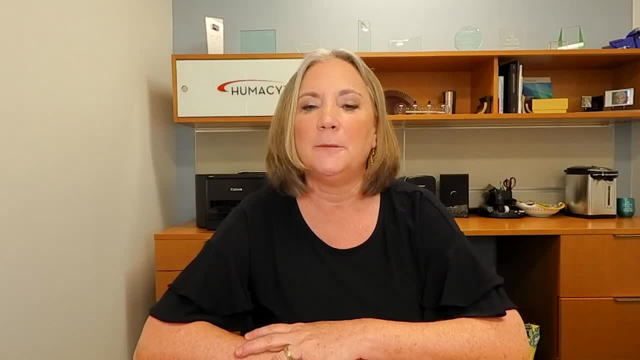 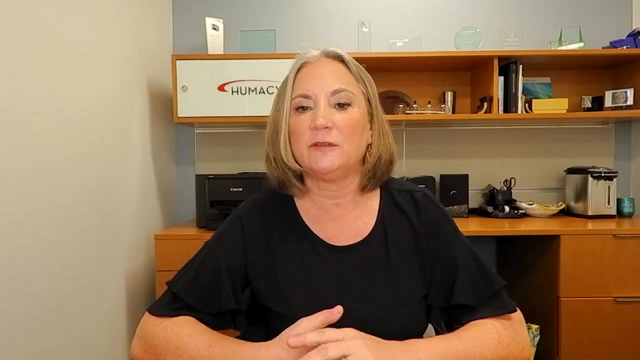 that we could repopulate an organ and achieve gas exchange, even for a short period of time. I was actually flabbergasted that that was possible, But since that time we've really been working from these initial prototypes and really trying to hammer out some of the obstacles. 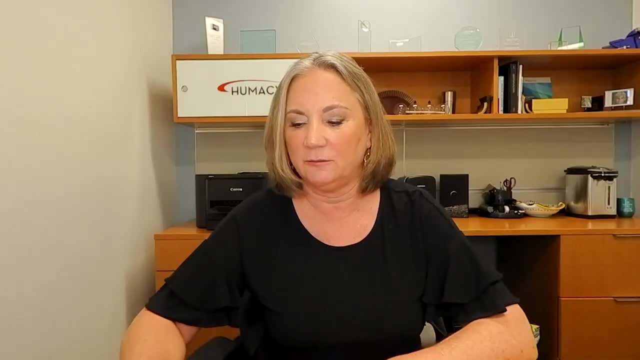 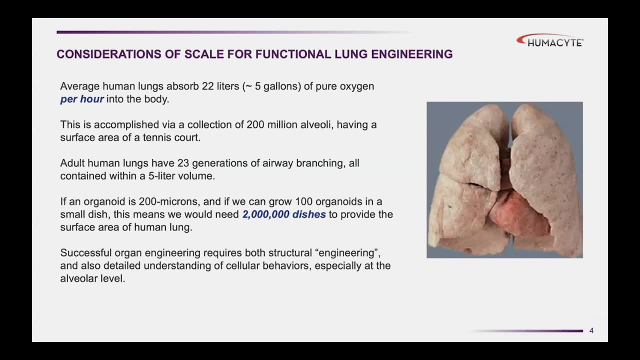 that stand between us and engineering a lung that can exchange gas in the long term. So, as I always say to my students and postdocs, you know it's important when you're thinking about regenerating a tissue that you want to be functional, it's critical that you think about the key, what we would call 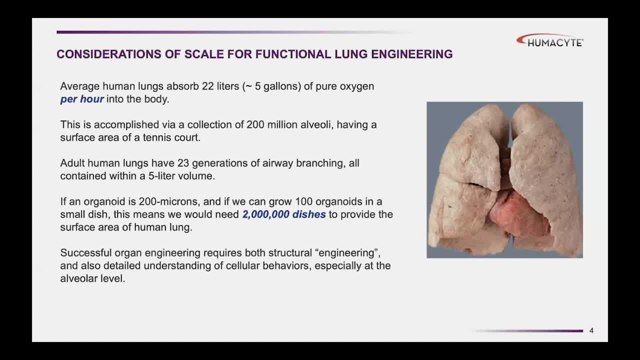 design criteria that go into whatever you're going to engineer that's going to really drive function. And there are some fun facts about the human lung. You know the average human lung absorbs about five liters of pure oxygen every hour, which is actually a large volume of gas. 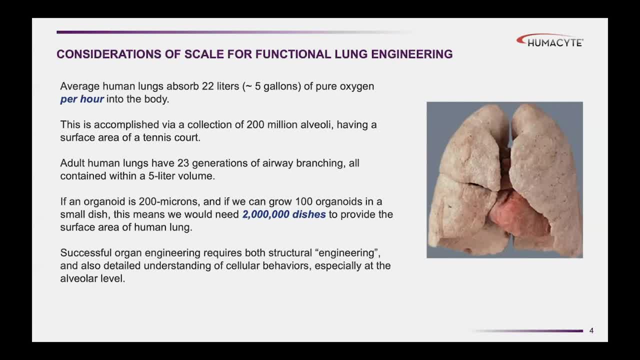 And it also excretes a similar volume of carbon dioxide every hour. This is accomplished through 200 million alveoli, each of which is about 200 microns in diameter, And with the 23 generations of airway branching, there's actually roughly. 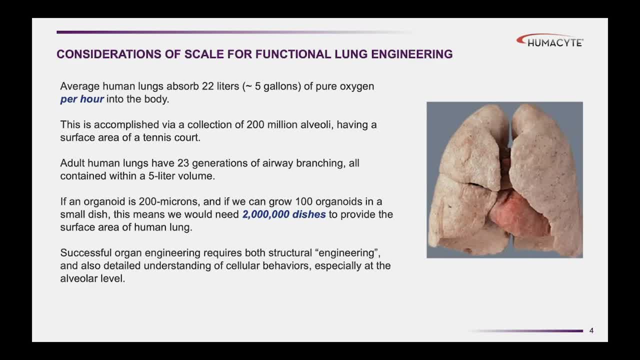 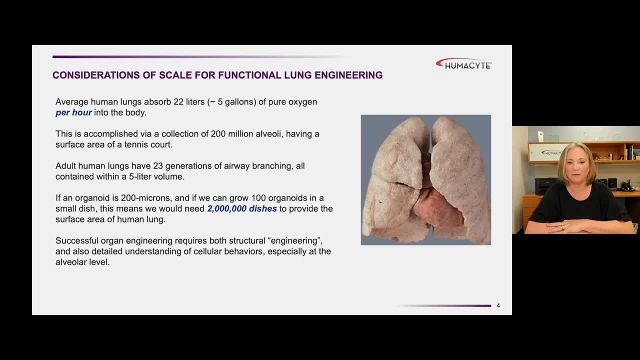 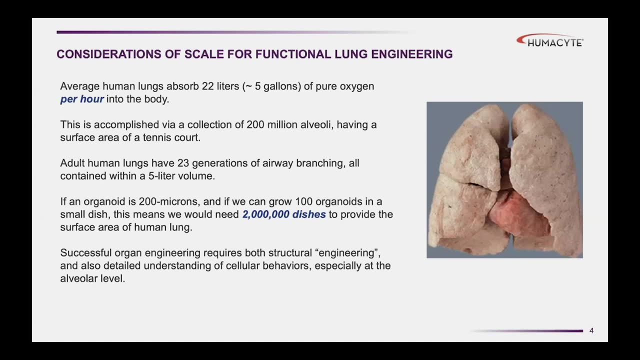 a 70 square meters of surface area in your chest which is useful for gas exchange and which provides this highly efficient gas exchange surface area, But if we think about what it would take to reconstitute a set of functional human lungs- one of my favorite facts that I 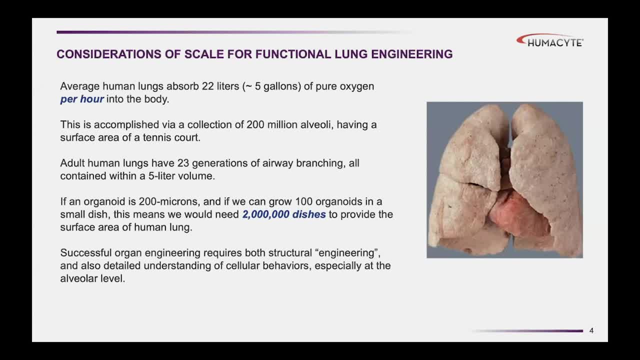 tend to quote with stem cell biologists actually is that if we had organoids that we were growing in hydrogels and if each of those organoids was 200 microns in size, we would need roughly 2 million dishes to get enough organoids to reconstitute a full 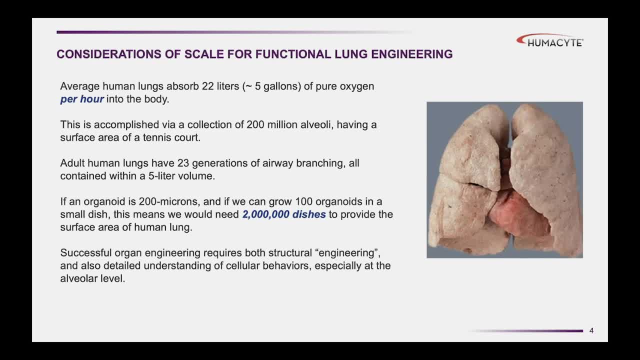 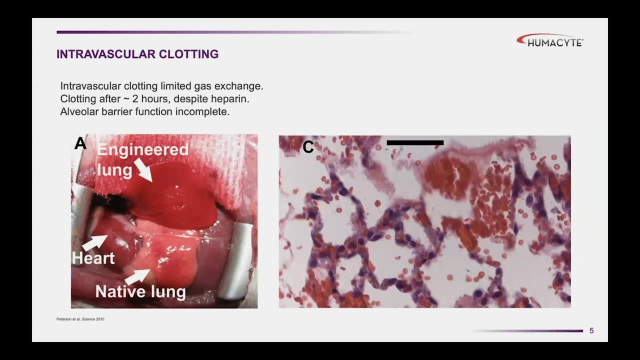 human lung And so clearly just growing small, small little organoids that represent individual alveoli is is not going to get us really to a functional organ. So, as I mentioned, we have in our early studies. we took a cellular lung matrices that we carefully decellularize to 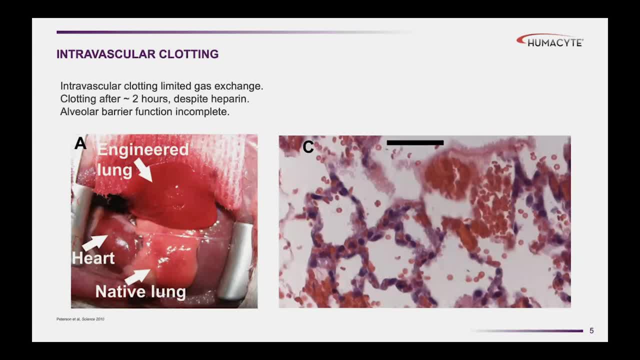 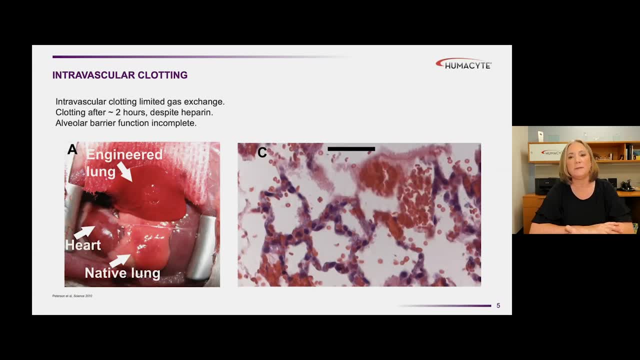 really retain the alveolar structure, And so we're going to have a lot of organoids that are in the microvascular structure. And when we repopulated these organs and then implanted them in vivo, what we found was that the primary failure mode actually was intravascular clotting. 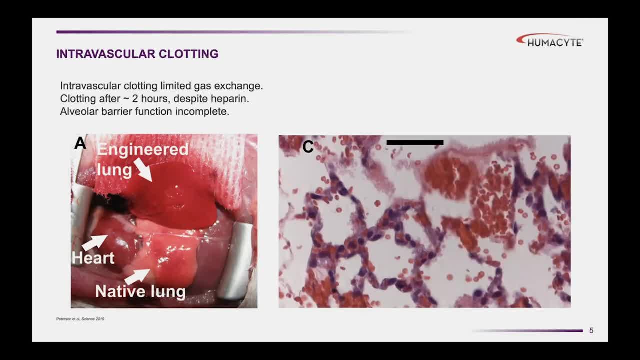 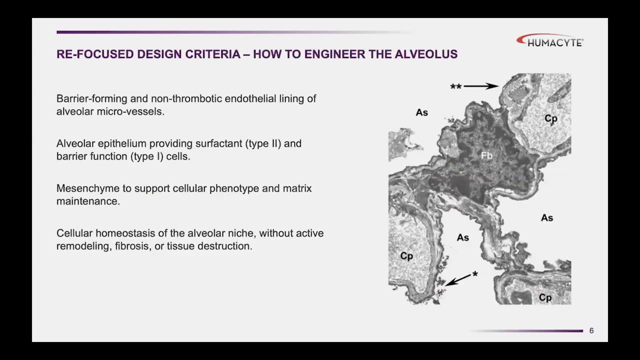 So you can see an engineered lung that had been implanted into a rat for several hours on the left, And what you see is that it's sort of this beefy red appearance, And that's because there was a lot of microvascular and intravascular coagulation. So this really led us to think very. 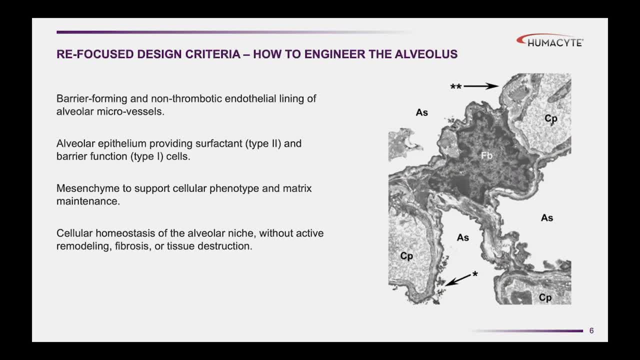 carefully about the alveolus, which is really the functional unit for gas exchange in the lung. And really the alveoli in your lung are replicated millions of times over and they're a fairly stereotypic structure. They contain about six or seven different cell types, including 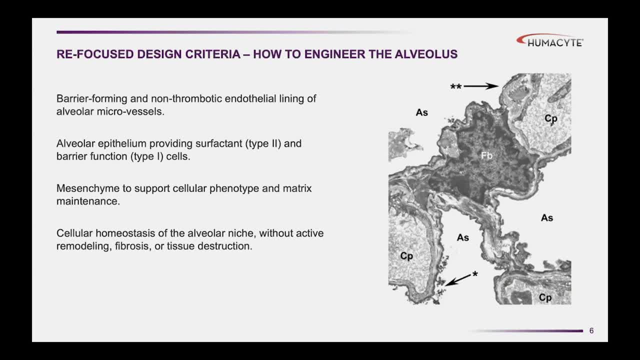 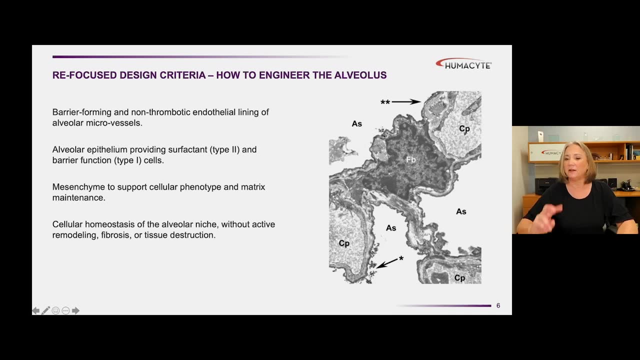 microvascular endothelium on the vascular side of the barrier, but also a collection of fibroblasts which sit in the septae, in the wall of the, the alveoli, And also they contain epithelial cells, actually of two flavors: type one and type. 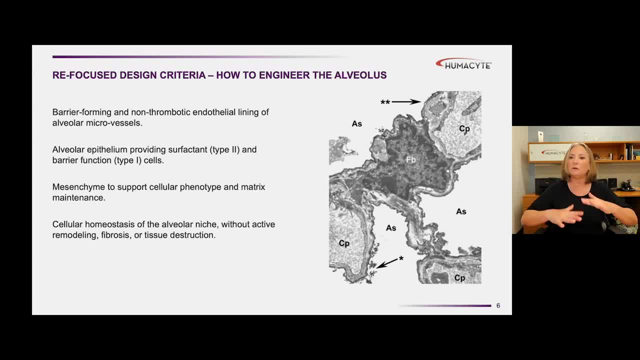 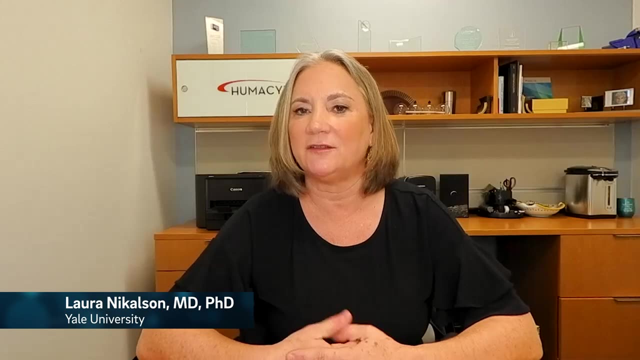 two epithelial cells And the type one epithelial cells really stretch over the surface of the airway and sit right on the other side of the basement membrane, right next to endothelial cells, And I'll show you later on in this talk that we've done some single cell analysis to try. 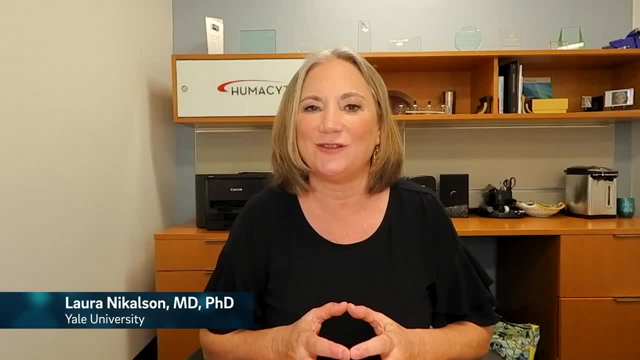 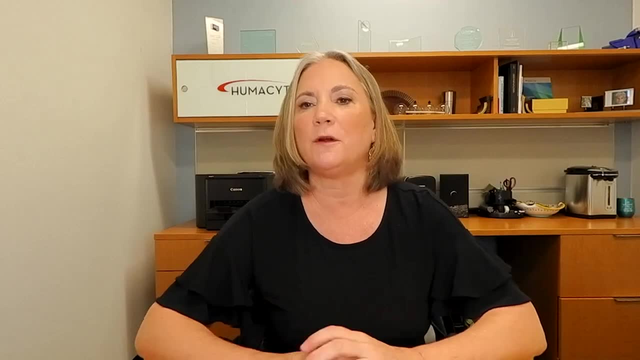 to understand how these neighborhoods or collections of cells talk to each other in the normal alveolus. But but just to start, you know, this just sort of orients you to to the different types of cells that are located in the air set. 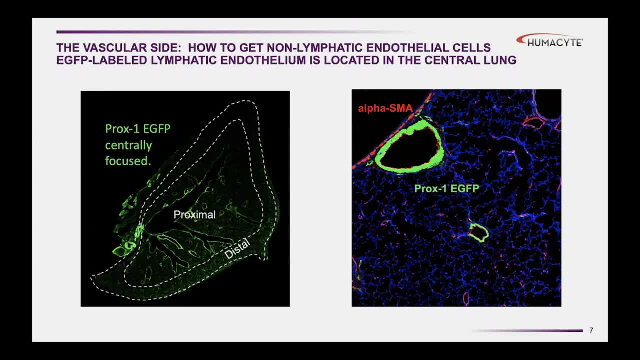 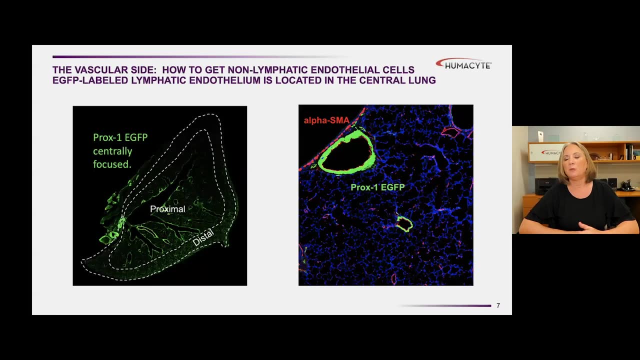 So when we began focusing more on on providing a a stable and complete endothelial layer in the vasculature in order to avoid clotting once we implant the lungs into, into native living animals, We realized at first that that there's actually two flavors of endothelium: two, two broad flavors. 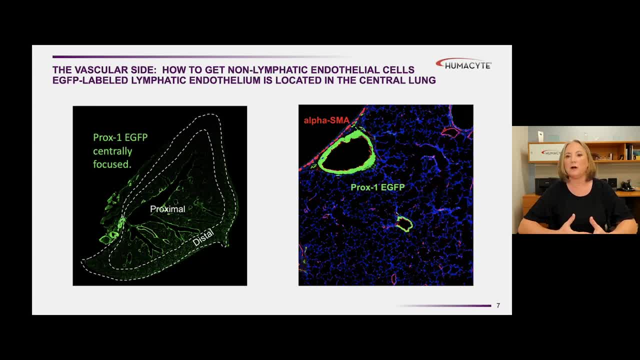 of microvascular endothelium in the lung. One is what we call blood endothelium, which it comes in contact with the bloodstream. But another form of endothelium is lymphatic endothelium, which, as as the name implies, aligns all of the ducts of the lymphatic system, And there's actually a large 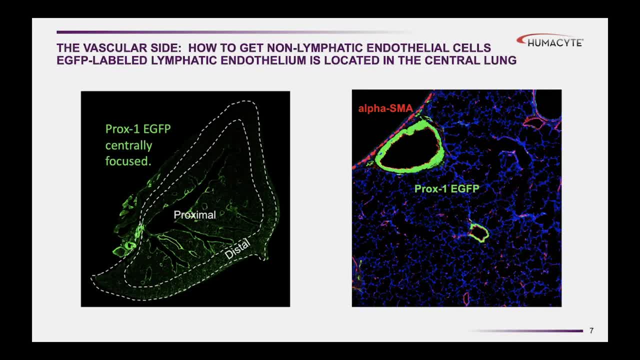 lymphatic system in the lung that's very active. The endothelium of the lymphatic system is a system that's very active And it's very active. And the lymphatic system is, by by design, much leakier than the endothelium of the of the blood. 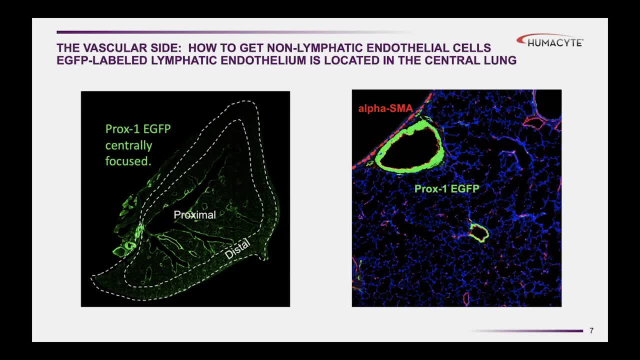 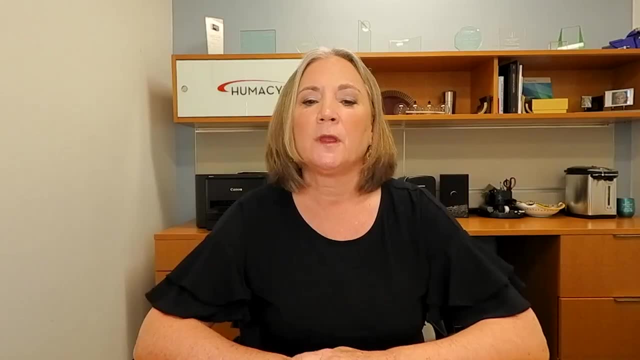 system, And so we became interested in really identifying the endothelial cells of the lung, that would be blood endothelium as opposed to lymphatic endothelium. And blood and and and and lymphatic endothelium share a lot of markers, but there are some distinctions. So we obtained a 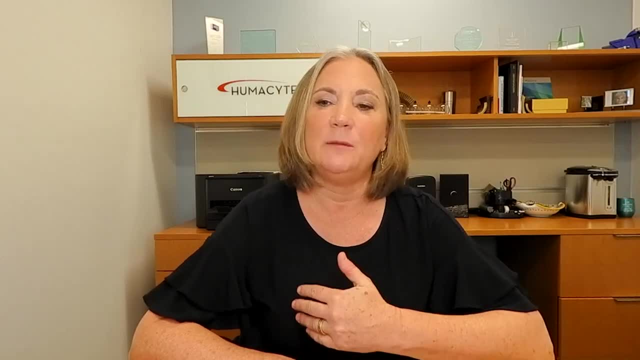 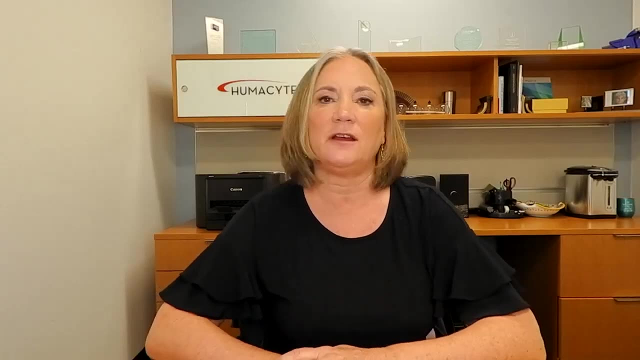 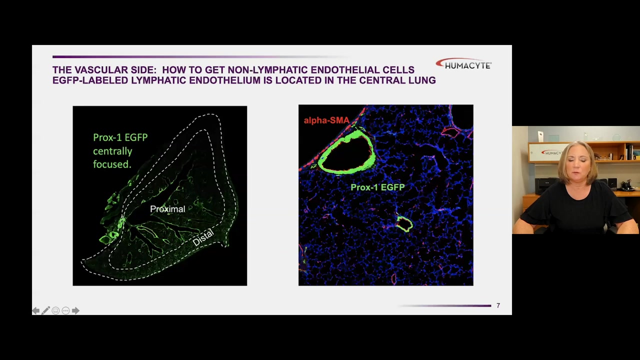 a transgenic rat that labels all of the the lymphatic endothelial cells with EGFP. And these lymphatic endothelial cells express a transcription factor called PROX-1.. So, as you can see in this image, on the left in the central, 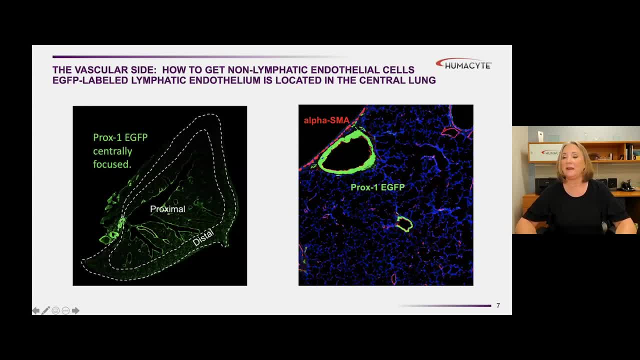 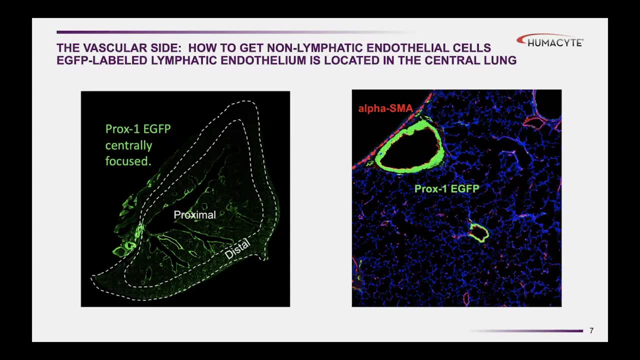 portion of the lung is particularly lining the airways, is where the majority of the lymphatic endothelium resides, and that stains green, And so we were able to develop cell sorting methods whereby we could digest a whole rat lungs from these PROX-1 cells, And so we were able to develop 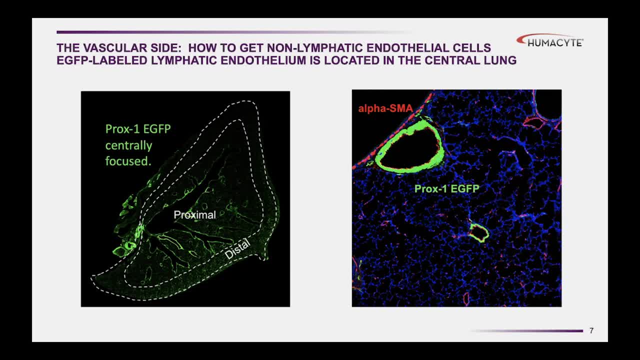 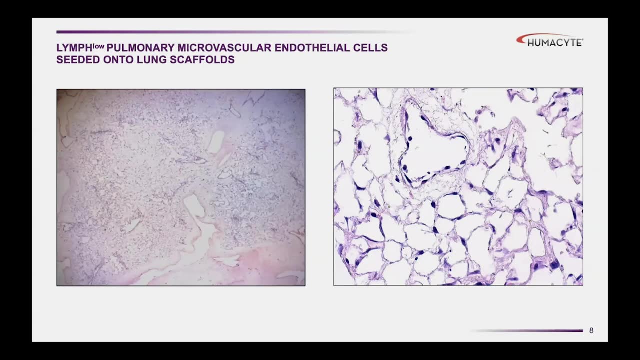 these PROX-1 GFP rats and really select out the endothelium that was negative for GFP so that we were really getting a purified cell collection of blood endothelium which would presumably have higher barrier function When we took these endothelial cells and seeded them into a cellular 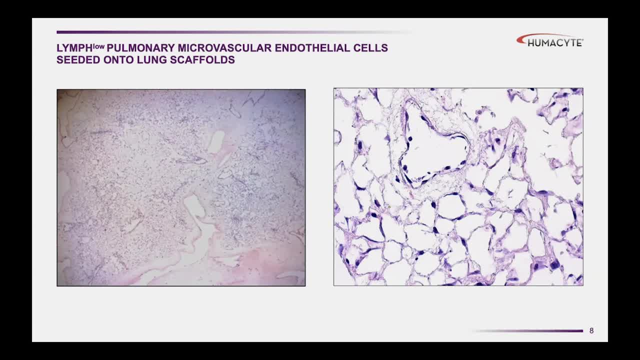 lung scaffolds that we had decellularized in the rat. you can see it in a low power image on the left that we were able to get fairly broad coverage of the microvasculature and the larger vessels in the lung. And you can see on the right 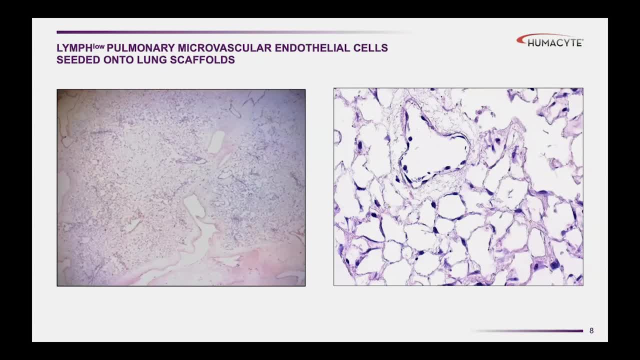 that this is an example of blood endothelial cell seeding into the acellular lung matrix And you can see that many of these cells permeate into the small microvasculature in the septa surrounding the alveoli. When we look at marker expression of these cells that are seeded into 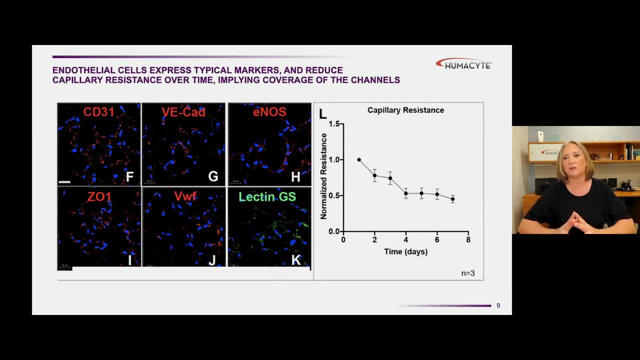 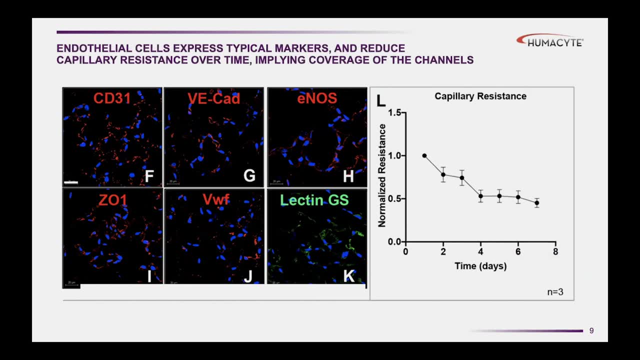 the lung. we can see that they are seeded into the lung, And so we can see that they are seeded into the lung, And so we can see that the blood endothelial cells express a lot of markers that we would expect to see in native microvascular endothelium, including CD31, V-cadherin. 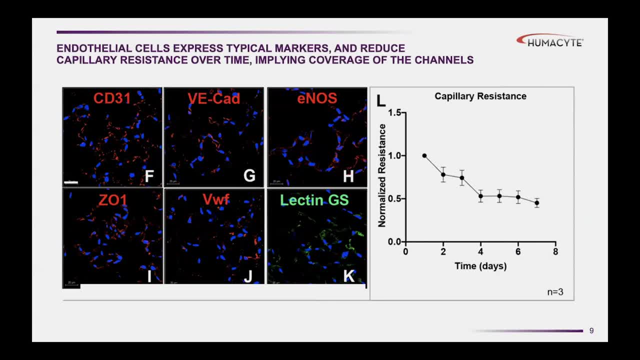 endothelial nitric oxide synthase, VWF, and also Zona occludens 1, which is an important molecule for forming tight junctions and forming barrier in between endothelial cells. And, as you can see from this image on the right, when we measure the resistance of the capillary bed which we're able, 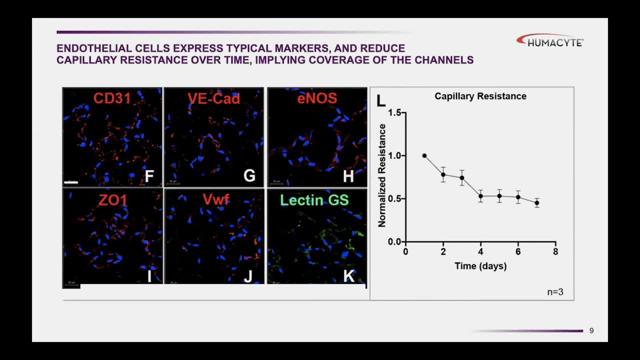 to do by flowing culture medium through the vasculature and by measuring pressure drops across the vasculature over time and we can calculate a capillary resistance. what you can see is that over time, as the endothelial cells migrate into the microvasculature and begin to 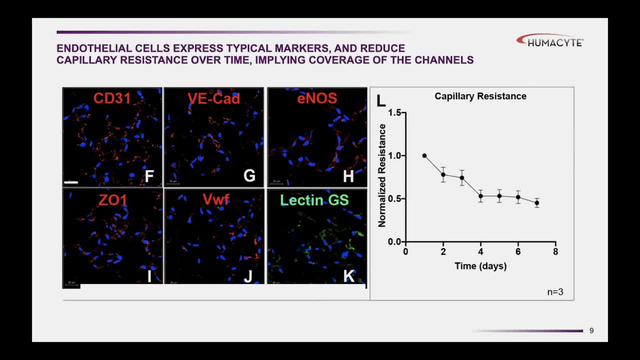 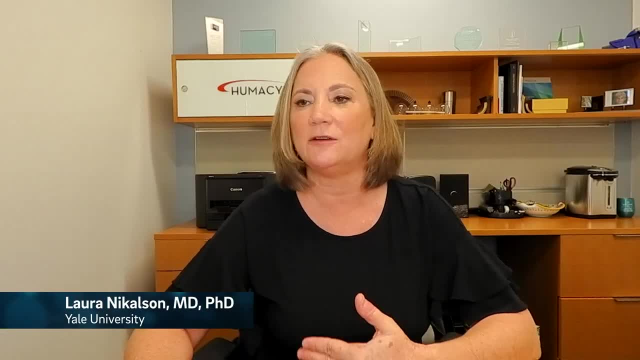 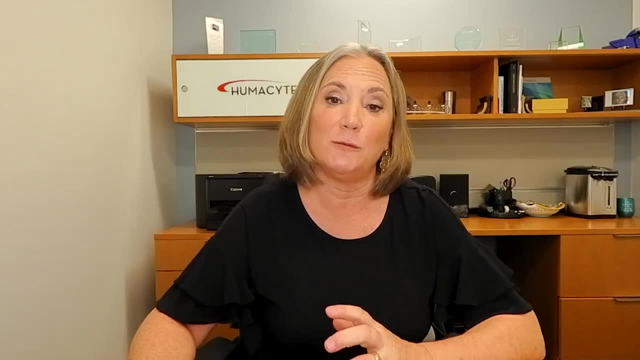 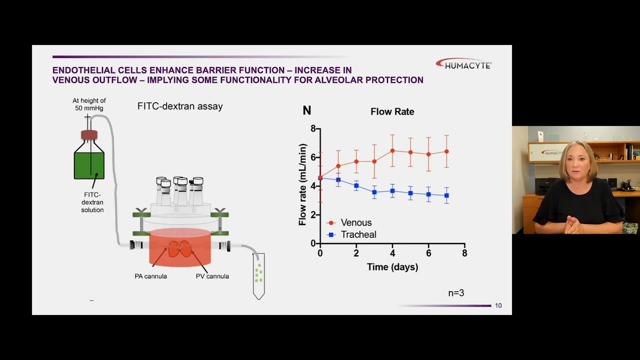 line the conduits, we see that the capillary resistance actually goes down over time, And we viewed these as sort of positive indicators that that the endothelial cells were adhering to the walls of the of the vessels and doing what they were supposed to do. We then also performed assays that measured not just the resistance of the 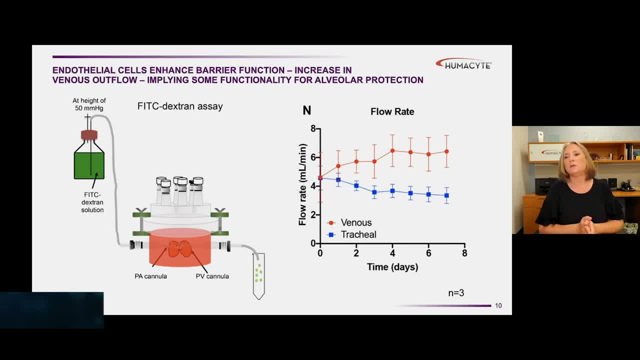 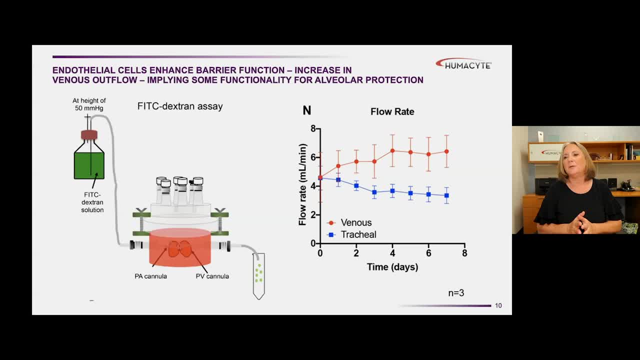 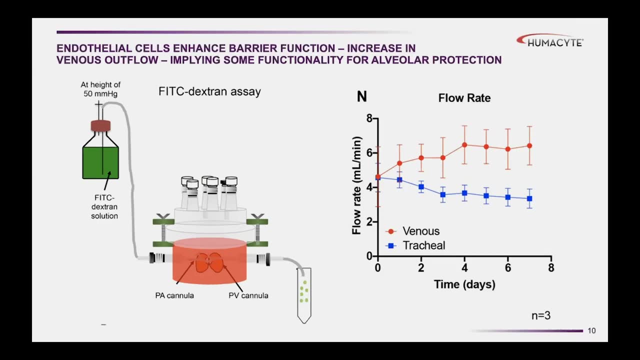 and the blood in the microvasculature of the lung, And so the ability to recapitulate that barrier function so that you don't get transudation of fluid across the alveolar barrier is really a key aspect of whole lung engineering. And what we found when we measured a barrier function or 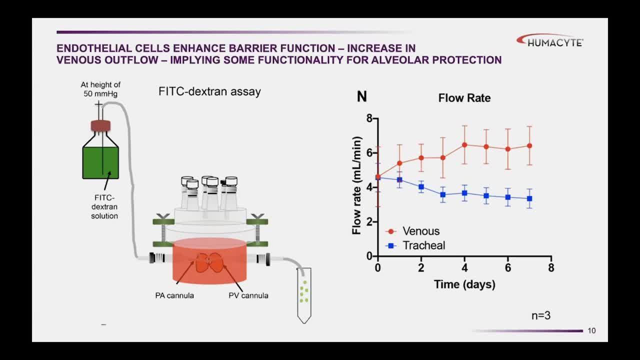 or essentially flow rate, liquid flow rate- going across the the alveolar barrier from the vascular compartment into the airway compartment. what we found is that the alveolar barrier is not. that flow across that barrier tended to go down over time as the endothelial cells were cultured. 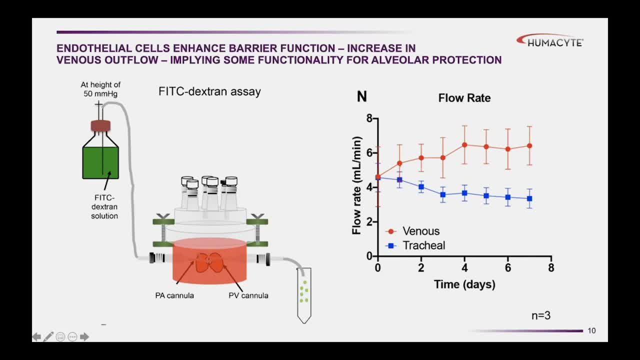 in the vasculature And you can see this image on the right. these blue squares show that there's a slight decrease in fluid flow across the barrier And going along with that, there's a concomitant increase in vascular flow that enters the pulmonary artery and then exits the pulmonary. 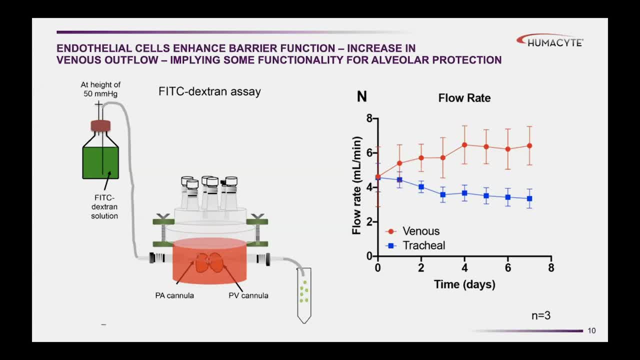 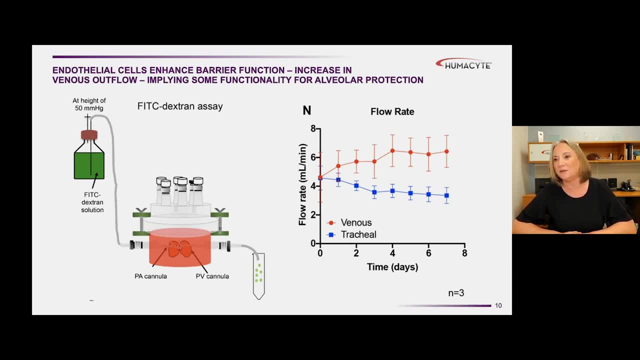 vein, And while these are both things that we would like to see, what's important to note is that the flow rate in blue boxes here certainly does not go to zero over time, So that means that there's still quite a bit of fluid transudation from the vasculature into the airways, And 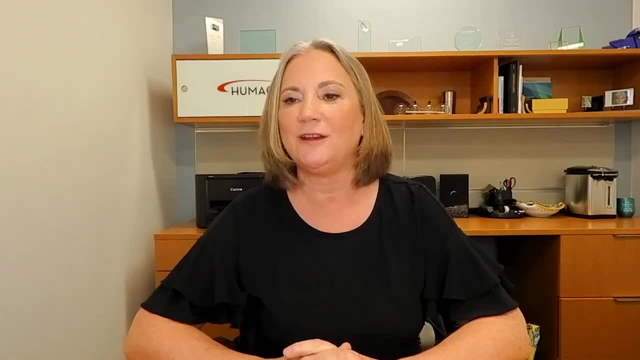 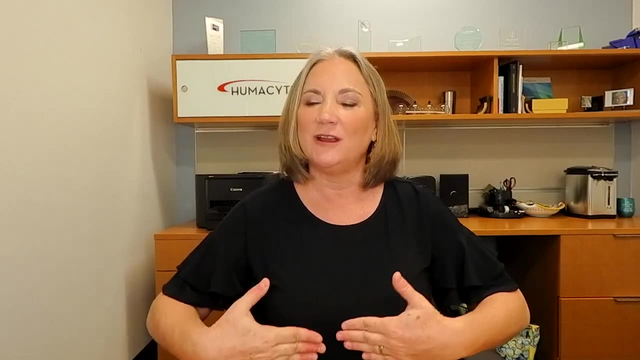 that's a nice way of referring to drowning actually. So if you put a lung that's very leaky into an animal or into a human, then you'll get that fluid transudation into the airways and you'll basically drown the recipient. 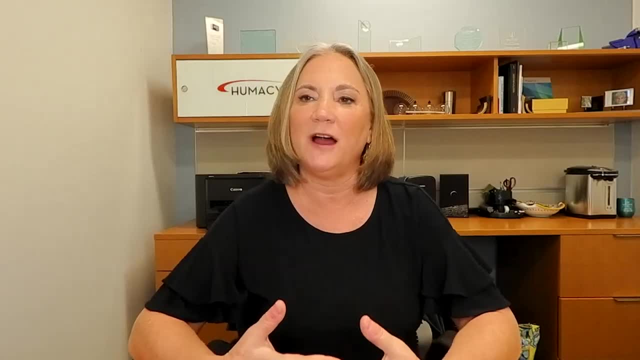 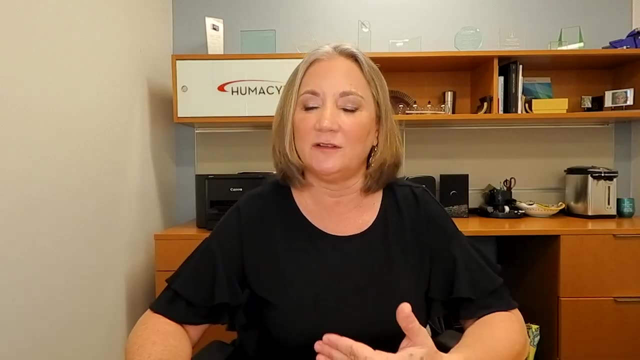 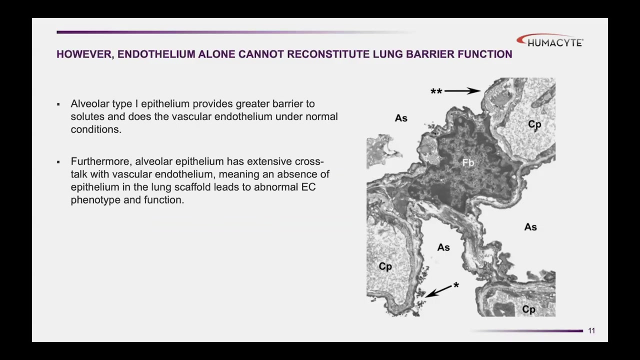 So the message here is that, while providing blood endothelial cells into the microvasculature certainly helped with decreasing resistance and increasing barrier, and while it was helpful in our hands, it was not sufficient. So, then, that caused us to look a little bit more carefully at not just the endothelium on the vascular side. 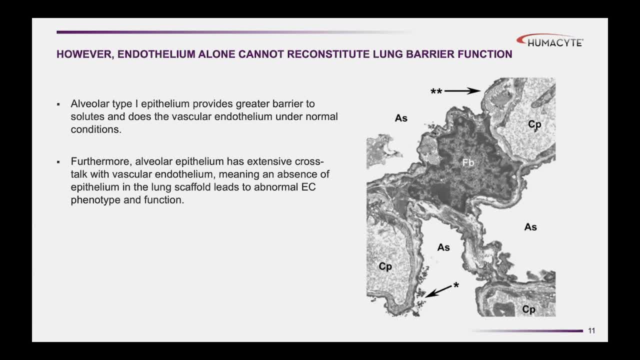 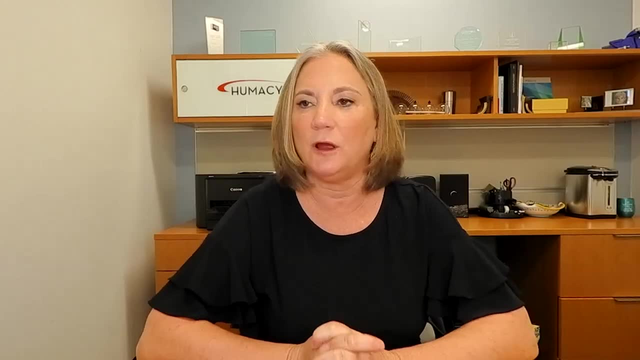 but also to try to understand how the endothelium interacts with other cell types in the alveolus to maintain homeostasis and also to try to maintain barrier function, And this led to a set of experiments that was done by a very talented graduate student in my group named Katie Leiby. She's an MD-PhD. 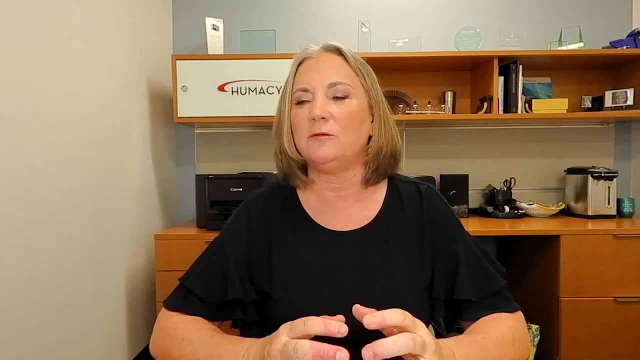 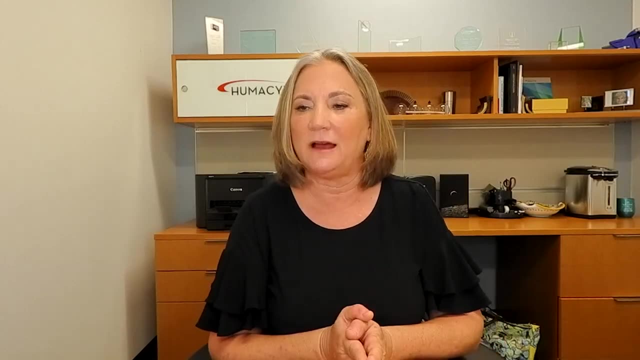 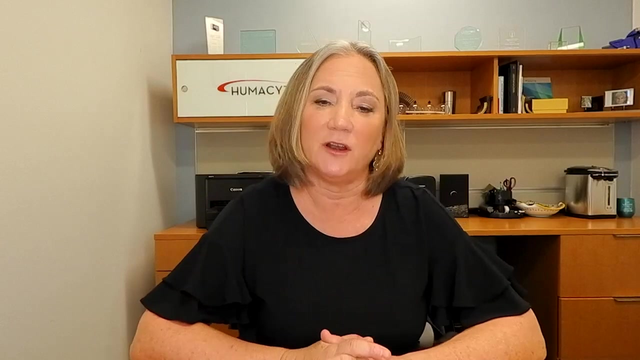 student, And what she wanted to understand was the impact of different cell types, particularly endothelial cells, but also alveolar fibroblasts, And so what she did was she did a lot of research on alveolar fibroblasts, on the differentiation and the growth of the epithelial stem cell of the 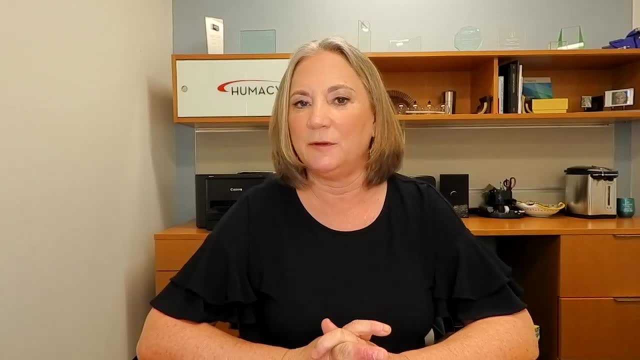 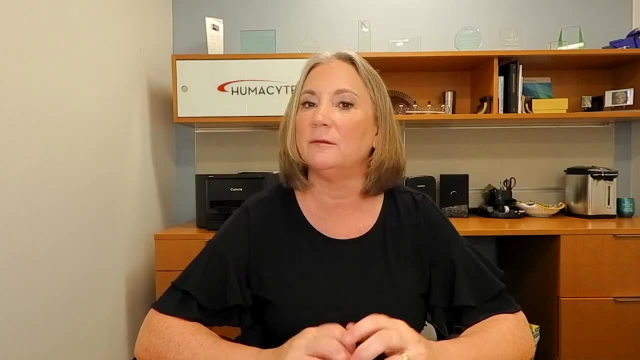 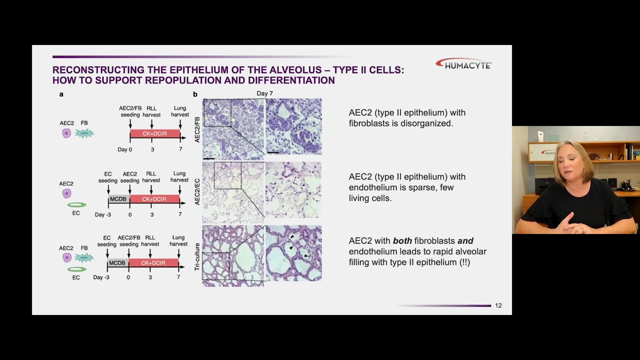 lung, which is really the type two alveolar epithelial cell. So in our alveoli there are really two flavors of epithelium. They're the type two cells which make surfactant and which allow our lungs to expand, but they're also the local progenitor cell for the type one epithelium. 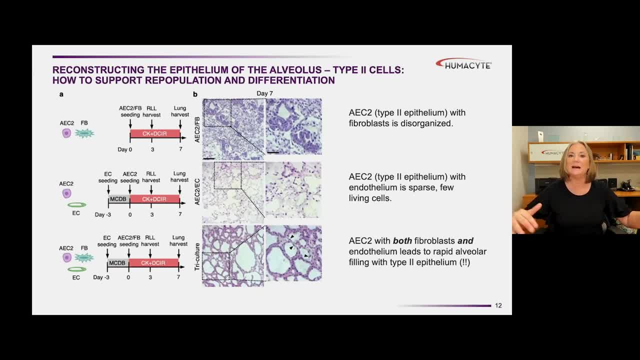 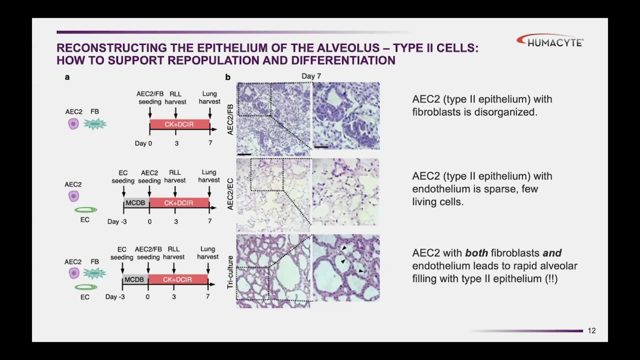 And the type one epithelial cells are the epithelial cells that really line most of the surface area of the alveoli and provide a lot of barrier function. And so what Katie found is that by combining a really type two epithelial cell conducive medium, combining that with co-culture with both fibroblasts and endothelial cells, 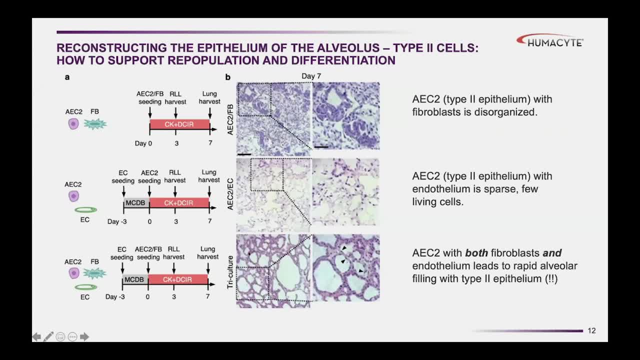 she found that she was able to form really dense rings of alveoli that were lined almost entirely with type two epithelium, which is actually kind of an extraordinary finding, because it means that she was able to essentially reconstitate the epithelial component across an entire organ in a fairly organized 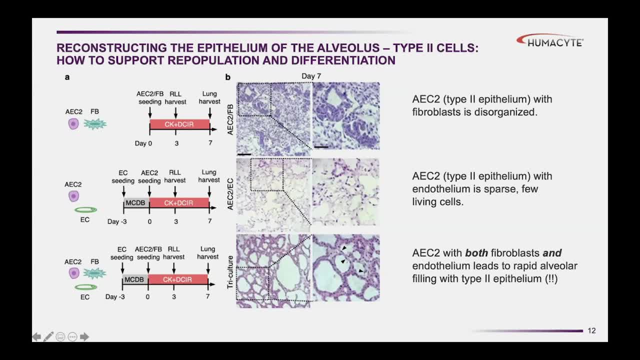 fashion. What she also found was that when she just seeded the epithelial progenitor cells just with endothelium that the growth of the epithelium was not so great. So she found that epithelium was poor and if she seeded them with just fibroblasts that there was a lot of 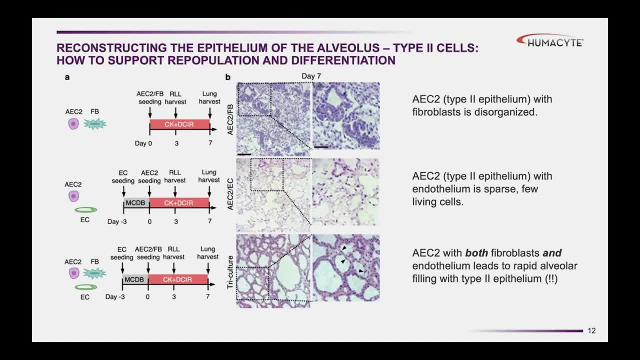 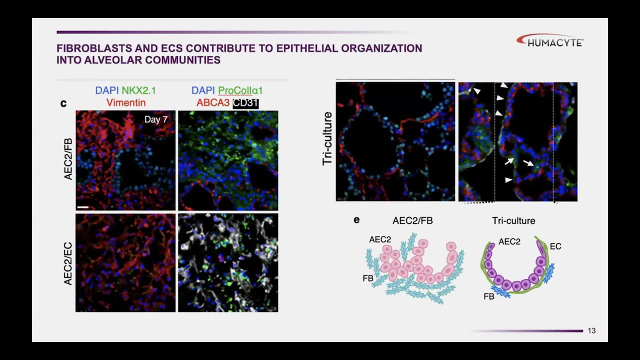 epithelial cell growth, but it was very disorganized. So having these two other cell types was really pivotal for generating alveolar structures that contain really robust epithelium. And if we look at this a little bit more closely again, there's some immunostaining here for some. 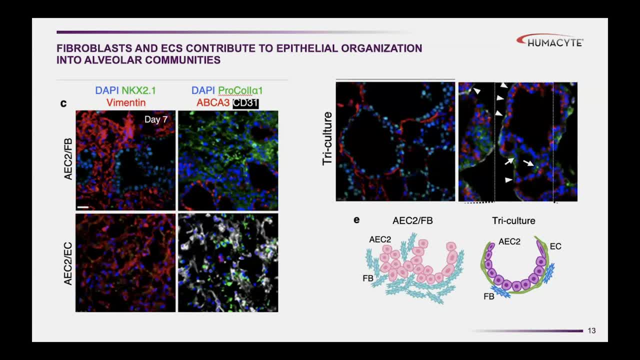 markers that may not be familiar to some folks if you don't think about lung all the time, But essentially what this staining, what this shows, is that in triculture lungs we got a tremendous amount of what we would call native alveolar markers, including type 2 markers, which is ABCA3, and also vimentin and 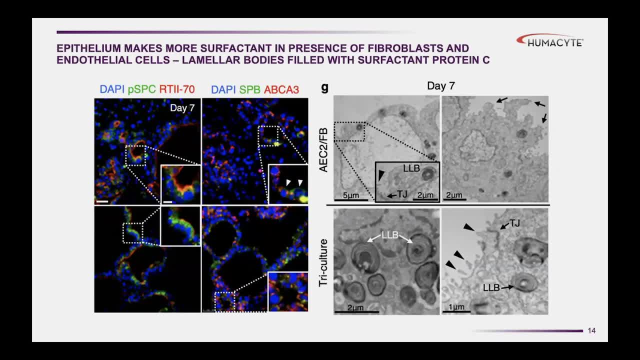 NKX2.1.. This just shows even a little bit more detail looking at the functionality or the ability of these type 2 cells to make an important, you know, function. And then we also have a molecule which is surfactant molecule, which allows our lungs to 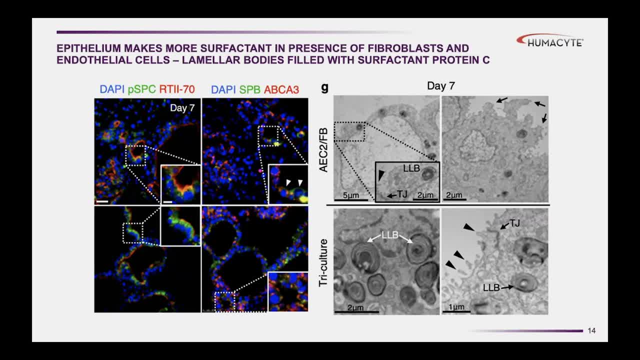 inflate and lowers the surface tension in our lungs. Surfactant molecules are stored in lamellar bodies and you can see that in triculture the type 2 cells have huge numbers of lamellar bodies which contain surfactant that's waiting to be released. 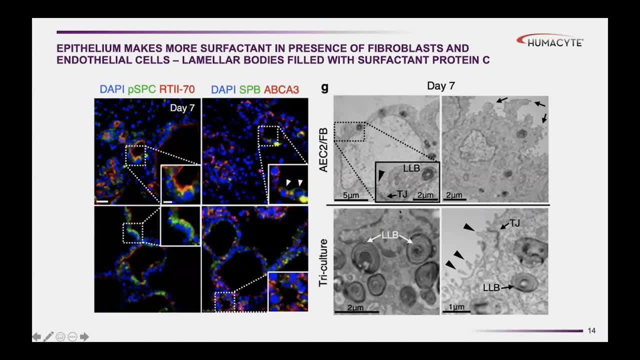 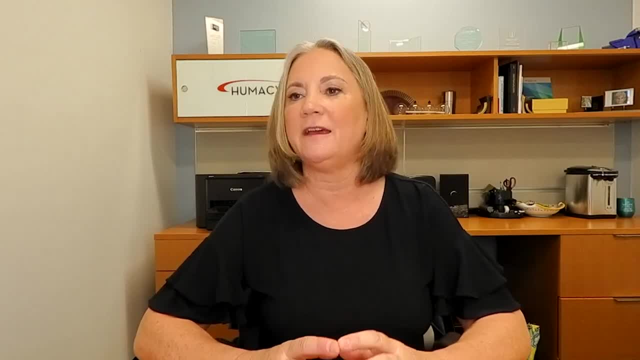 from the cells And when we don't have triculture, we see many fewer of these lamellar bodies. So what we're trying to do is focus a little bit on some of our single cell work that has really tried to understand what are the conversations that are going on between the different cells in. 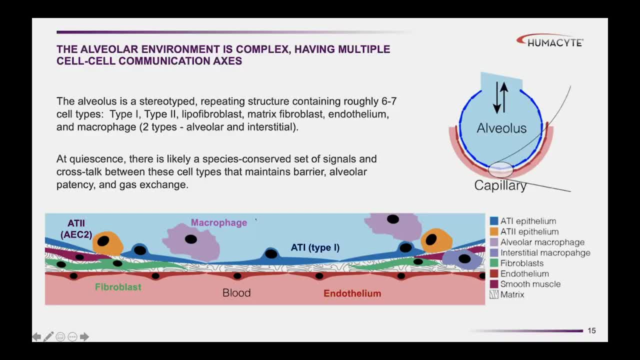 the alveolus. So this is really a cartoon of these different cell types that we think are important and are present. As I mentioned, there's the type 1 epithelial cell, which covers most of the alveolus. There's the endothelium, the blood endothelium, which sits on the other side of the basement. 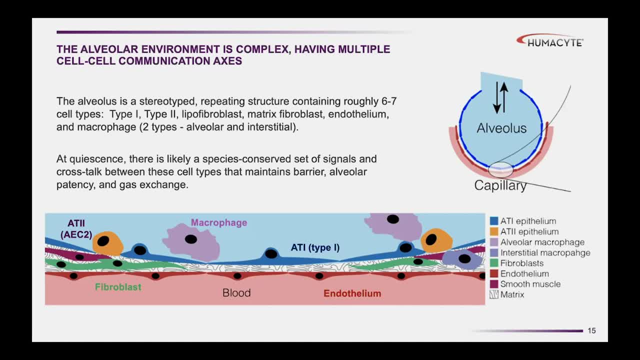 membrane, The cells that cover most of the surface area, are really separated by only about 500 or 50 or 100 nanometers, So it would not be surprising if those two cell types actually had very active conversations with each other. But in addition, there's type 2 cells, there's macrophages and there's a couple different flavors. 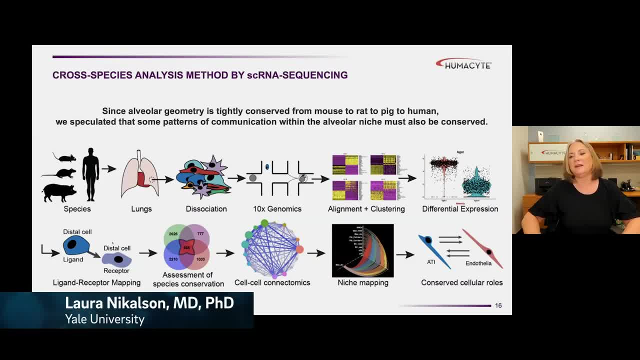 of fibroblasts. So, in order to understand in a very broad way how cells in the alveolus talk to each other, we really wanted to get a signature of lung movement, A signature of what the alveolar communication system looks like. 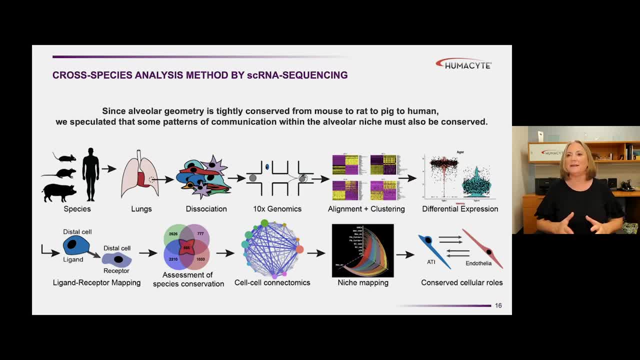 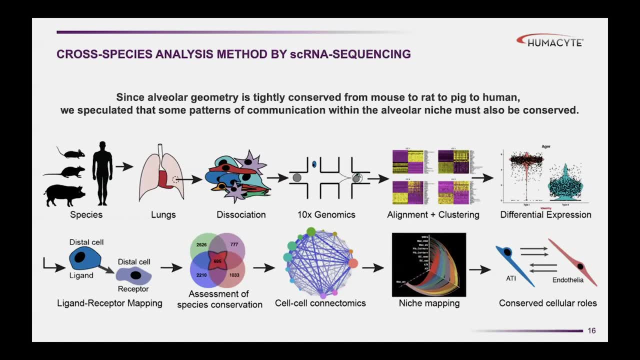 And to do that, what we did is a single-cell analysis of the connectomics between cells in the alveolus, but not just in one species. We actually looked in four species. We looked in mouse, rat, pig and human, because our goal was to not have species-specific. 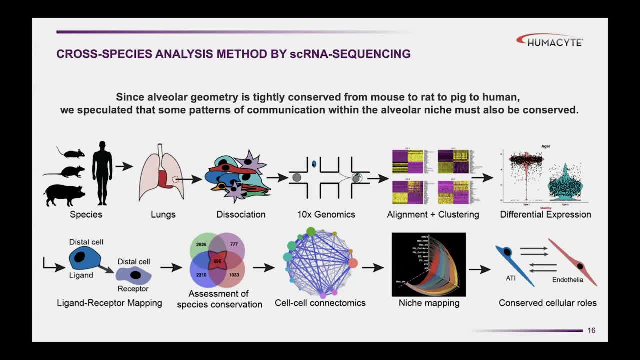 communication algorithms that we were focused on. but really to try to understand, what is it about the alveolus that we're talking about? And so we looked at this collection of six different cell types that creates homeostasis across alveoli, across all of these species. 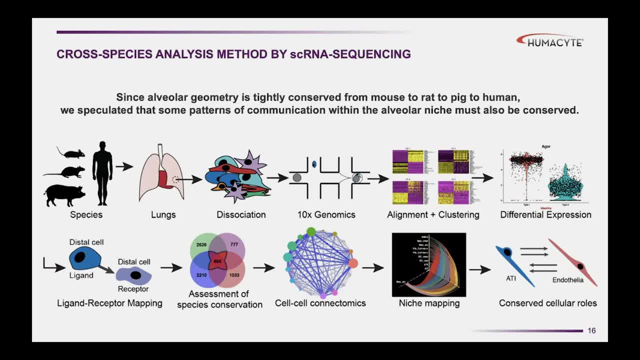 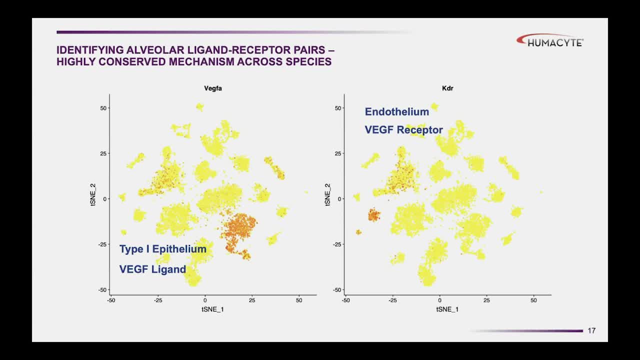 Because, you know, a rat alveolus looks a lot like a human alveolus, And so we speculated that the signaling would also be similar, And this is just one example of one signaling vector that we identified. that's certainly not. 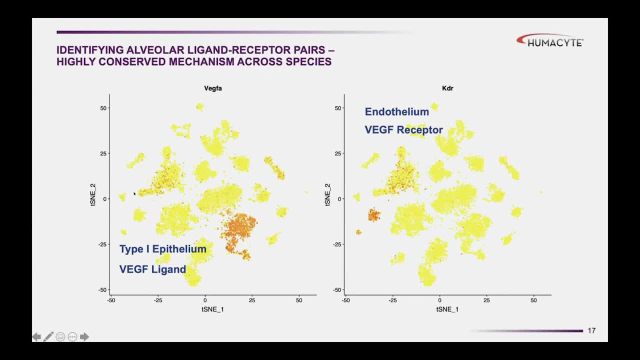 surprising. This is some single-cell data looking at the expression of VEGF alpha And, as you can see, most of the VEGF is actually made by this single cell. Most of the VEGF is actually made by this cell cluster here, which is actually the. 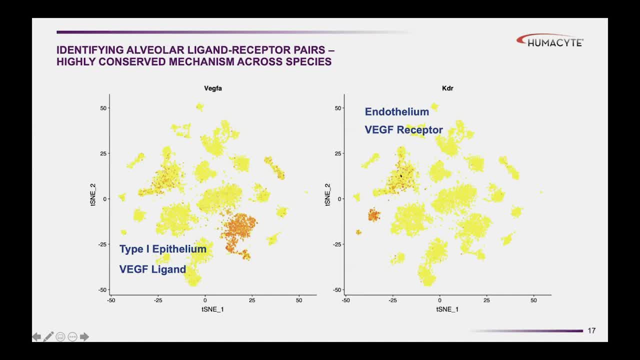 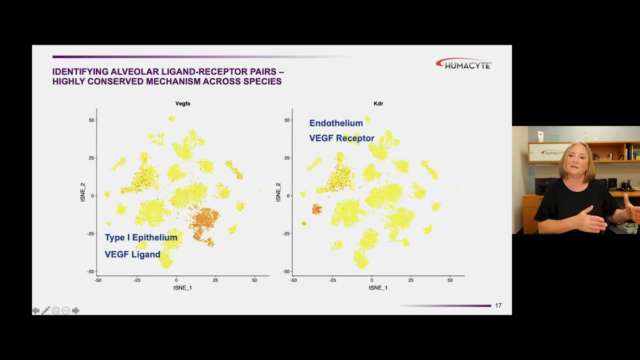 type 1 epithelial cells in the alveoli. Similarly, if you look for the receptor for VEGF, you see that it's located almost entirely on the vascular endothelium, as you would expect. And so by looking at these two sets of data, we can essentially draw a vector, a signaling. 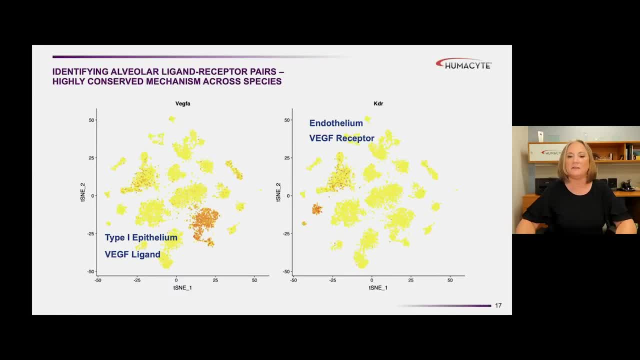 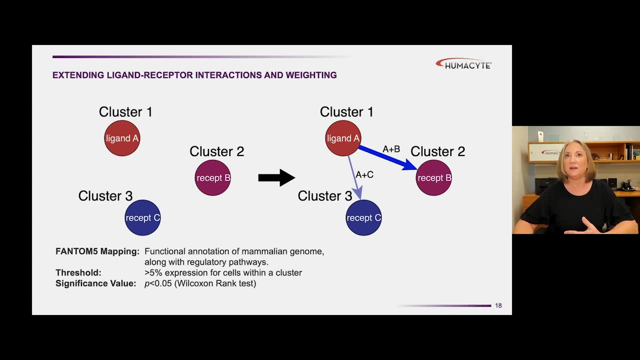 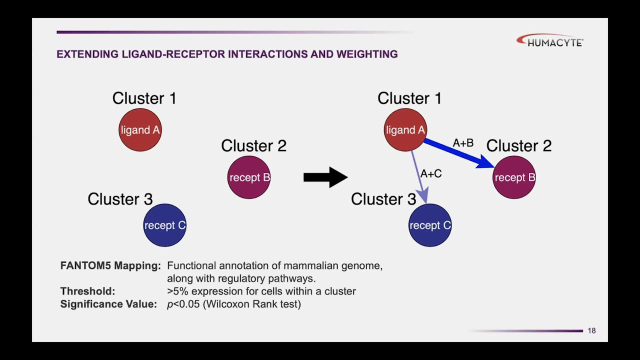 vector that connects the type 1 epithelium to the endothelium in the alveolus. And so we've Another graduate student in my lab. Sam Reardon has done terrific work here looking at how we can generate sort of a connectome or collection of conversations between these different 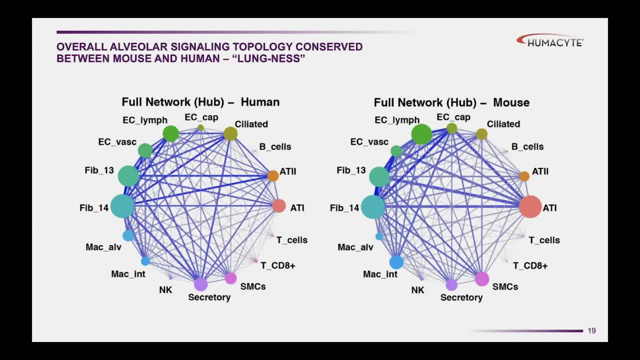 cell types. And what he's shown is that if you look at multiple cell types in the lung- so this is not just the alveolus, but this is cell types even higher up in the airways- it's possible to draw vectors of communication between these different cell types and then to graph the 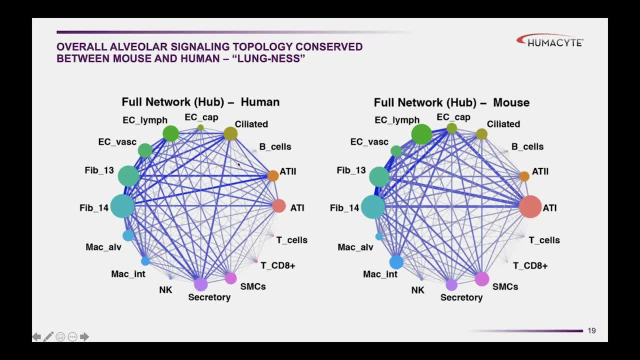 results of that visually And as you can see, the connectomics of cell communication in the human lung is actually at a gross level- bears a lot of similarity to the connectomics in the mouse lung which is shown on the right here. 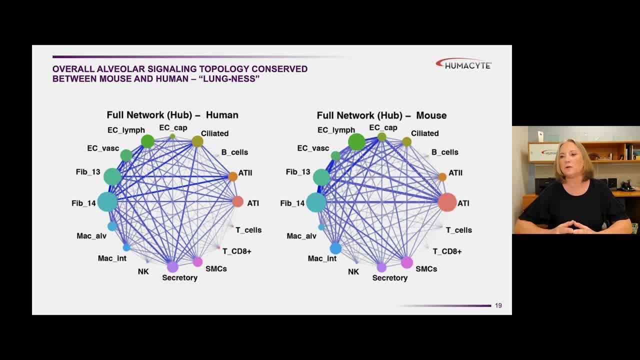 Specifically, the fibroblasts in the alveolus are incredibly important signalers to type 1 and type 2 cells in the alveolus, as well as to other epithelial cells. And that's just one example of a conserved signal. 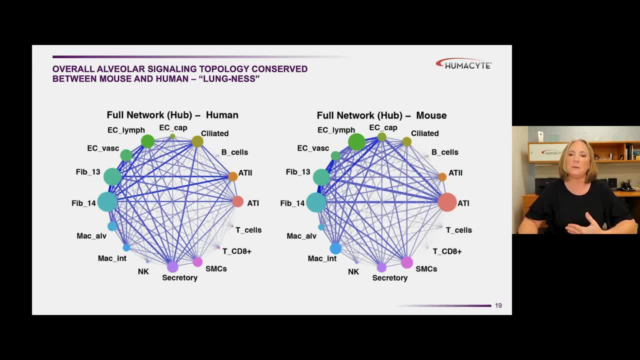 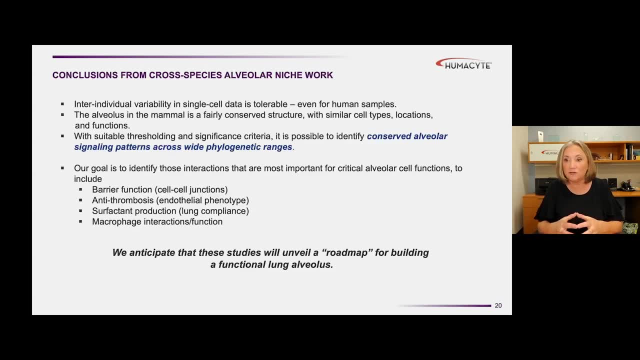 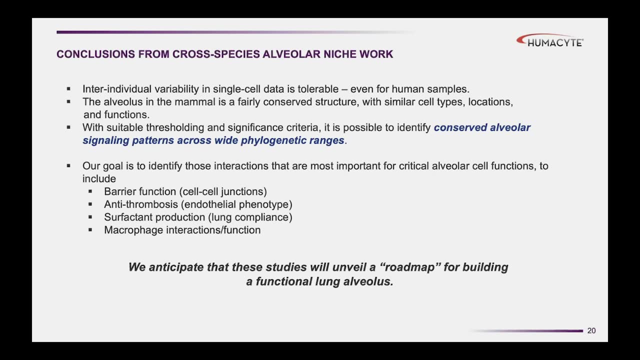 Or conserved signaling pattern. So we do believe that we're making progress in understanding what are the key signals that cells in the alveolus need to talk to each other and to maintain their function and their stability, And we believe that once we're able to tease out this roadmap of communication, we'll be 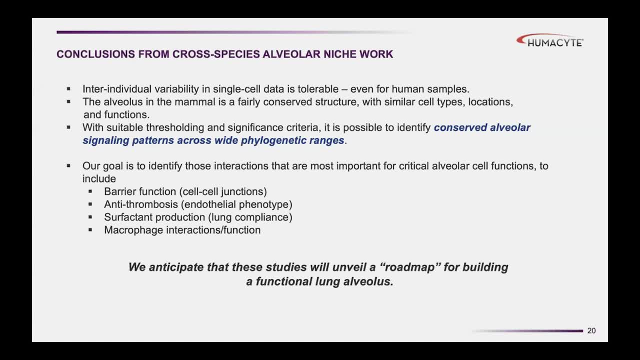 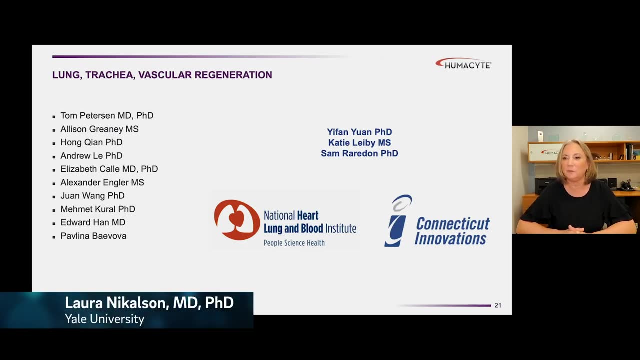 able to translate that into our engineered lung system and really provide the right cues so that we can generate alveoli that are functional, where these five or six different cells types are all behaving as they should. So I'll just finish up there. I really want to thank my fabulous group at Yale who's been working on this problem for a long time. 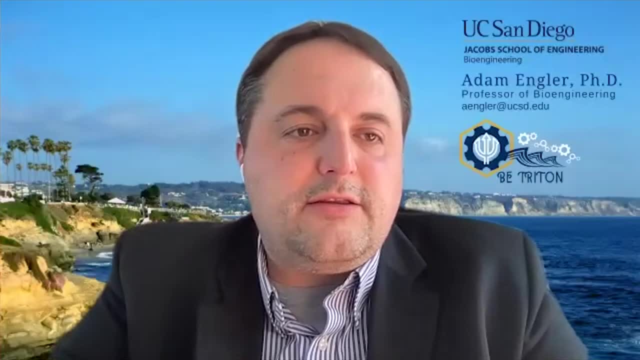 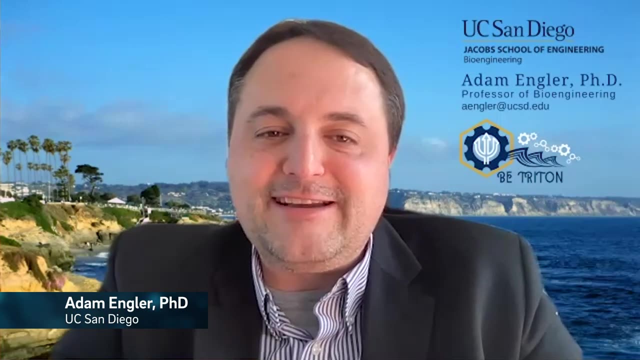 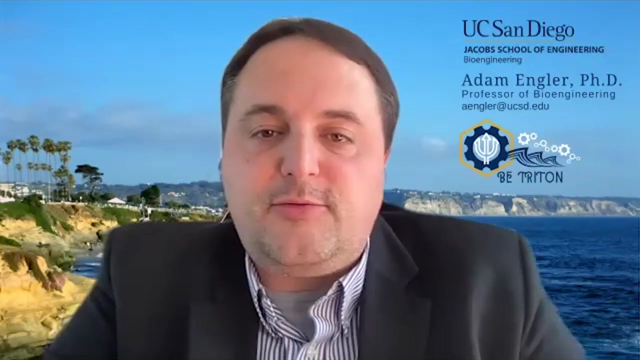 And I'll take any questions at the end of the session. Great, Thank you so very much, Laura. It's greatly appreciated And I'll have to steal that term cell conversation, if you don't mind. So our last speaker joins us from Rice University. 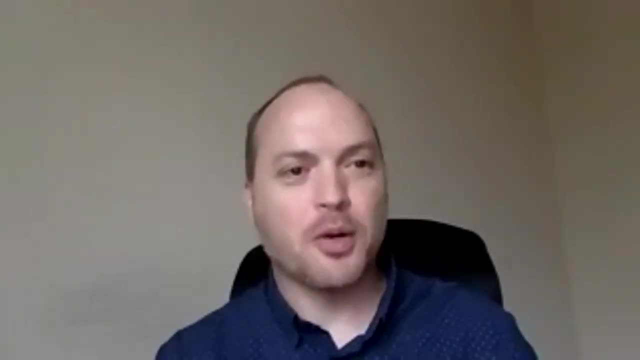 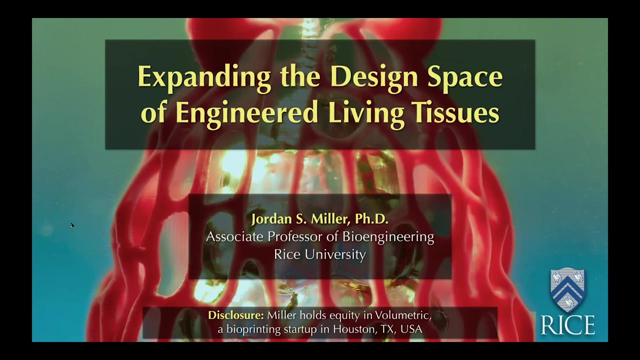 It's my pleasure to introduce Jordan Miller. Thanks Adam, Thanks everyone, It's great to be here And thanks for the invitation. So we're looking at tissue and organ engineering from a bottom-up approach. looking at 3D printing. 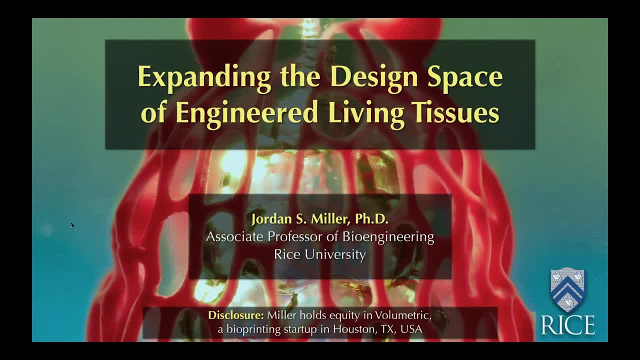 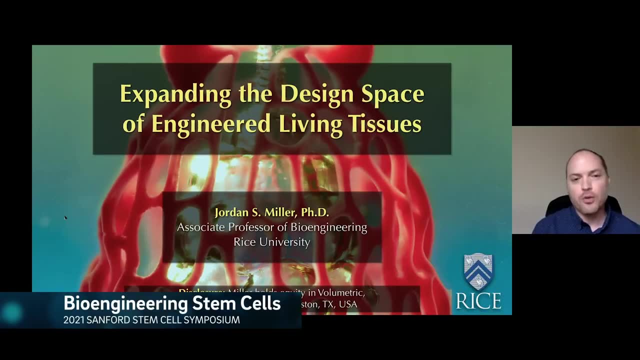 to structure and figuring out that ultra structure. The way that we're looking at this is similar to if you think about the amazing engineering that's in the phones in our pockets now. We started from a very crude single transistor. It was very large. 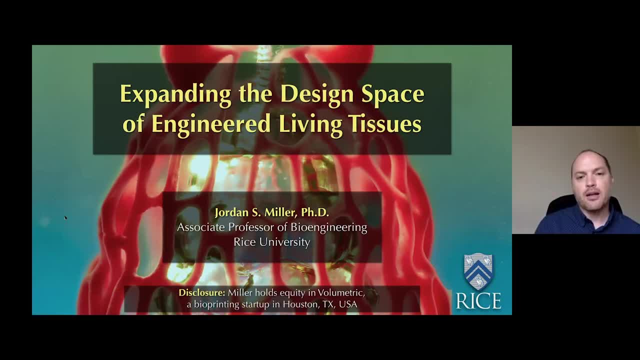 And there was one. It was functional unit of compute And that has scaled through Moore's law, gotten miniaturized and now we have billions of transistors inside of our phones. We have a similar type of challenge that Laura was really explaining clearly where we have. 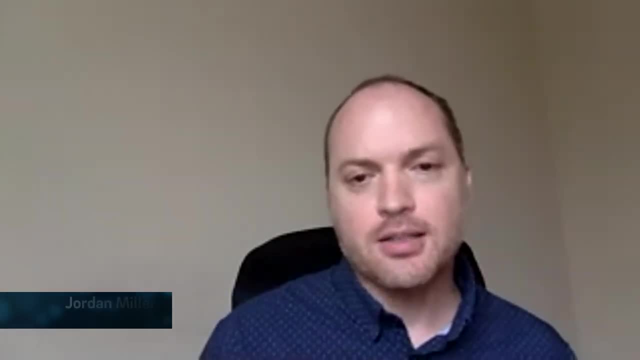 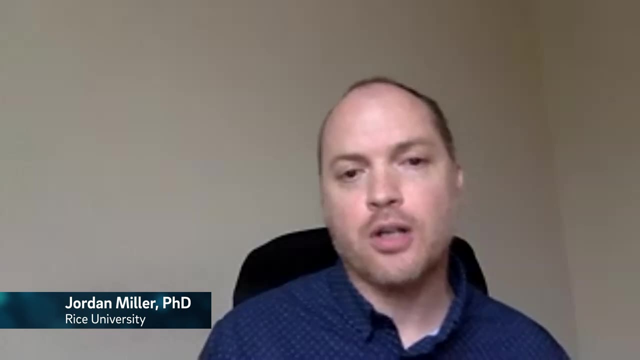 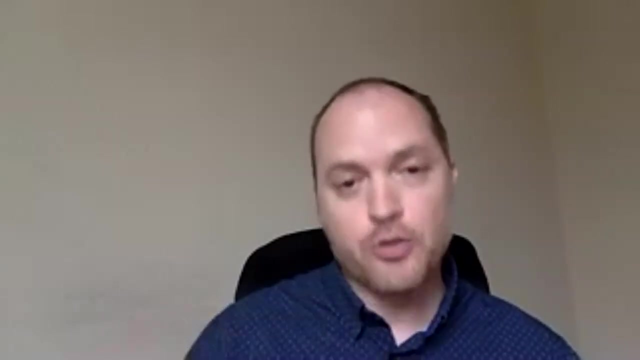 to think about. what is the vascular unit cell inside of our functional organs, organs like the lung and the liver, and the pancreas and the kidneys. They do have similar types of architectural design patterns, where we have a functional vascular unit cell And it's replicated and scaled up hundreds of millions of times in our organs. 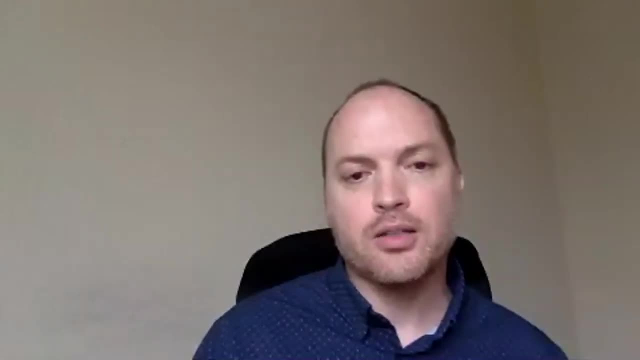 And so we're asking the question of how can we design such unit cells from scratch? And then we have a lot of work to do to miniaturize them and replicate them hundreds of millions of times. So generally, this idea is centered in oh and sorry. as a disclosure, we have a startup. 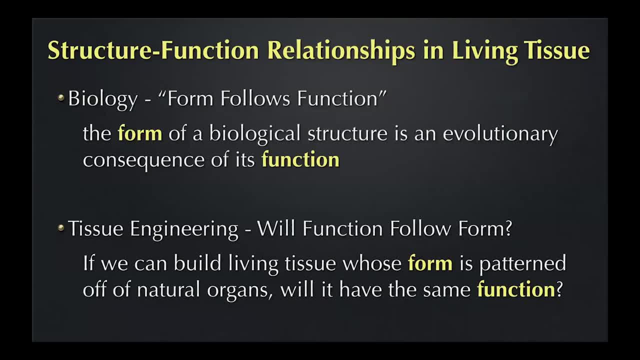 company, Volumetric, that is commercializing this technology. So we're really focusing on the structure, function relationships and living tissue. And in biology we have this idea: Form follows function, where the form of a biological structure could be anything from. 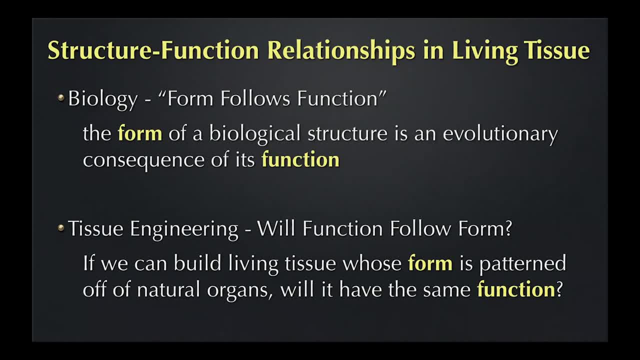 a single protein structure all the way to the limb of an organism or the organism itself. It's really an evolutionary consequence of its function And in tissue engineering we're really asking the converse question: will function follow form? If we can make the structure that replicates what we see in the body, how much of that? 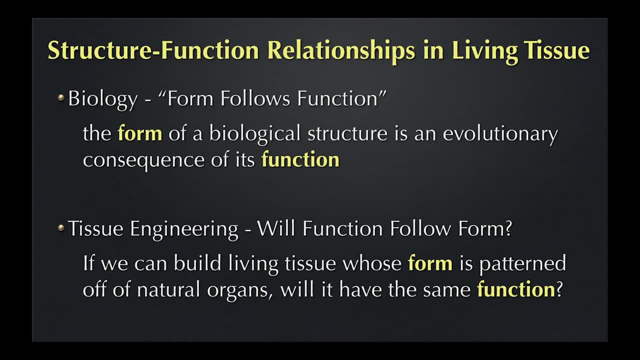 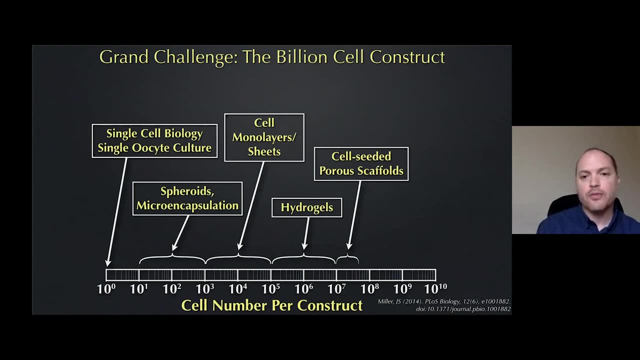 do we need to replicate? using a very reductionist perspective, Could we build up structures from scratch that begin to replicate, And then we're going to mimic some of these functions, And would that be sufficient to help human patients? So one of the challenges that we think about a lot is: how are we going to get enough cells? 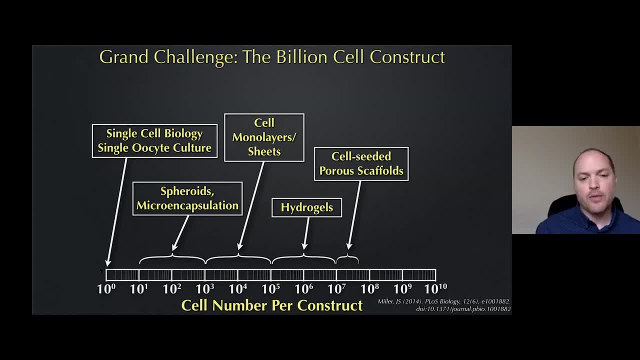 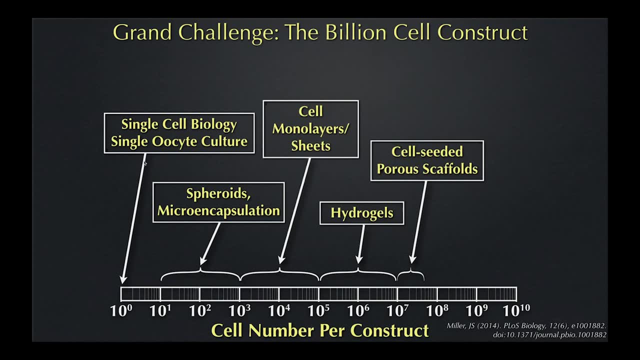 And a lot of us are in this regime. So I have here an exponential graph along the bottom: 10 to the 0,, so cell number per construct. 10 to the 0, single cell biology way over here. A lot of our lab's work is here. 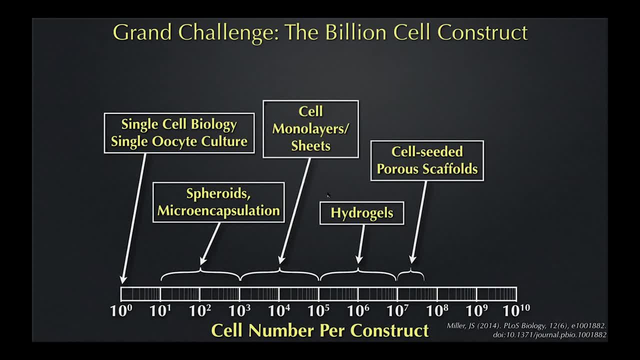 And we really need to be thinking about the organ scale. We have hundreds of billions of cells. We have hundreds of billions of cells in our organs, And so we need at least 1 to 10 billion cells in organ scaffolds to begin to replicate some. 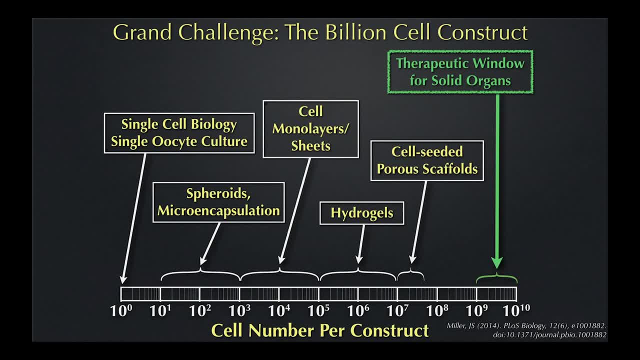 of that biochemical function that is, an additive sum of all of the cells and all of their efforts inside of a effectively portable volume that fits inside of our body. If I make an organ that is 10% as efficient as the liver, it has to be 10 times bigger. 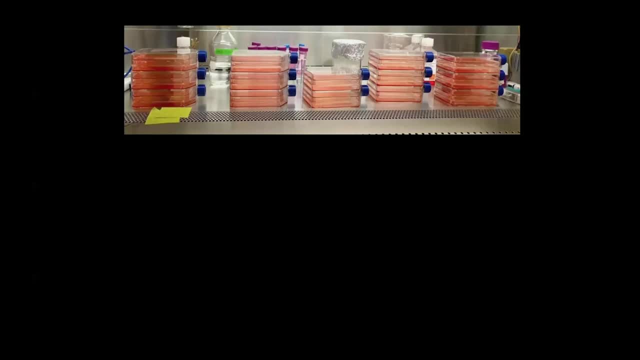 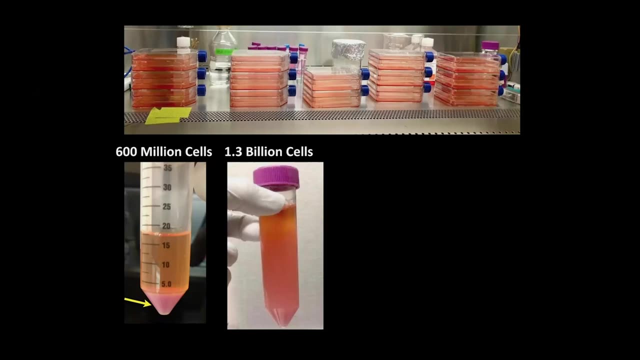 And that's not going to fit inside of your torso. So we can grow billions of cells And a lot of you are growing a lot more cells than we do. This is what a billion cells looks like in a single 50-mil conical. 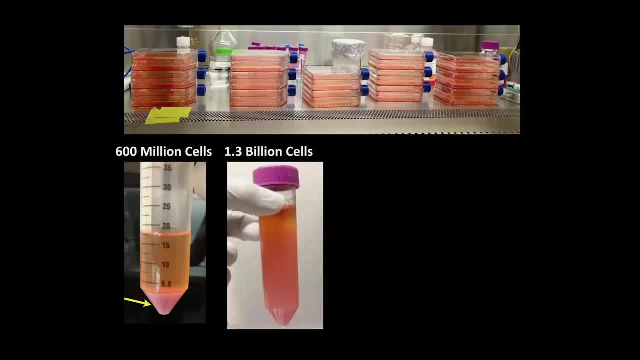 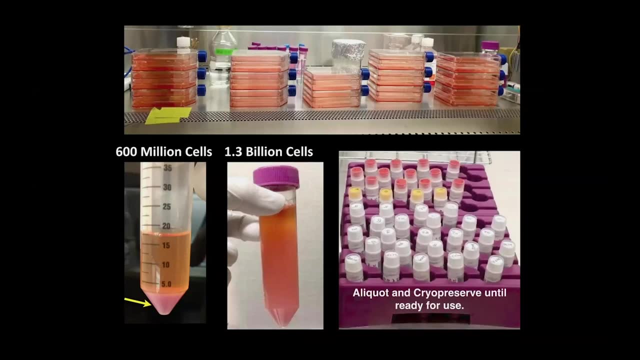 But when we're talking about adherent cells and a lot of the parenchymal cells we're interested in, we are not able to keep these alive for very long. As soon as we trypsinize them, we're starting a clock to cell death. 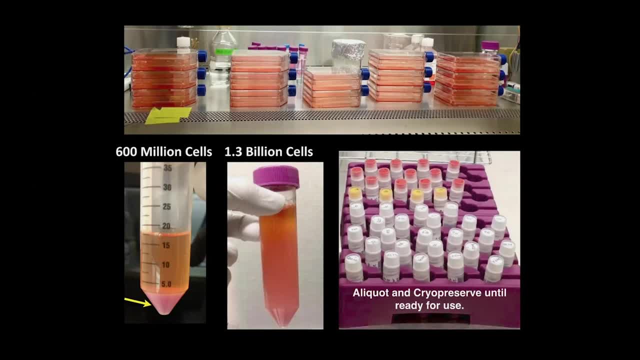 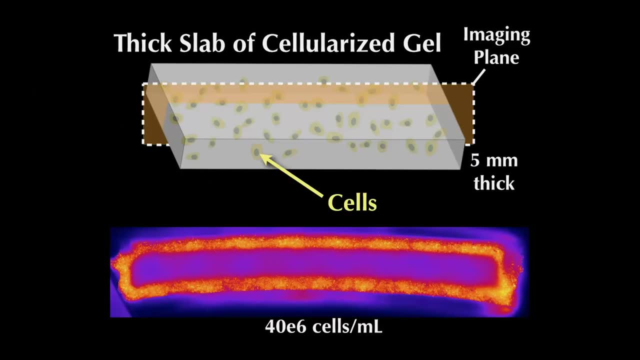 And instead we have to just aliquot the cells down, freeze them down and try to use them when we can. So if you take these cells, what if you just stick them in a gel? So this is really a lot of the early work in the field where you would do an experiment. 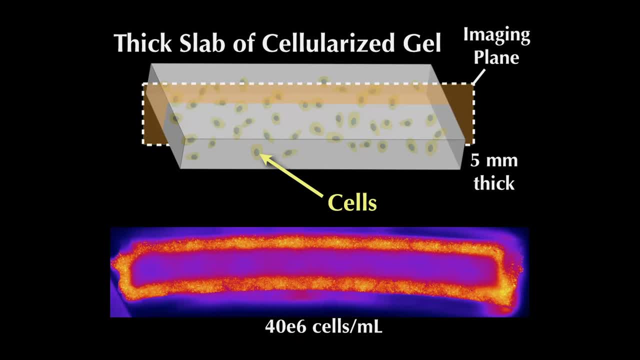 like this. This is our take on it. So you have a thick slab of gel. thick from a cell's perspective, 5 millimeters, very thin from a human perspective, But we can load it up with tons of cells: 40 million cells per ml. 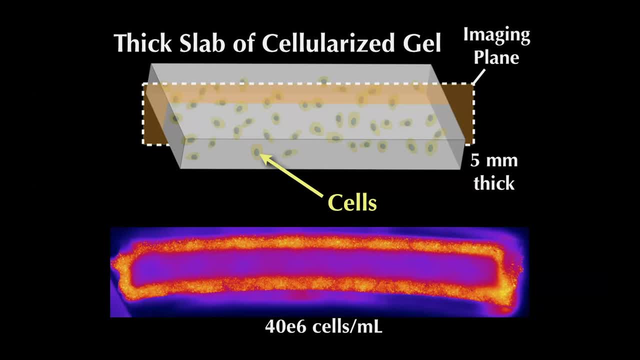 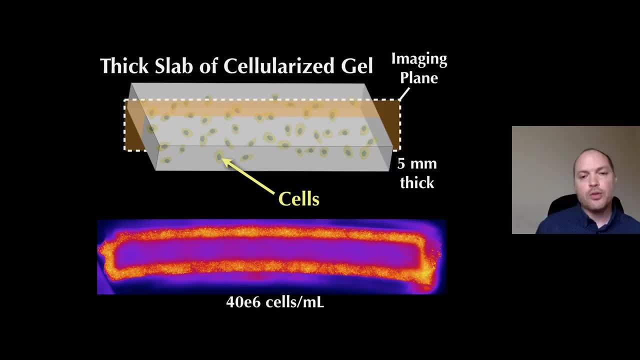 These are HEK cells that are expressing a destabilized EGFP And if you grow this for a couple of days, you take a cross-section through it. This is false color for the destabilized EGFP. You see that you get a crust-like gel. 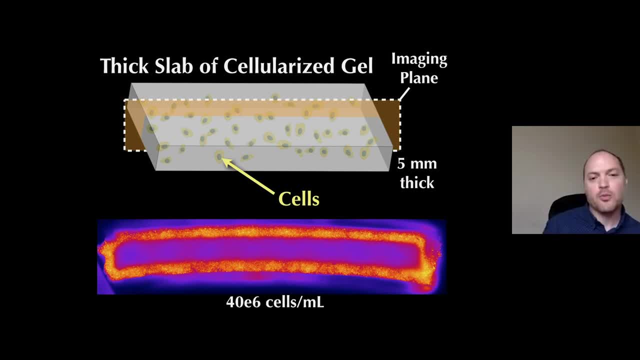 This is a layer of cell survival. It looks like a slice of bread where you have the outer surface. That is where oxygenation is happening when you're making bread. That's where oxygenation is happening in our tissues when we're making these thick. 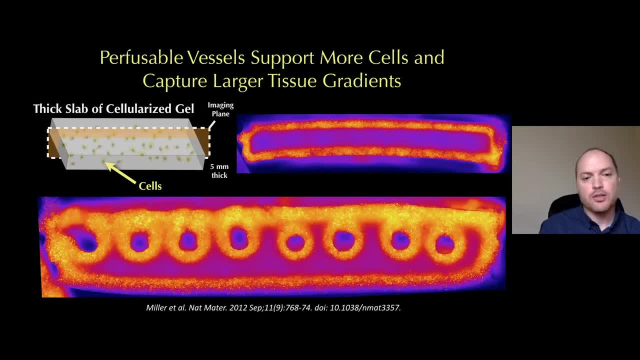 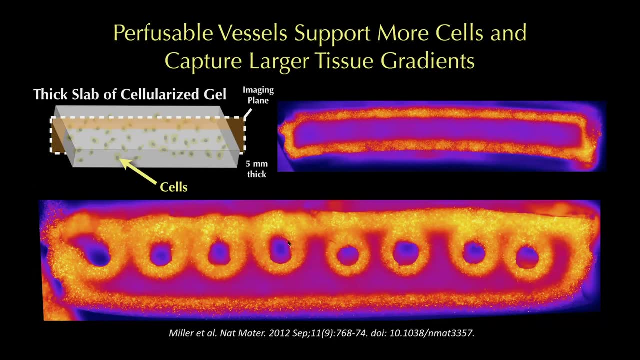 slabs. So we showed that if you have just very simple channels inside of these gels, you can get flow through them. And when you have that flow, each individual vessel- here we're looking at 800 micron vessels inside of these tissue slabs- they are able to keep a circumferential volume. 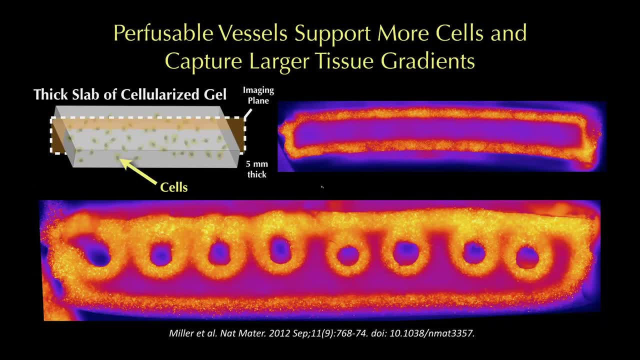 of cells alive, in contrast to tissues that don't have any vessels. But you see, it's not a perfect job here. We have lots of dead zones still in the tissue that we needed to optimize If we looked at this further more recently. this is the work of Ian Kinzinger in our group. 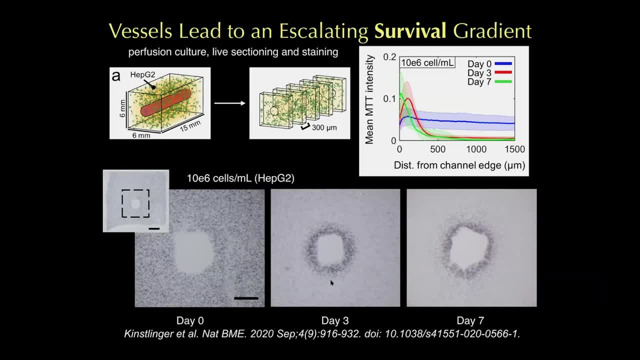 who just went on to start his postdoc in Boston And he has been looking at HEPG2 cells. We can talk about the value of HEPG2 cells in tissue screening. The point is that they're mammalian cells that are highly metabolically active. 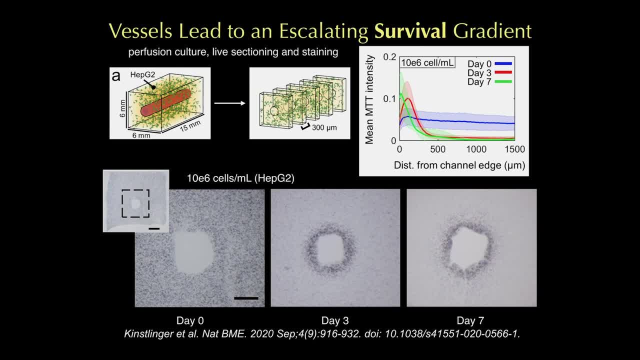 We were able to quantify that these vessels in highly proliferative cells were getting escalating gradients of survival. You can see here, with the MTT staining and escalating proliferation gradients that you're seeing here, that tend to follow each other And we think these are non-degradable gels. 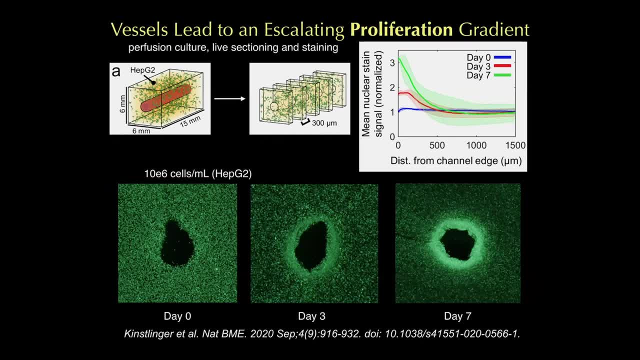 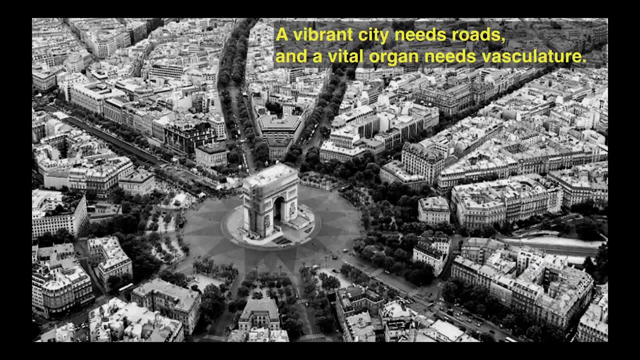 In this case, we think the cells are proliferating closer to the vessel and dying further away. So the reason this happens is the same reason And the same thought process that goes into the design of cities. actually. So, just as a vibrant city needs roads, a vital organ has to have vasculature. 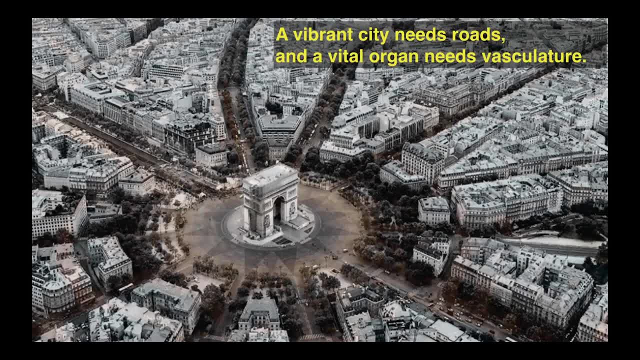 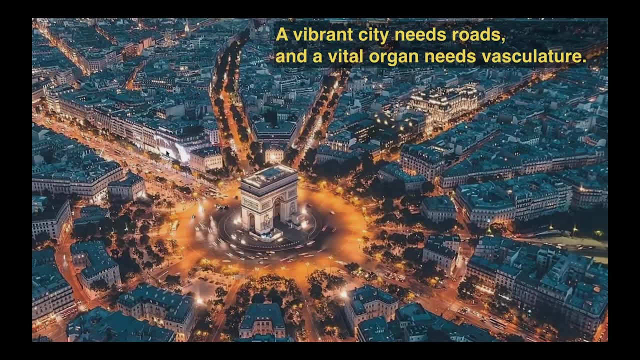 So with a city, we have certain city blocks where the residents live. So here's a great picture of Paris And in our tissues we have the areas where our cells are residing. They're in place, They're trapped inside the solid. 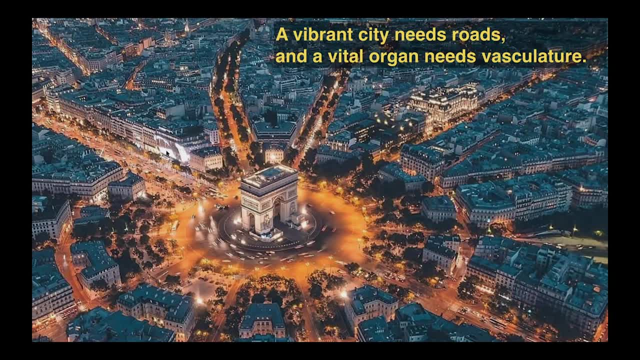 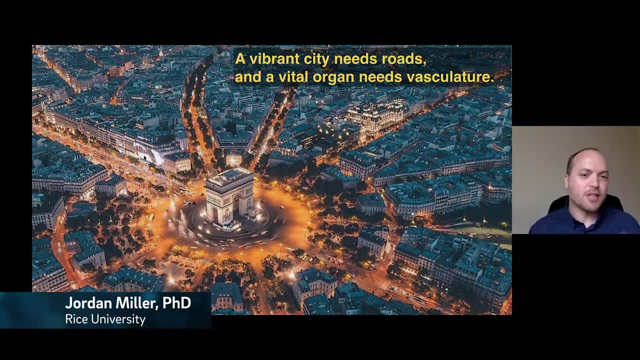 And we have to have these highways. If you imagine a city that didn't have roads, how would you get your furniture home? How would you get groceries home? How would you take out the trash? This is exactly the same challenge that our cells have to do at a micron scale. 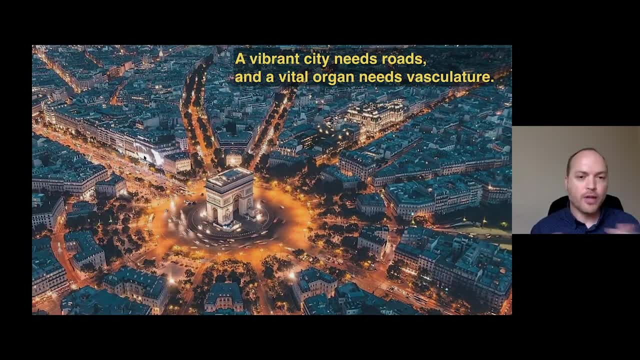 And if we don't provide the highways for that nutrient and waste transport, it's not going to be a very efficient tissue and the cells are going to die very rapidly. We have to think about this. the total organ scale In our liver? it's the same story. 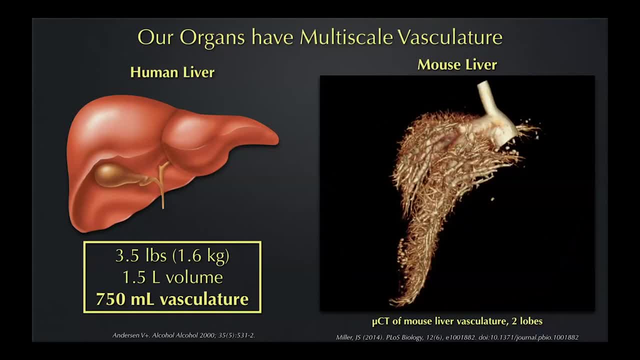 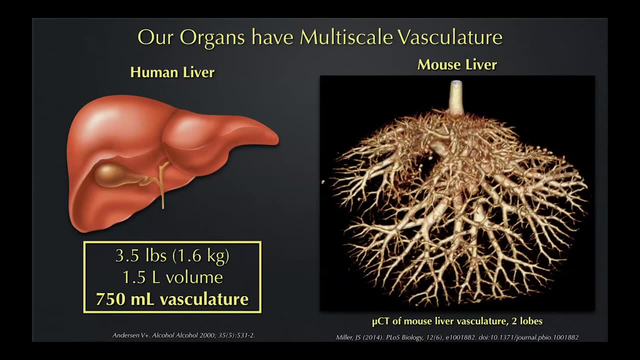 A very large organ. over half of the volume of the liver is liquid. The concept of solid organ is actually a misnomer, right If our large volumetric organs are more than half liquid, with perfusion volumes. that includes the blood vessels, includes the lymphatics and includes things like the bile duct tree. 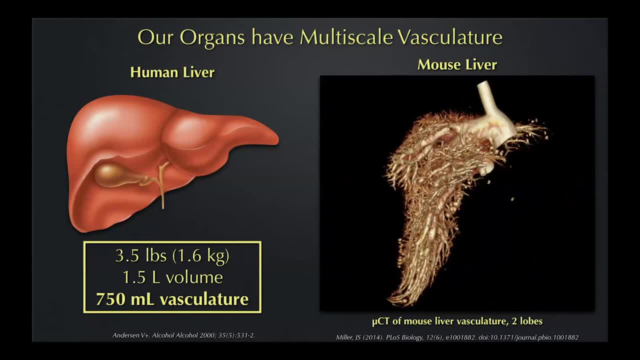 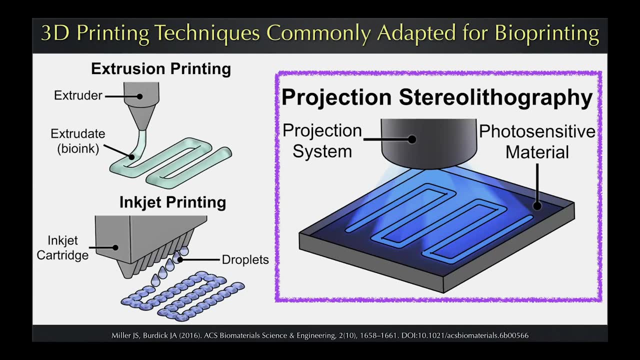 in the liver, the urinary tree and the kidneys. So we used- in this case we're using- projection stereolithography. So it's adapting techniques from the 3D printing industry that have been around for almost 40 years now- a lot of these ideas- and adapting them into biology and biomaterials that we 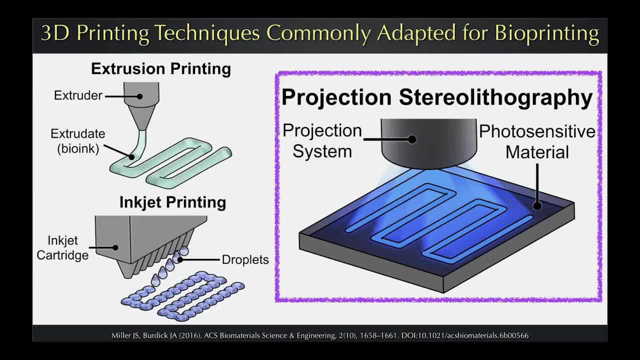 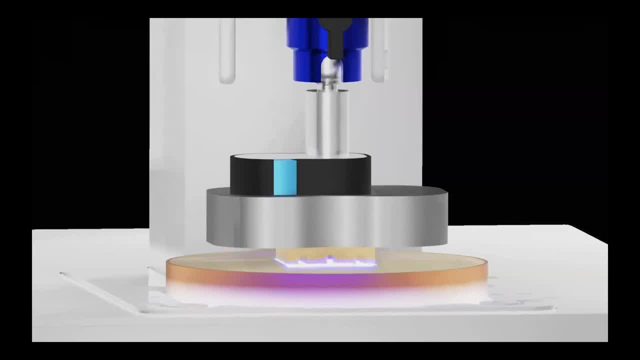 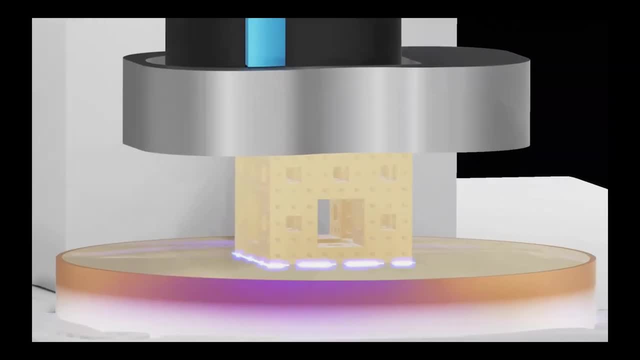 can structure the material And then interrogate in a very reproducible way: how functional is that architecture? So we're using layer by layer projection where a light sensitive polyethylene glycol diacrylate gel is being polymerized. We can also do this with gelatin, with acrylate, in degradable settings. 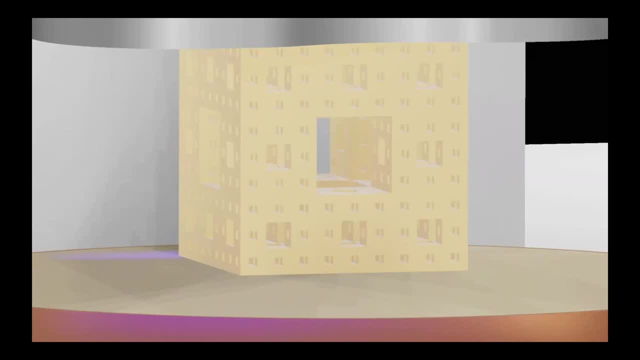 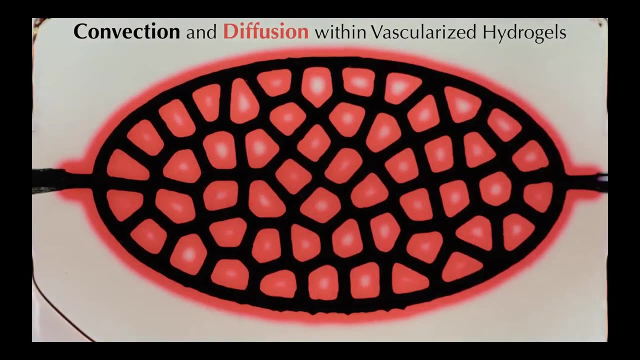 Every individual layer is a different image getting projected and effectively building up the object. So what we like about using 3D printed hydrogels: you can make really intricate blood vessels networks. You can see here: Here we're perfusing in two different materials. 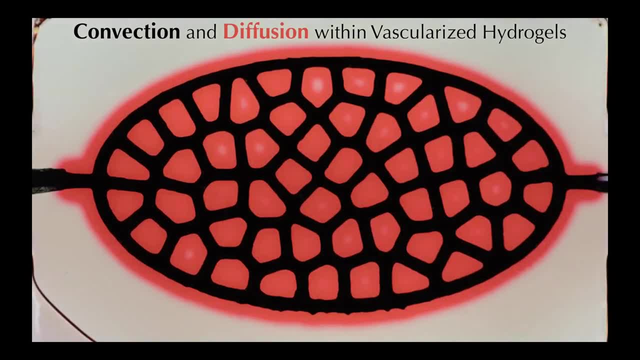 We have colloidal black ink- India ink- going in. It gets trapped and stays inside of the vessels. We're also perfusing in red food coloring, a small hydrophilic dye that diffuses out And you can see it looks like this. Voronoi architecture resembles what you might see. 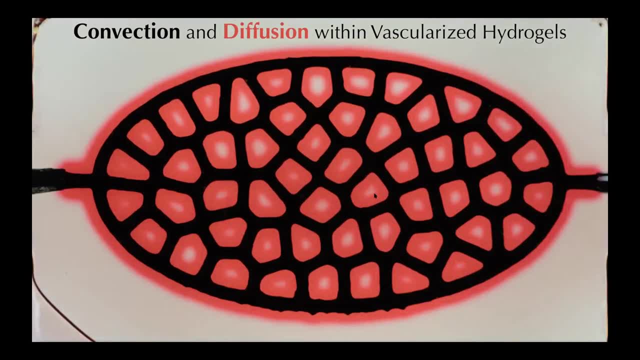 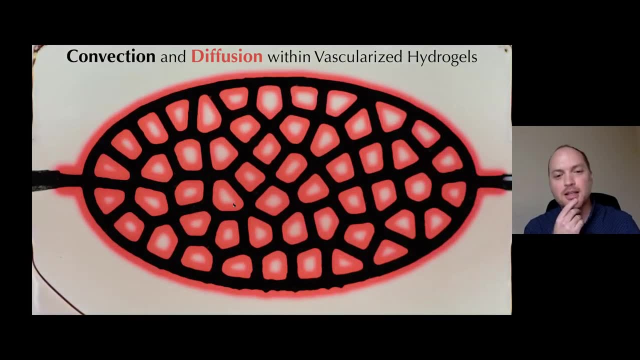 in a city block diagram. This would be a hard city to drive through. Maybe this feels more like I'm remembering my times in Boston. And so you have these individual city blocks. We're going to have the cell residents live And we need to see how fast can we deliver nutrients and oxygen to the cells that we 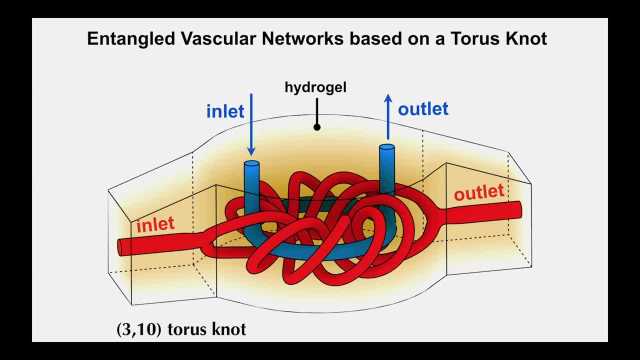 trap there. We needed to go more complicated. So we began to build up different architectural concepts and explore these new design freedoms in tissues based on this technique. So here's a torus knot. It actually is reminiscent to me of the glomerulus in the kidney. 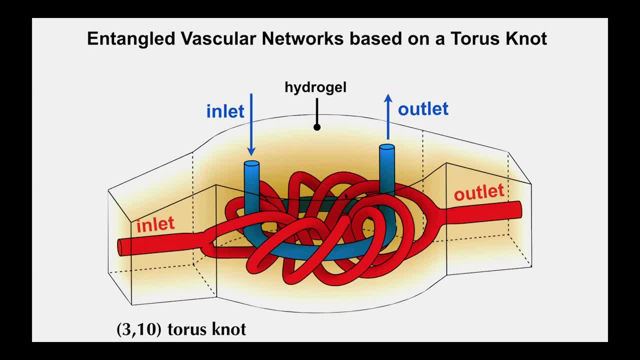 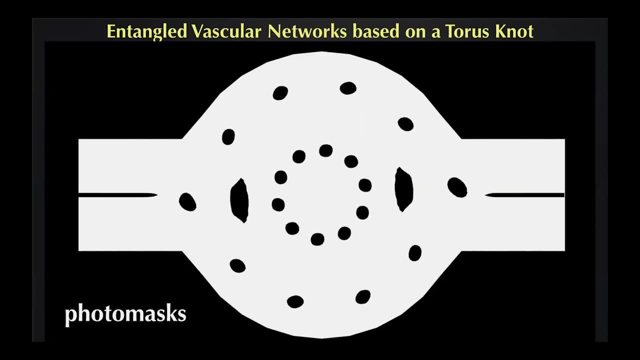 Here we can do an inlet outlet, which is the torus, And the torus knot is the red topology that sits on the surface of the torus. You can see what the Individual photo mass would look like to build that object up and how that would then build. 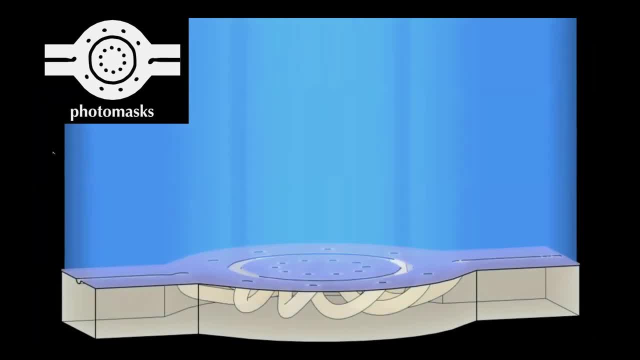 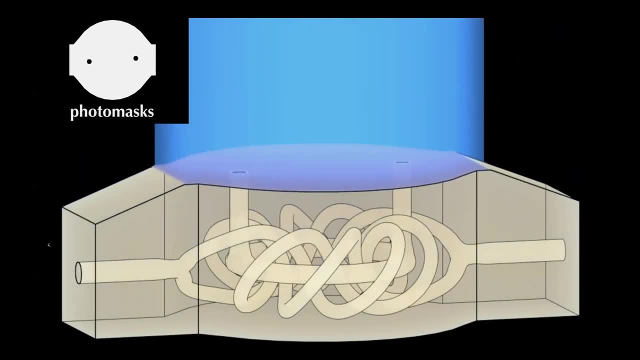 up to make the object. So the photo mass in the upper left up here, And we're building up the object one layer at a time. We have now two independent vessel networks with branches inside of the same tissue architectures to this hydrogel material. 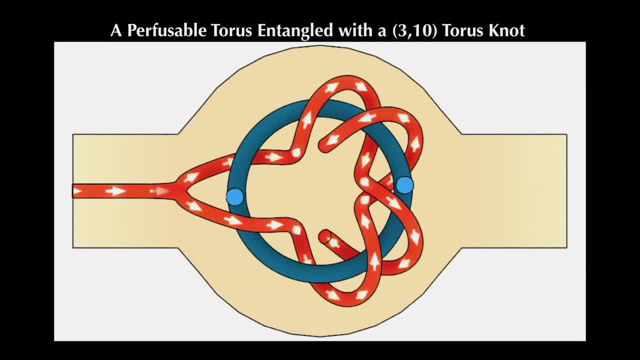 This is what it would look like if we could get the flow to work, And in fact, we were able to get the flow to work inside of the vessel. Now, this is again not at the scale we would like to do to make organs. 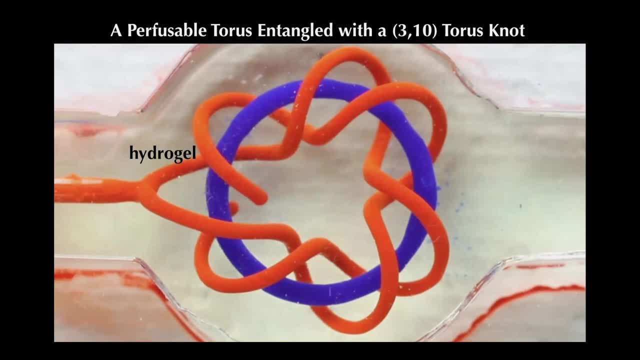 These vessels in this case are around 500 microns in diameter. We'll talk about getting to smaller diameter vessels, But this was exciting to us because it represented the ability to do multivascular architecture: two or more independent vessel networks inside of one gel. 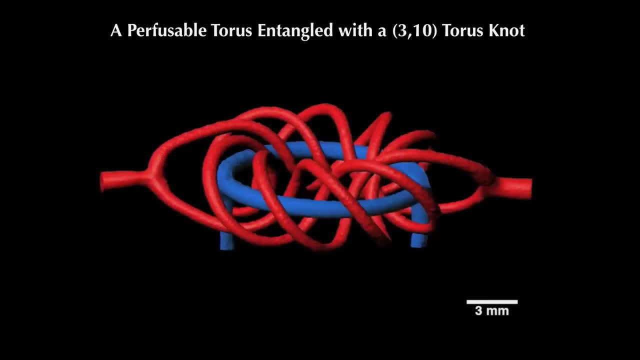 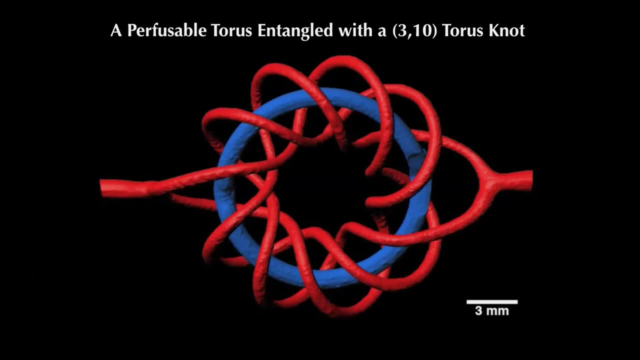 We can put different materials in use, one for in, one for out. Lots of different ways to think about this. Now, this was exciting to us, but this is not what our organs look like. Our organs look like this, Right. 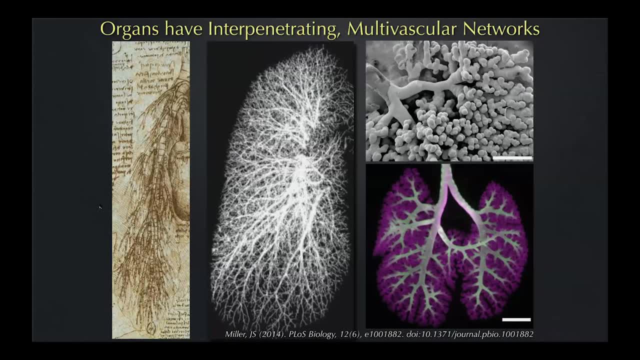 And you may notice or recognize the artist on the left here. This is from Leonardo da Vinci, Over 500 years ago, where he was really noticing this multibranching architecture. So we have the heart here. We have the blood vessels from the heart going down into the lung. 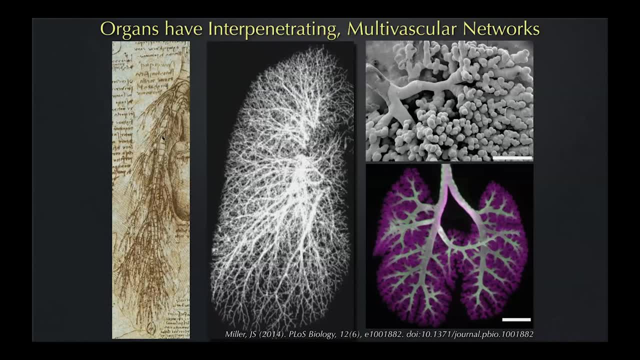 But you can also see another interpenetrating, multiscale architecture: the ribs of cartilage of the trachea going down also And, as far as Leonardo da Vinci could see, down into the bottom of the lung and the distal components. 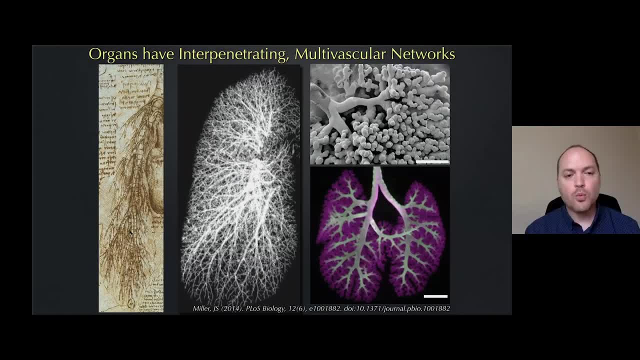 he continued to see the branching go all the way down. We still have a limited ability to understand the total architecture, but we can do a CAT scan of the whole vasculature of the lung. You can see just the vasculature here, not the airways. 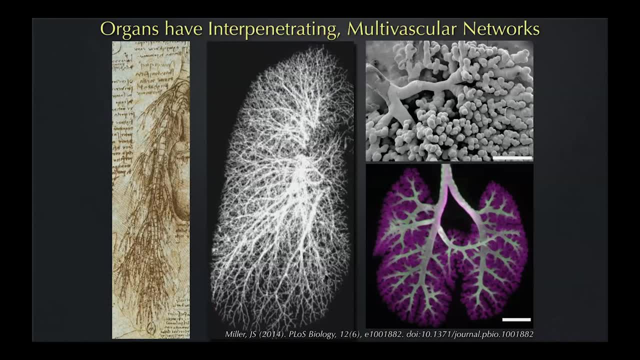 And you can see the capillaries, because the CAT scan doesn't have that kind of resolution. This upper right image- this is actually a beautiful photo from Laura Nicholson's lab. Thank you, Laura. This is resin casting of the airway of the lung. 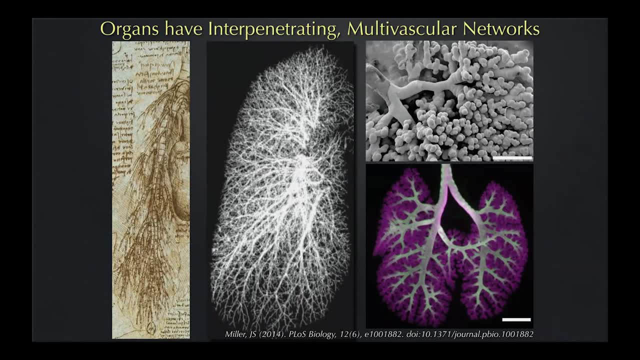 And you can see the beautiful, amazing architecture of the alveolar air sacs all the way at the bottom here. But then this resin casting technique. you know you can't see the vasculature too, because we're really looking at the resin getting into the airway to cast it. 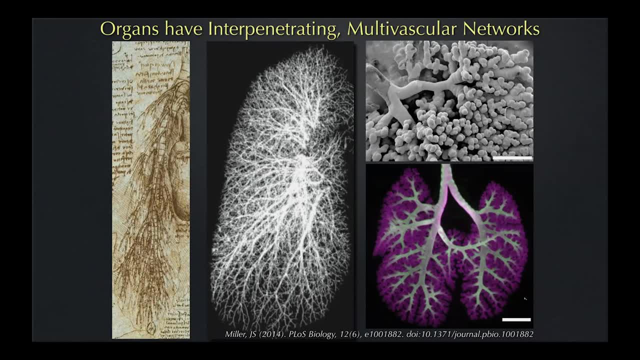 And then other groups. so this is work from Jichao Chen's group, where he's looking at the developmental biology of the lung from scratch and looking at that architectural development. So we were taking inspiration here, thinking, you know, we can't make a lung yet. 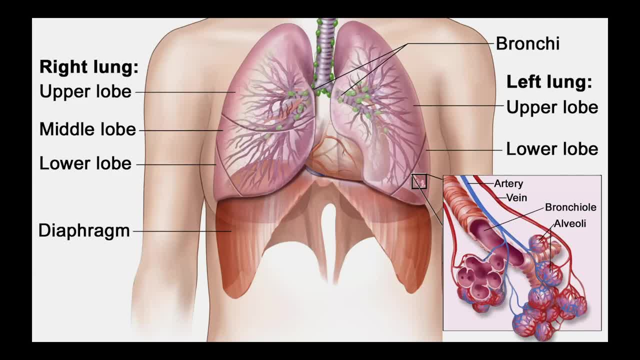 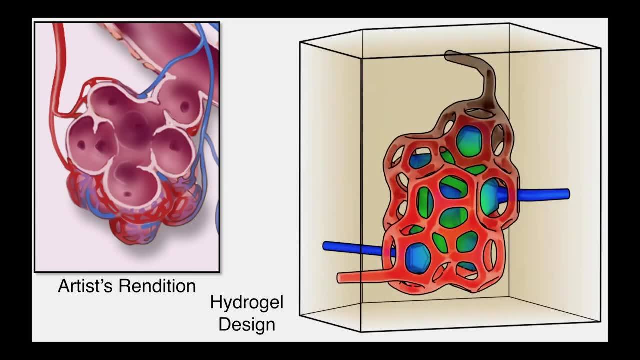 So we're trying to think about what is that vascular unit cell? Can we design it on the computer? Can we build it up? And we were able to do that inside of the gel. So you can see, here we're inflating the air sac. 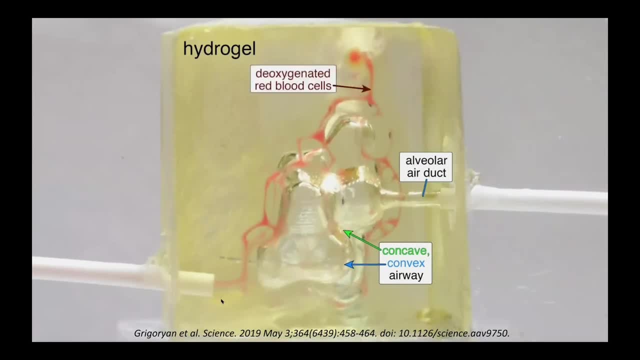 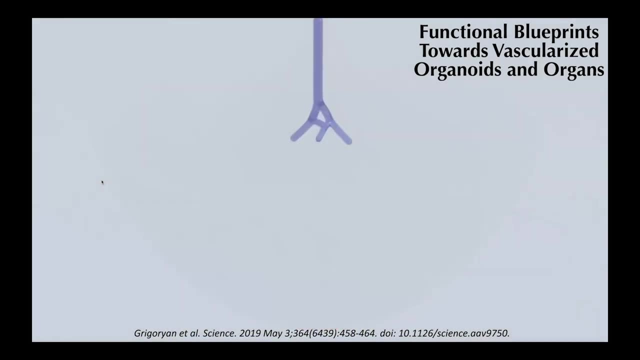 We're getting deoxygenated red blood cells coming in and then sheathing vascular architecture. They're picking up oxygen coming out And we were able to further show some design paradigms we think could be useful where you would first computationally grow the airway. 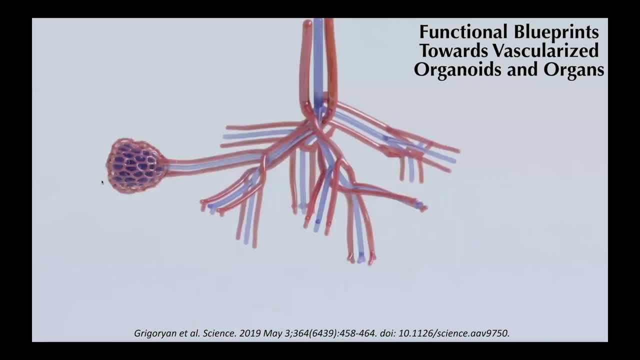 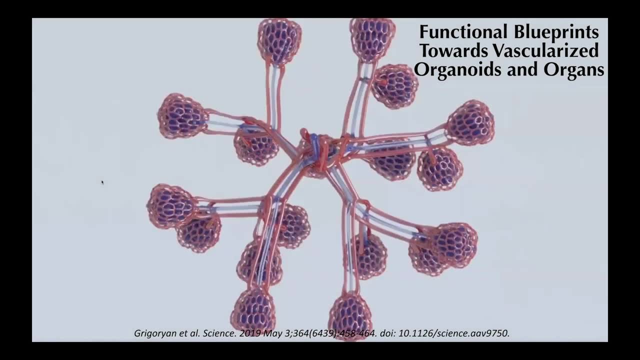 This is in collaboration with Nervous System, a design firm in New York, And then populate the tips of these branches with these alveolar air sacs- And we can't yet scale this up right. So we're trying to build this up further. 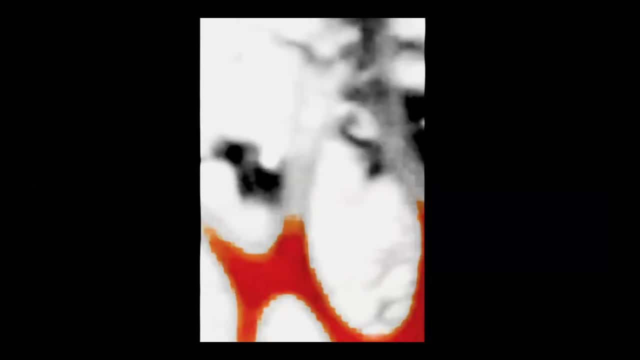 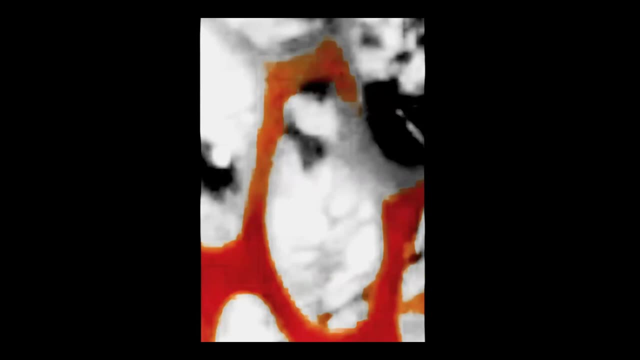 But this was our version, that we were able to show that some of that architectural complexity would impinge on the vessels in different ways based on the local curvature of the airway. So this is strictly topology And there's not any cells in the bulk of the matrix. 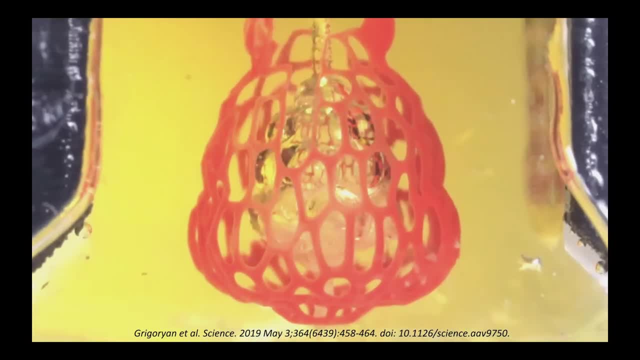 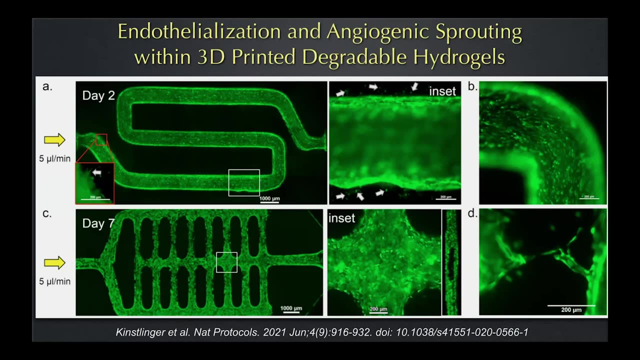 Those are human red blood cells we're perfusing through. But what about cellularizing these tissues? So we have been looking at more recently how we're going to be endothelializing these vessel architectures. You can see here just published recently. 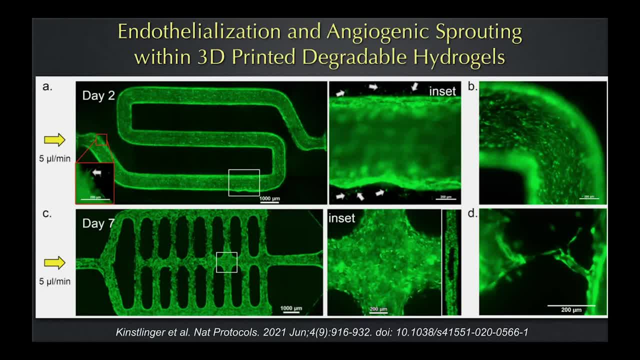 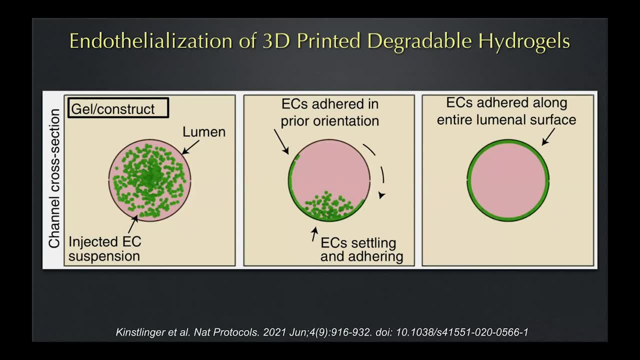 where we're injecting endothelial cells in. We actually did a detailed protocol of how this works. We're injecting cells in, We're rotating the tissue around. How do you rotate a tissue around if it's in a multi-walled plate? Well, you're going to need, actually, these 3D printed chambers that we also built and open sourced. 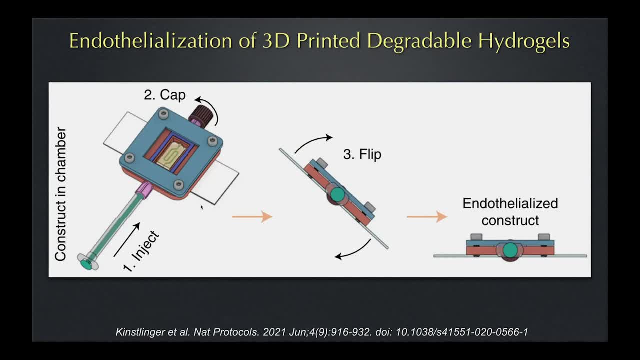 You can download off of the Nature Protocols website or off of our GitHub repository, And we have a whole set of protocols for how to both 3D print the gel and 3D print the chambers, all the parts to do this And even the machine that you can build. download, 3D print the parts. 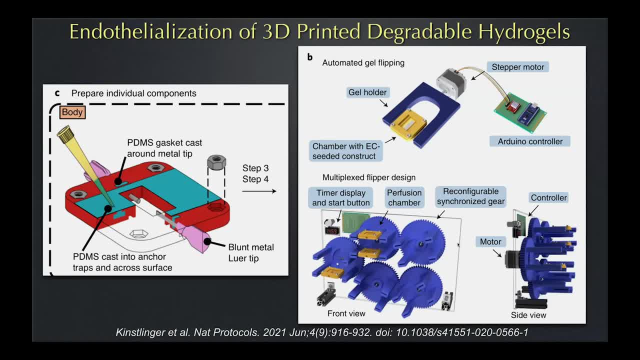 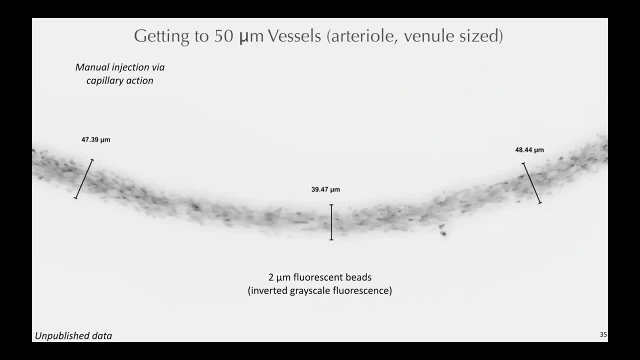 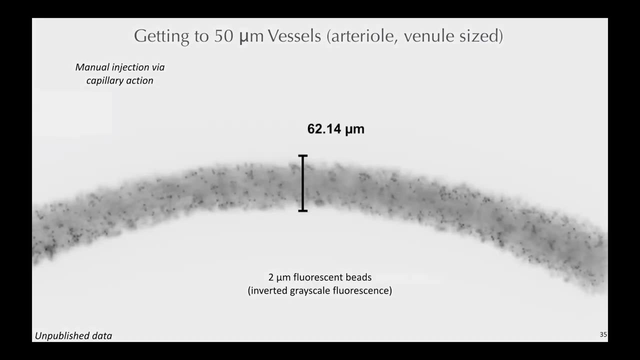 and it will auto-rotate your gels for you. So this has been really exciting for us and very useful for all of our individual seeding steps. So more recently we've been looking at going higher resolution. We've now been able to get you know: initially we had the 300 micron vessels in the alveolar air sac. 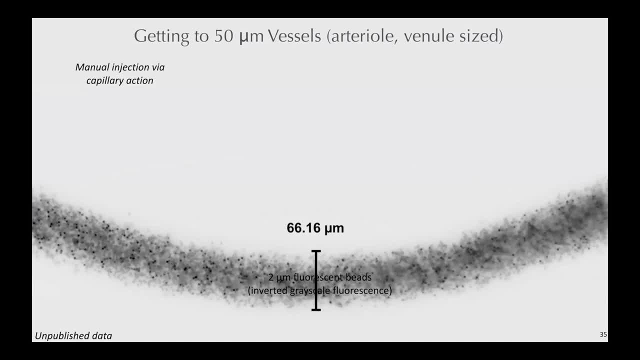 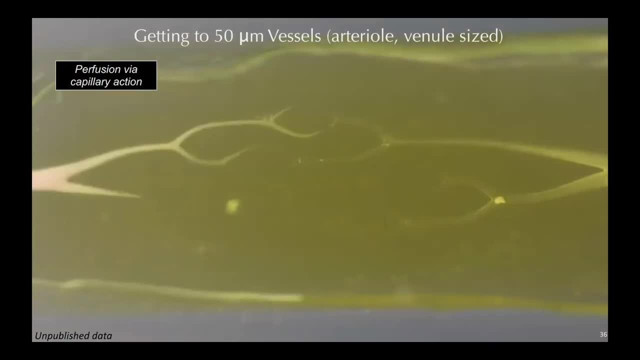 Now we're getting down to sub-100 micron, in some cases around 50 micron Vessel diameter. We're able to also get good perfusion through there, as you can see here. Here these can get perfused strictly by capillary action. but obviously we're going to grow human cells. 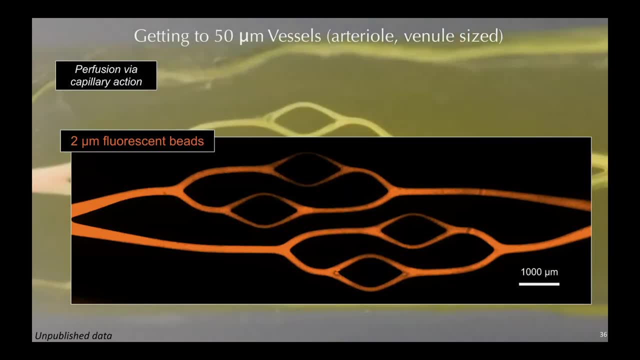 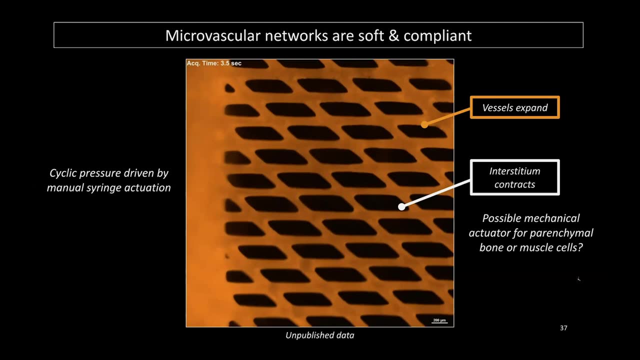 We want to do this in a more pumping perfusion way, So we've been looking into that as well. You can see these gels maintain their elasticity. We're looking at what is the optimal balance between vascular architecture and interstitial zones. If you have too much vasculature. 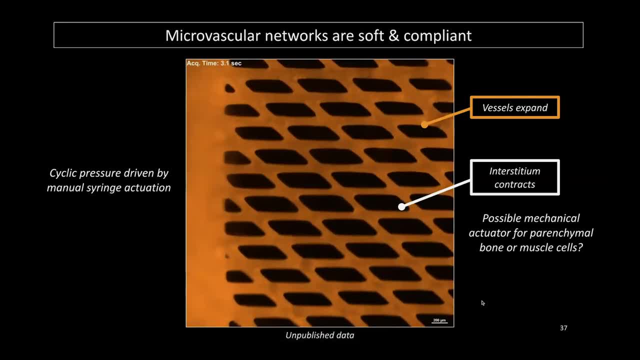 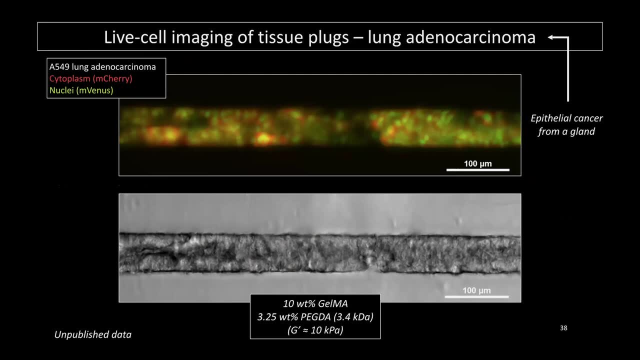 it's going to look like something like rosacea or something where way too many vessels not enough room for tissue function. We've also been able to now endothelialize vessels. So sorry, before I get to that, given some of the talks about cancer. 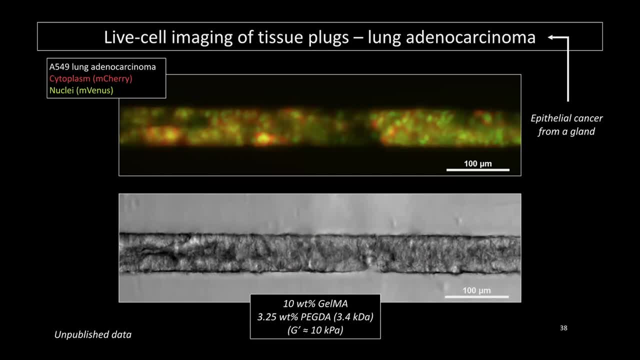 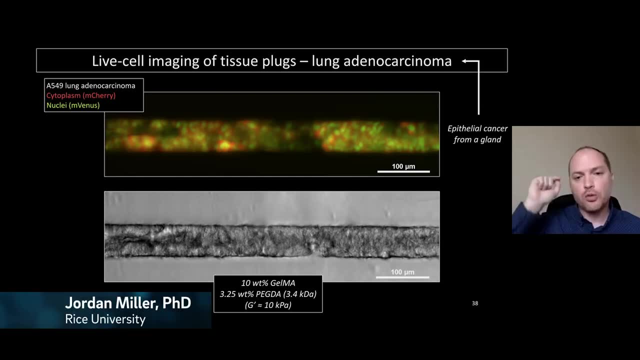 we're also looking at. you know, just because you have a vascular channel doesn't mean you have to do flow perfusion through there. You might think about structuring multivascular architecture: One of the vessel networks. you could inject a solid plug of cells. 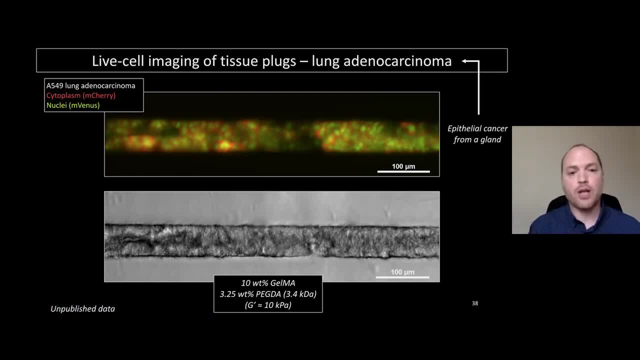 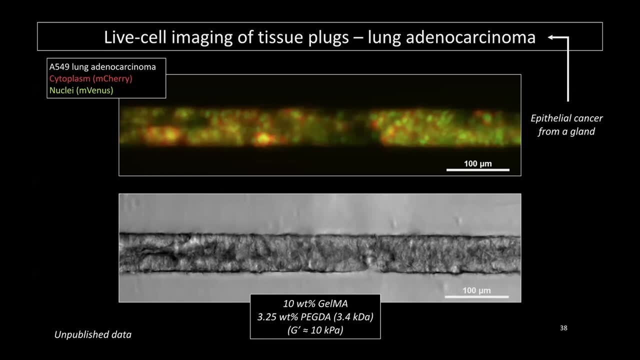 Wouldn't they all die? Well, they wouldn't all die If you have a second vascular network that is perfusing the nutrients through them. So here are some lung adenocarcinoma cells, double labeled for the cytoplasm and the nuclei. 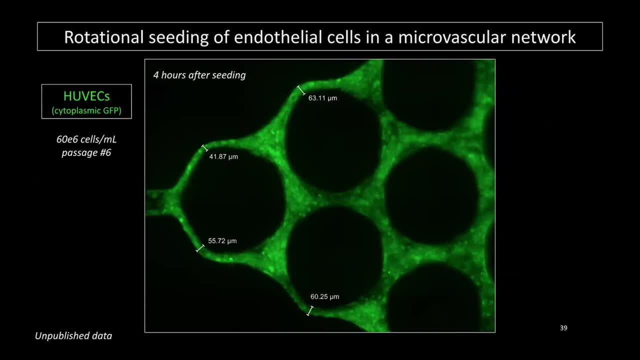 and just showing that the cells are doing OK there. So here now we're injecting cuvex. These are expressing constitutive GFP into these 50 micron vessel networks. Some of these images we're very happy with. Some of this process is very difficult. 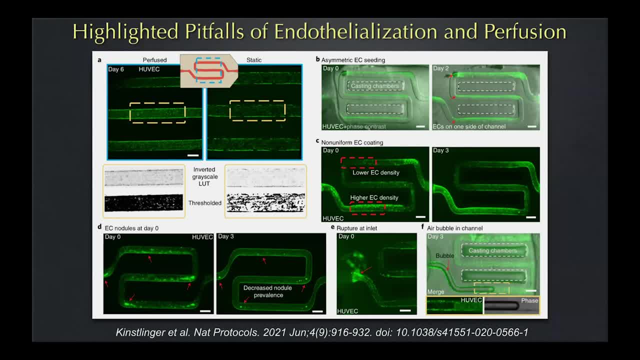 And in this paper we actually highlighted some of the pitfalls and dangers and complexities of endothelialization and perfusion. There's lots of ways to do this wrong, So we found in the gels: if you don't do perfusion, the cells tend to die. 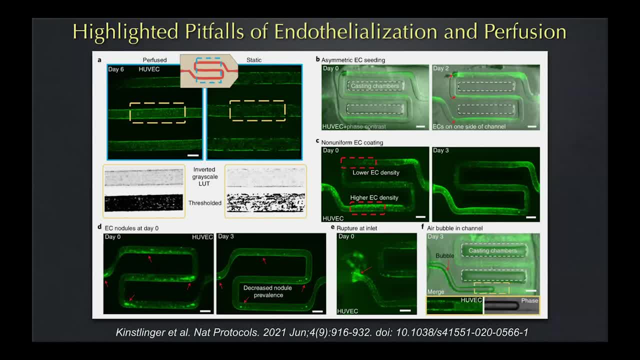 They need to have those nutrients coming in. If you over-seed, you'll get these endothelial nodules that seem to be some kind of bad physiology, maybe pathophysiology of the endos. That could be something interesting to study. We're trying to get really better endothelium. 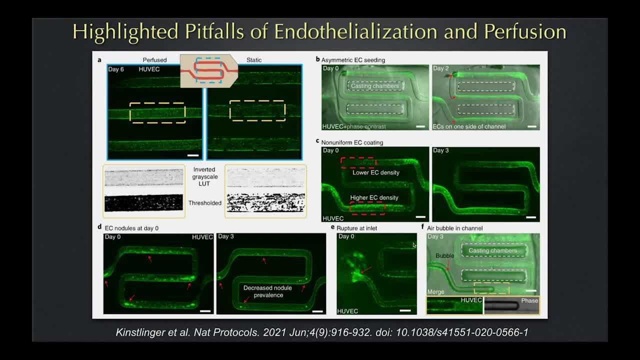 If you don't do the rotation correctly, you'll have other ways to get non-uniform seeding, And bubbles are always going to be something you're scared of when you're doing flow perfusion studies, So definitely want to have bubble traps, et cetera. 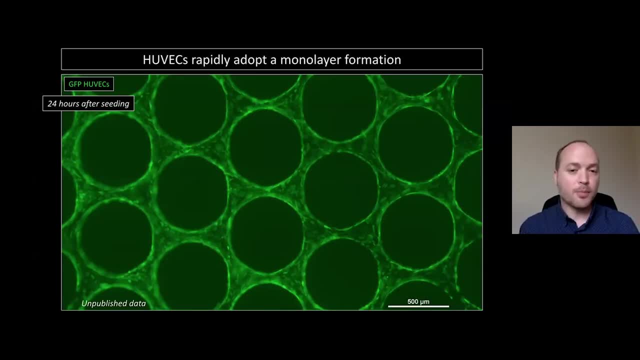 Once you solve all those problems, though, we've been able to get really – this is unpublished work, but we were able to get very exciting to us- vascular networks that are patterned, that have vessel components that are under 50 micron in diameter. 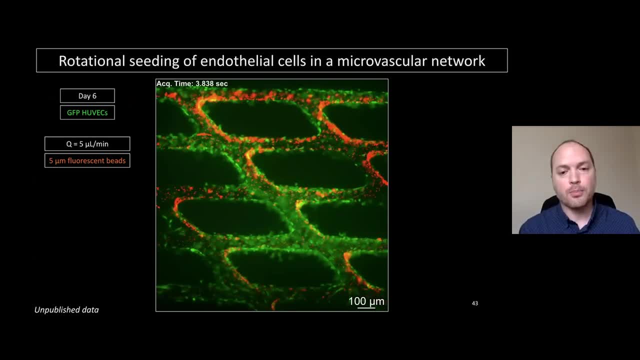 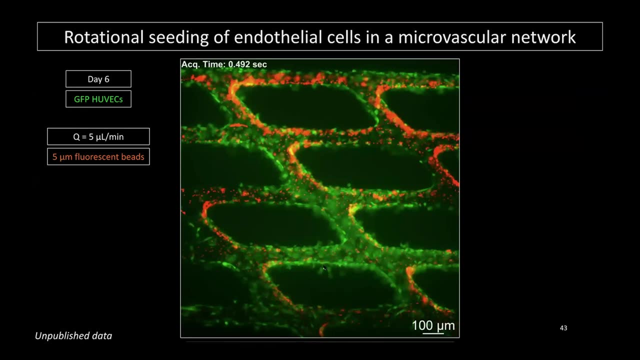 We're able to get flow through these. So here we can see five micron fluorescent beads flowing through what looks like, effectively a percolation network that's endothelialized. We even have some of the endothelial cells beginning to sprout androgenic sprouts into the vessel. 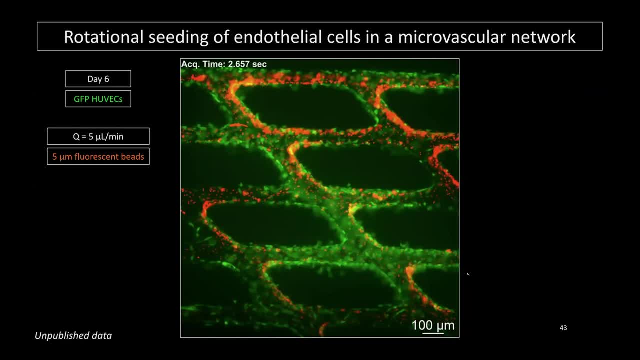 So we're still studying this in detail, But these are degradable gels. They're mostly based on gelatin, methacrylate, And it's sufficiently simple enough for the cells to grow and migrate through. They secrete their MMPs and go through. 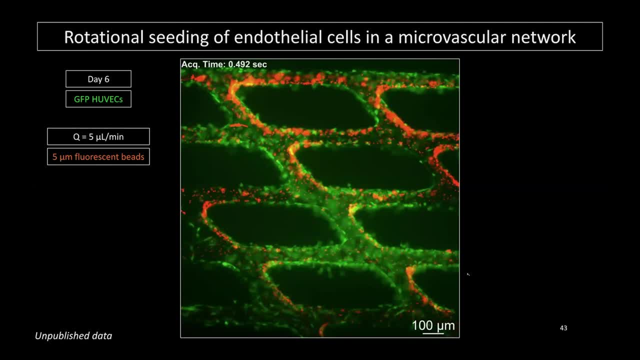 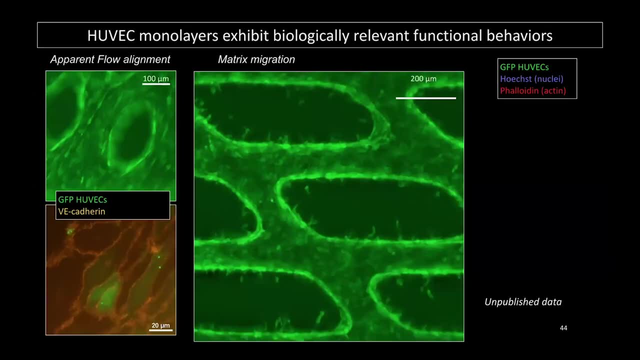 It's a lot simpler than some of the maybe random estrobond hydrolysis techniques that our field really came from And we're really looking at that endothelial physiology now. So we really needed new technologies to get the architecture. Now we have the architecture. 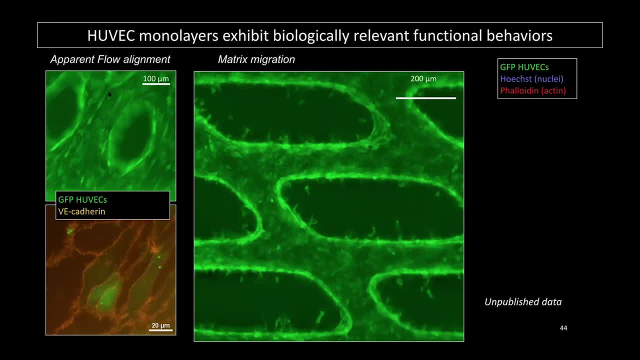 Looking back at biology, what can we get for the endothelial cells? How stable are we, Are they? Are we getting flow alignment? It seems it's possible. We're getting some evidence of that. We're looking at the VK adherence. 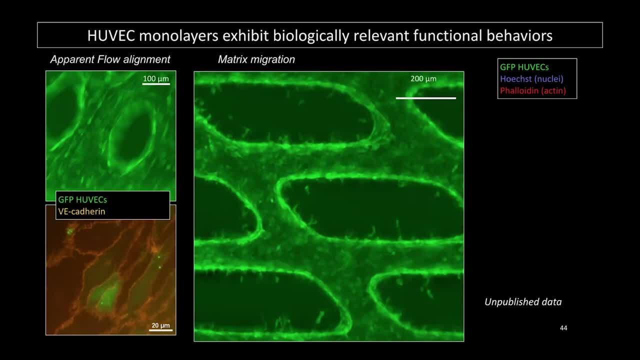 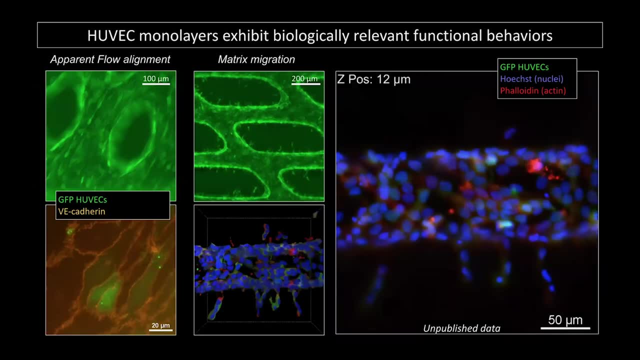 We're getting good cell-cell junctions And studying the permeability quantitatively of these vessels. we can do confocal microscopy and show what is the nature of some of these nascent – androgenic sprouts. How many cells are there? 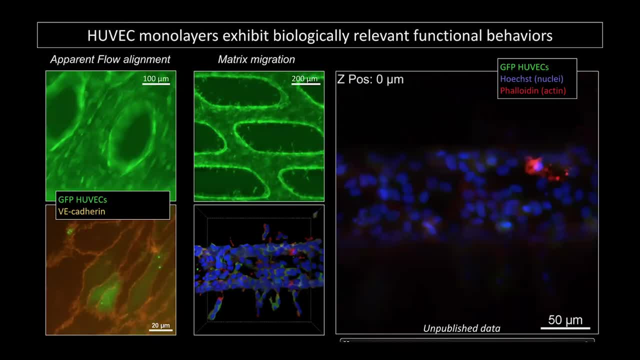 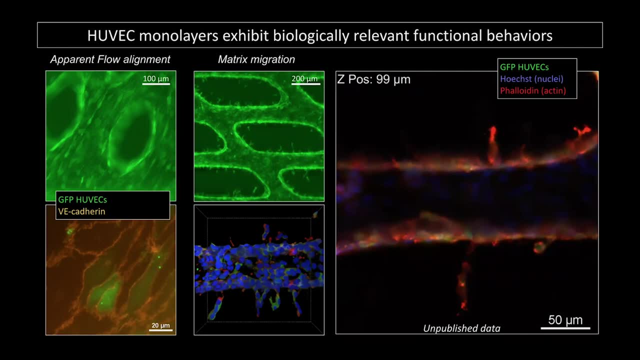 Are they connected? Where are their nuclei? Look at the phalloid. Very exciting to us. Now, what about this city block region that we want to put cells in? Well, this is even more recent. We have now – this work from Dan Sazer, who also just defended his PhD. 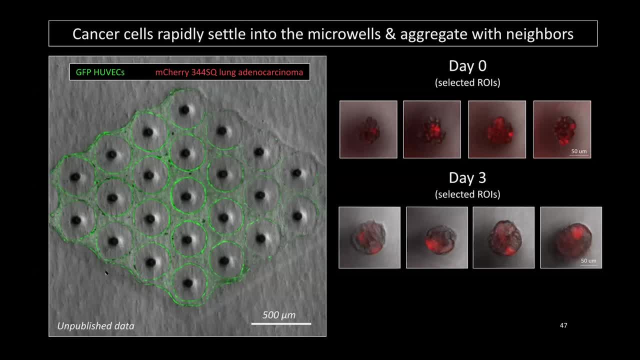 and also moved to Boston to do his postdoc – or sorry, he's working in industry now, but over in Boston. So now we have individual microwells that are at very – at very specific distances from our vascular endothelial networks. 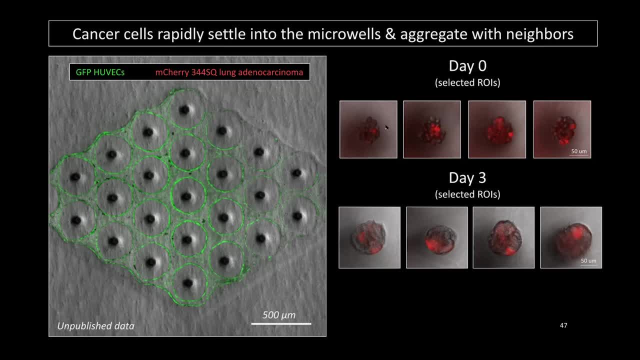 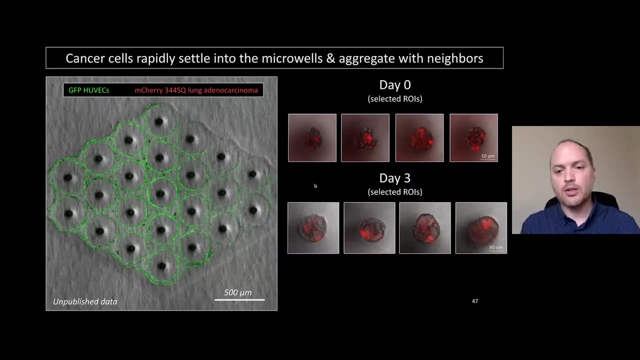 You can see, here we're looking at lung adenocarcinoma cells. just a very good positive control for us It just – are the cells alive or not? Are they able to capture nutrients? And so you can see, from day zero to day three, the cells and their aggregates begin to grow. 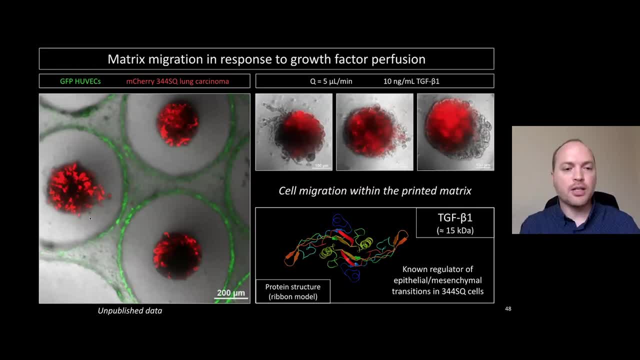 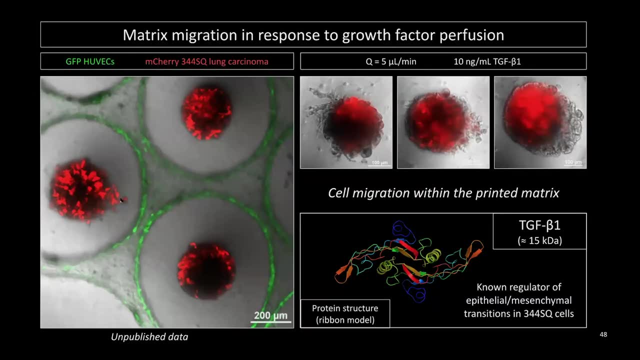 Further what we have – we're actually now seeing the cancer cells beginning to migrate out of their microwells, perhaps towards the vasculature. So we're seeing. how close can we make this distance? I don't think we can get down to sub-one micron distance yet. 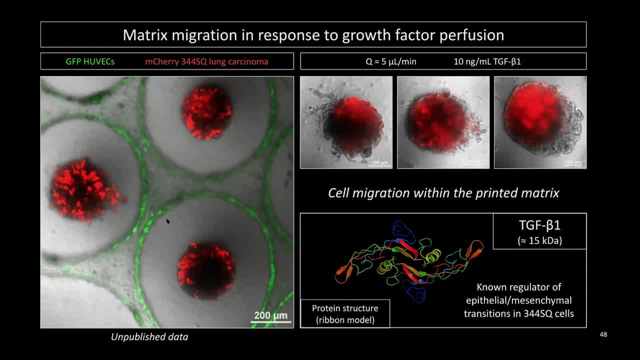 That's something that we may not be able to do by 3D printing anytime soon, but it may be moot, if this is reproducible enough, that we can study things like the androgenic switch or things like delivering specific factors to stem cell aggregates in these different areas. 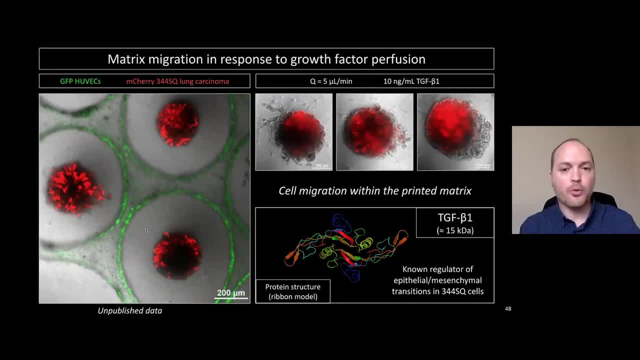 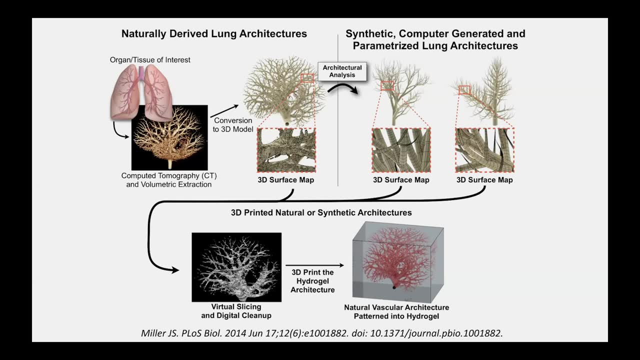 So this is brand-new work we're very excited about, very excited for potential collaborations with any of you, So I'd be glad to follow up Just overall. in general, what we're trying to do is think about what is the total organ structure. 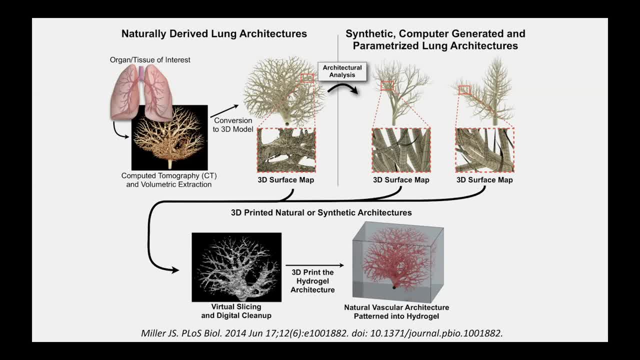 We definitely can't make that yet, but we're very excited for a pathway of a Moore's law-like scaling that we need to do, that our field is in process of doing, to get hundreds of millions of these vascular unit cells inside of a packed volume. 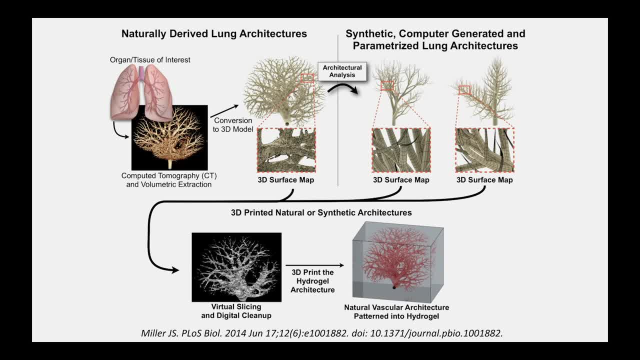 in a way that they're all connected and plumbed just like it is inside the organs. And we can do that by looking at organ structure, breaking it down on the anatomy side. But there's a lot of mappings of organ structure in the literature from decades ago. 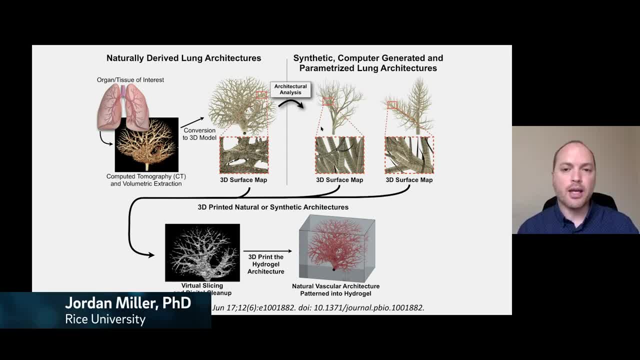 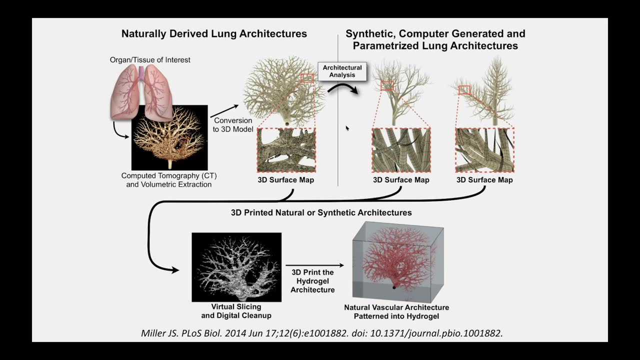 and some of the newer ideas are: we could build a de novo vascular network that uses characteristics of the in vivo environment and the in vivo network topology. regrow a synthetic topology would be cleaner to grow and modulate in terms of structure. put that into the gel and then study function. 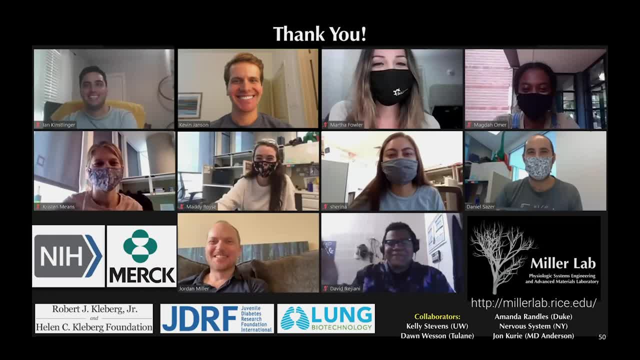 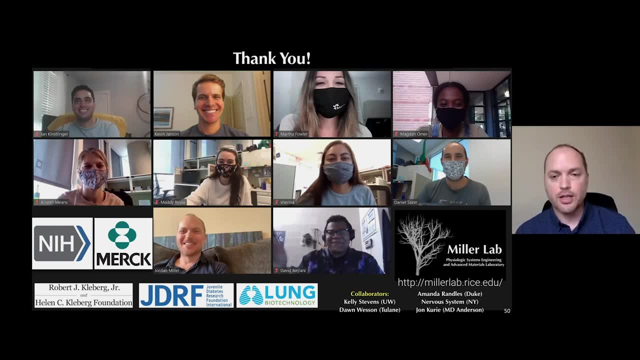 So with that I'd like to thank the members of the lab. so Gregor Gorian led up a lot of the early work in the science paper, Ian Kinzlinger and others on the endothelialization of the gels and looking at these growth and proliferation gradients. 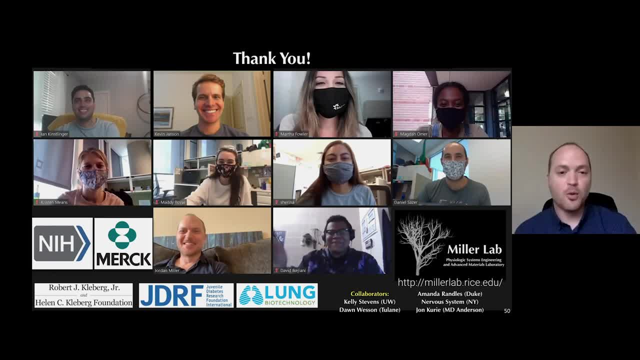 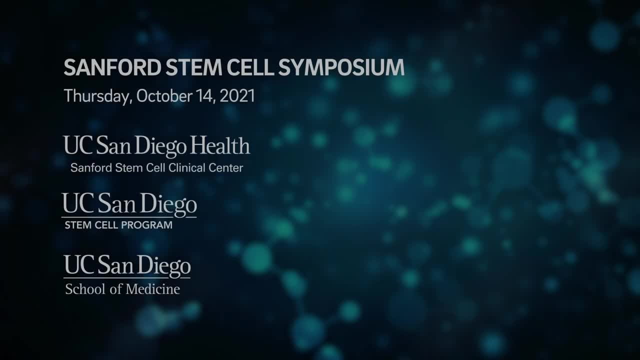 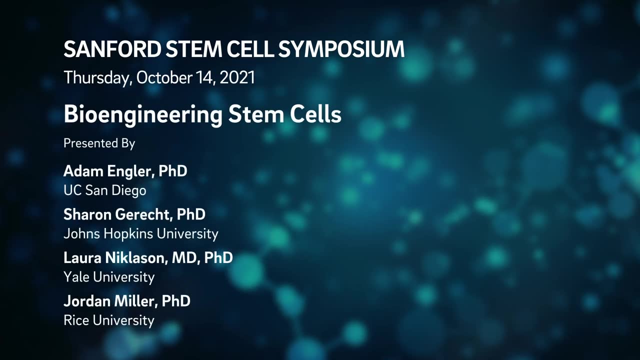 and Matt and Kristin doing a lot of the recent work on endothelialization of the smaller vessels, together with Dan Sazer. So thanks, Thank you.